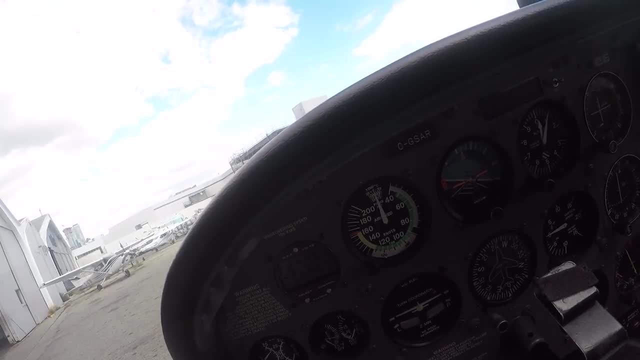 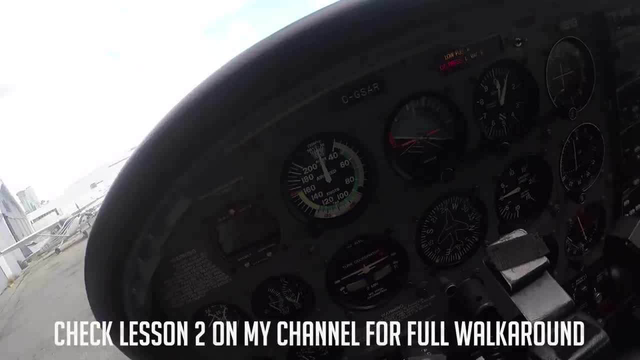 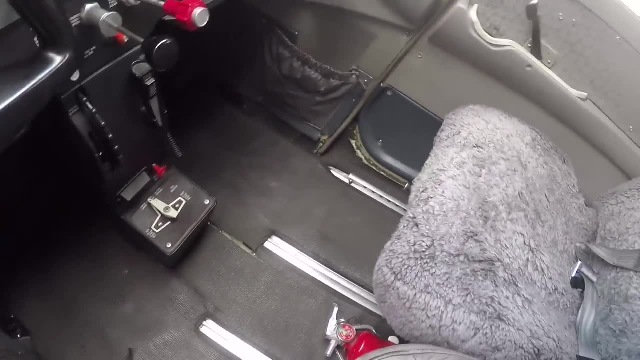 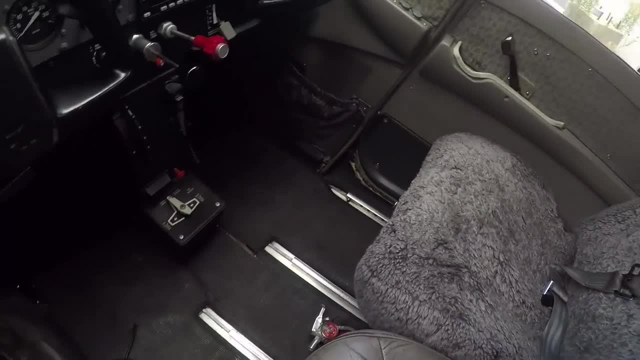 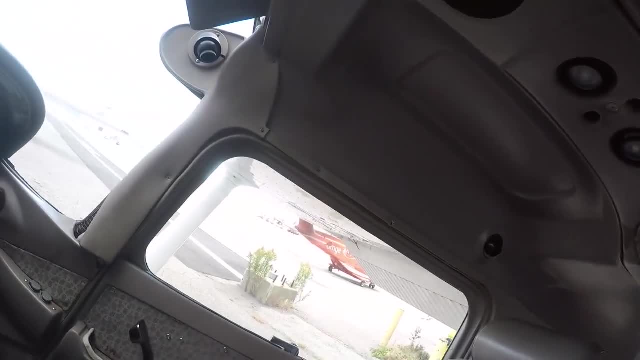 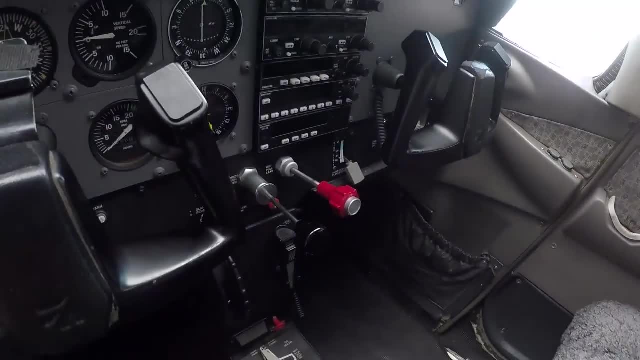 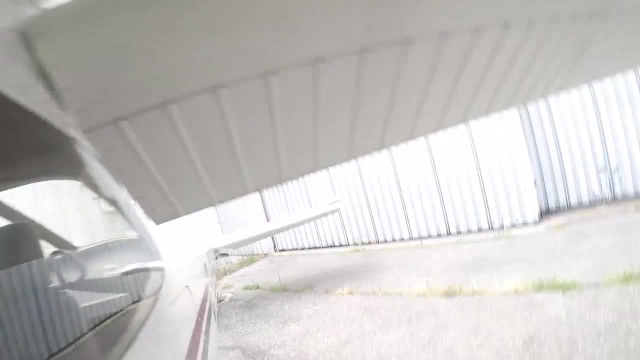 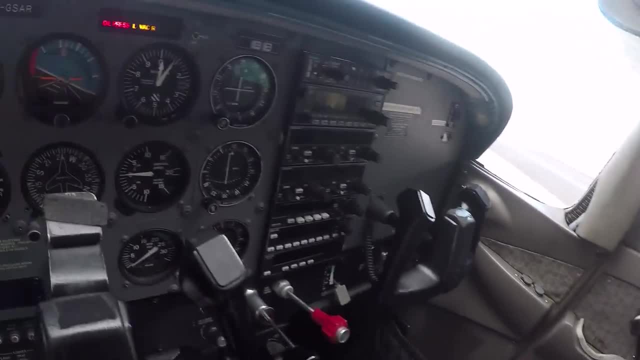 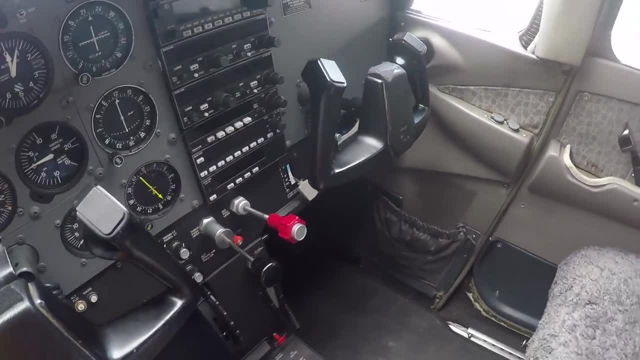 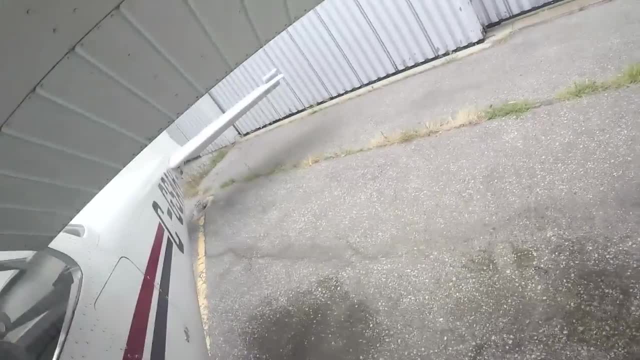 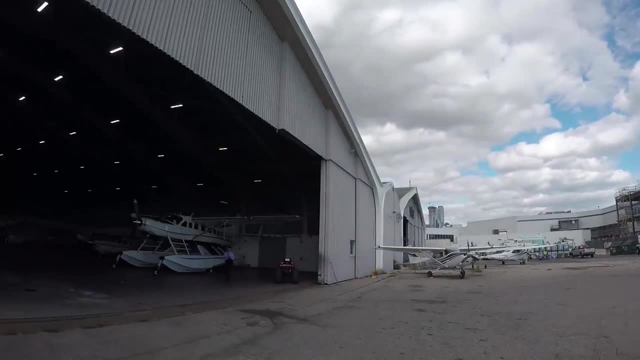 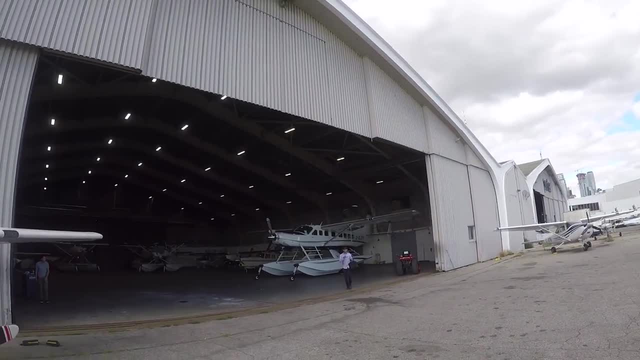 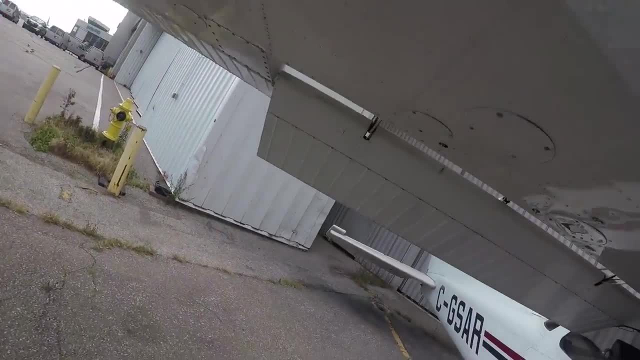 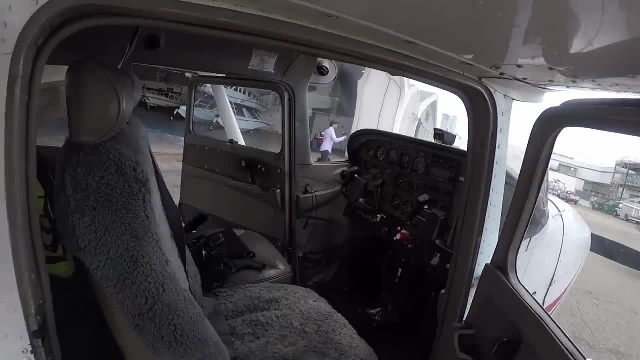 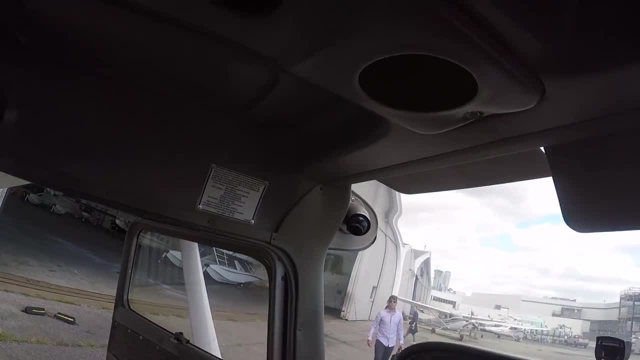 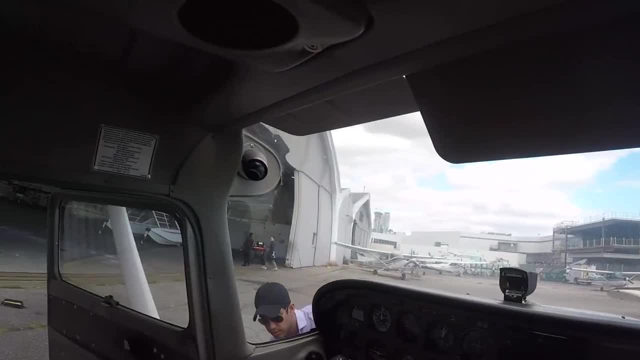 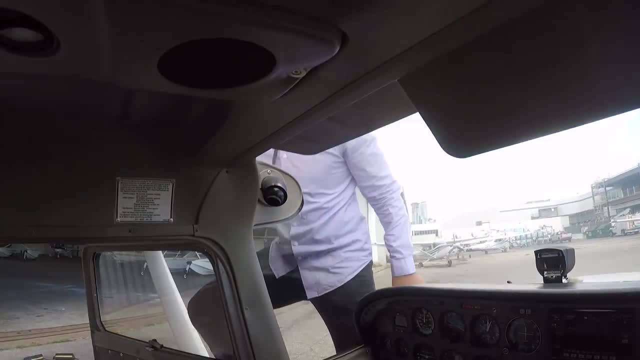 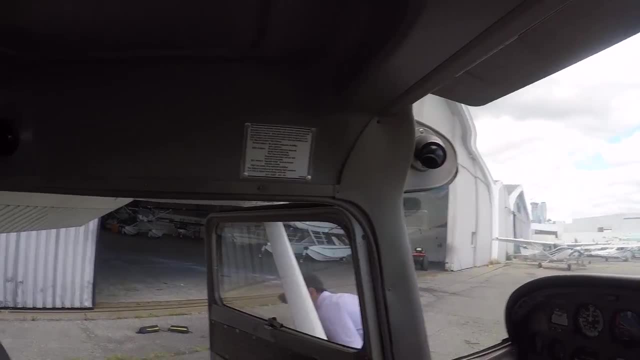 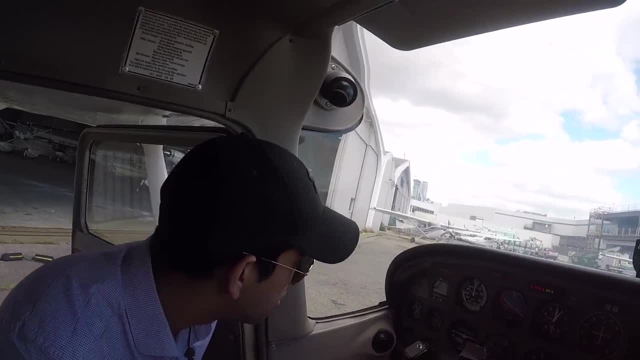 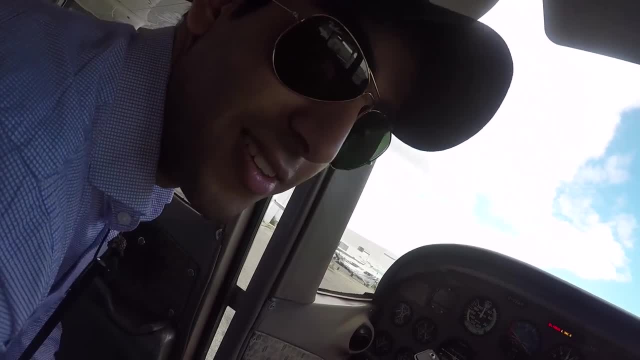 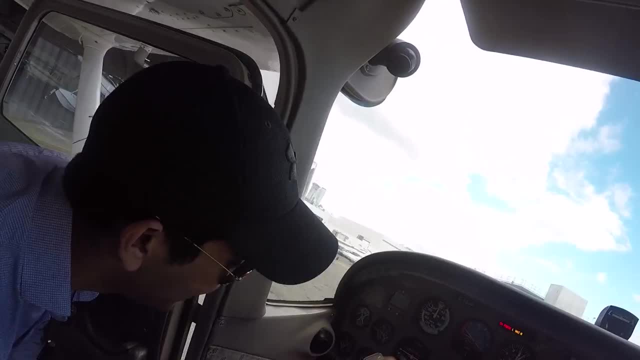 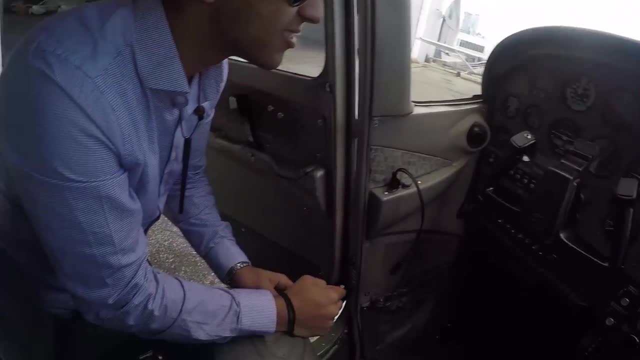 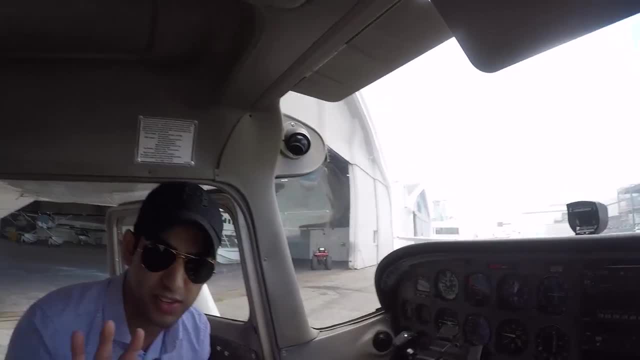 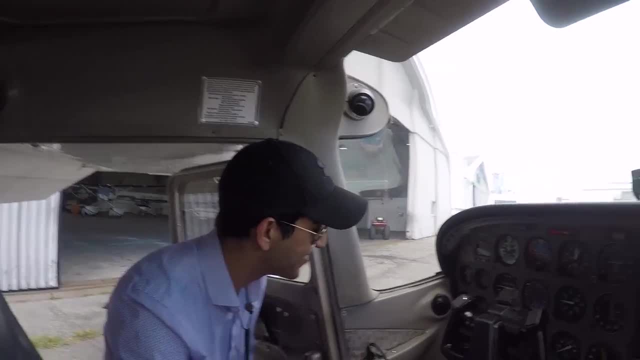 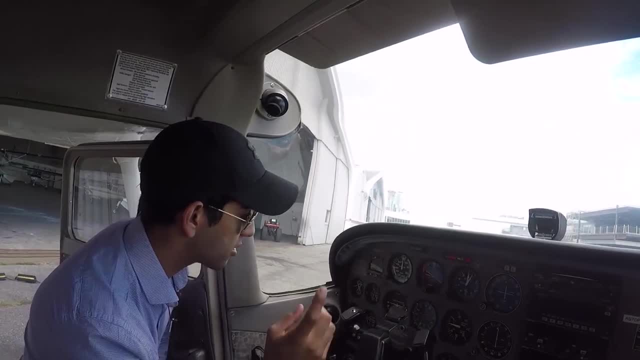 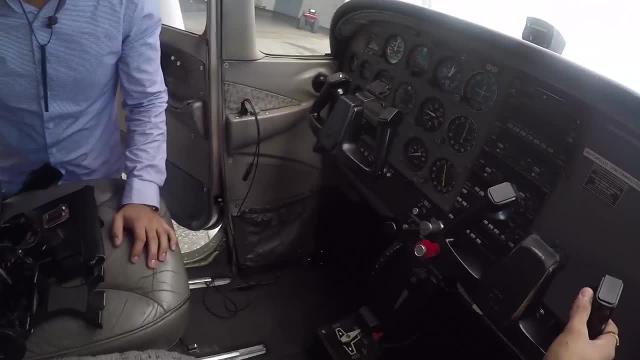 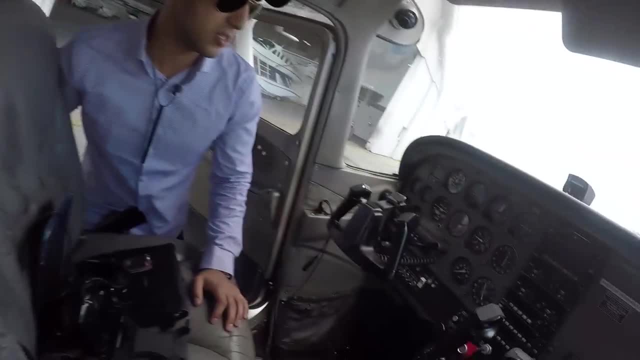 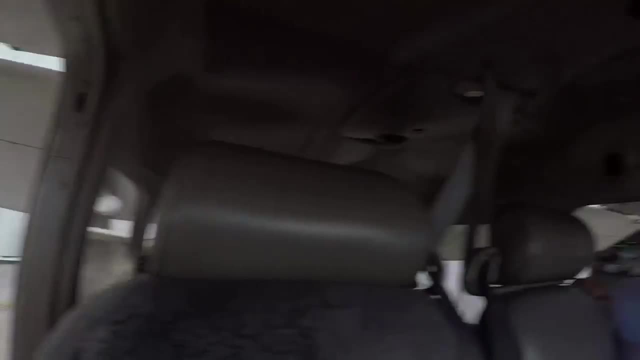 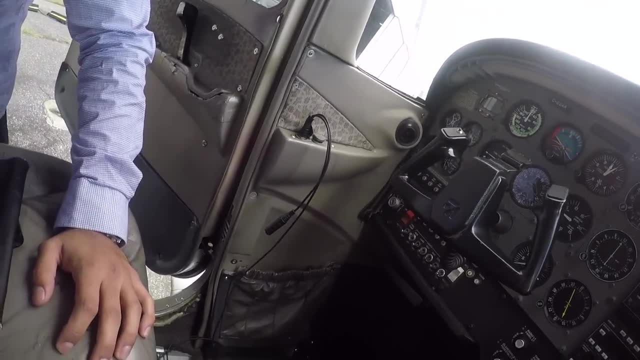 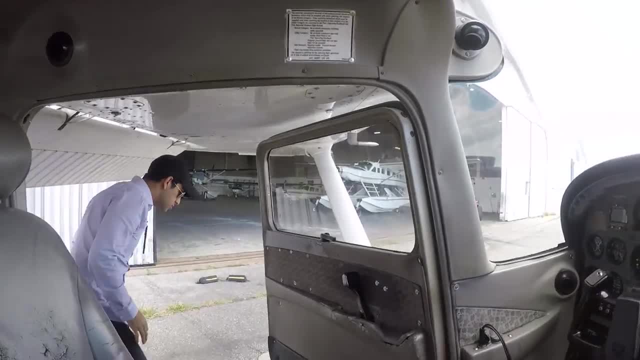 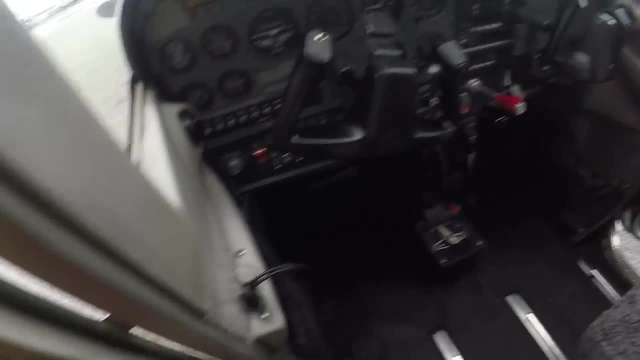 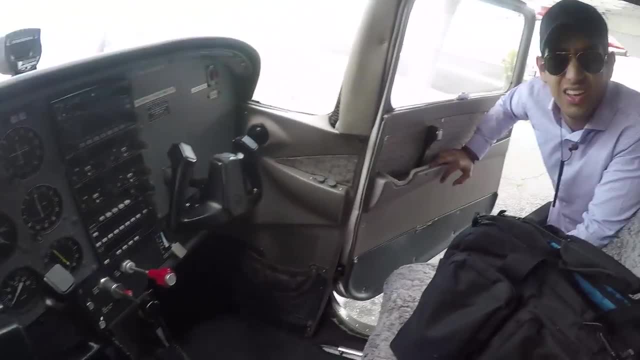 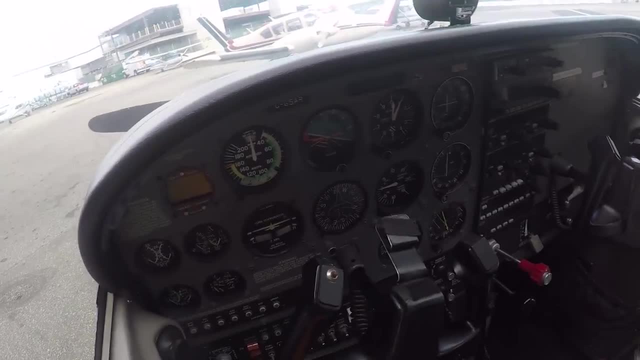 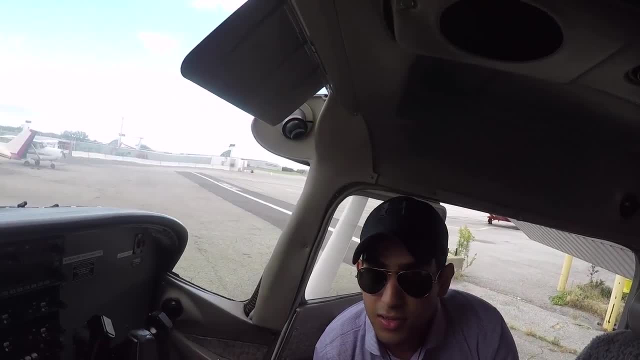 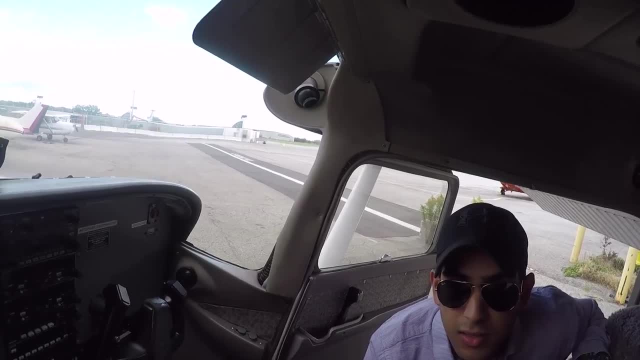 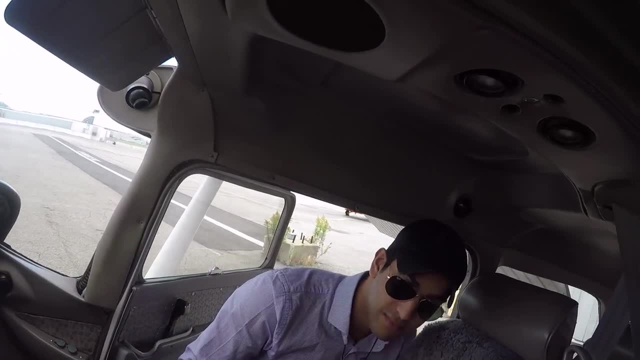 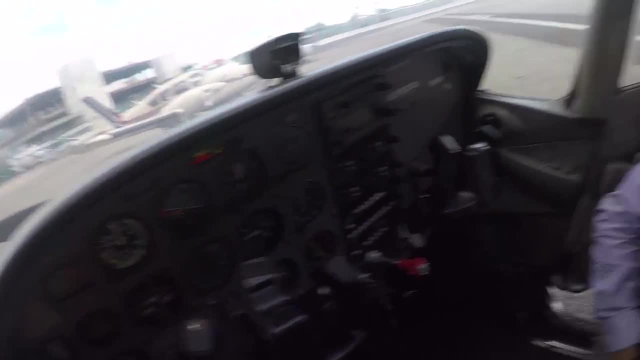 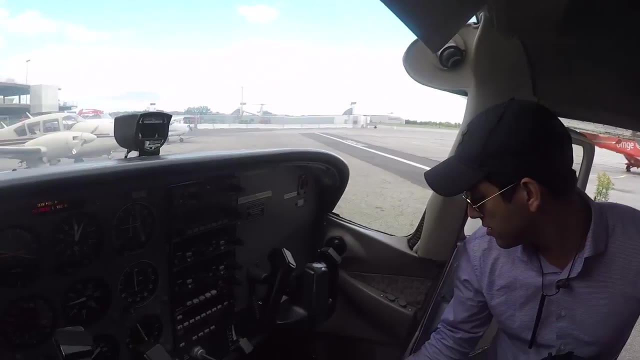 Welcome to the Wolfpack. and this is the Bad Wolf. how much fuel do you have in the right tank? it says zero. here again, you know how much is in the right tank, right, the gauges aren't reliable, right, okay? so, oh yeah, we have to see. never rely on the. 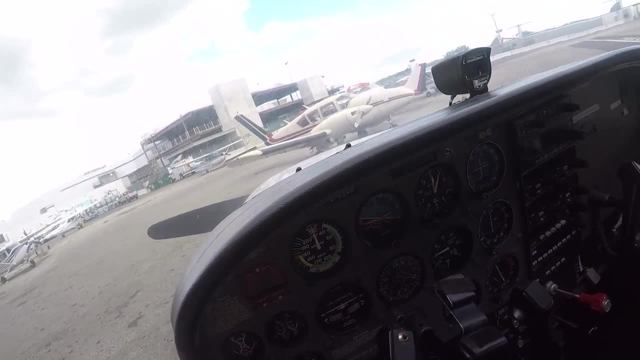 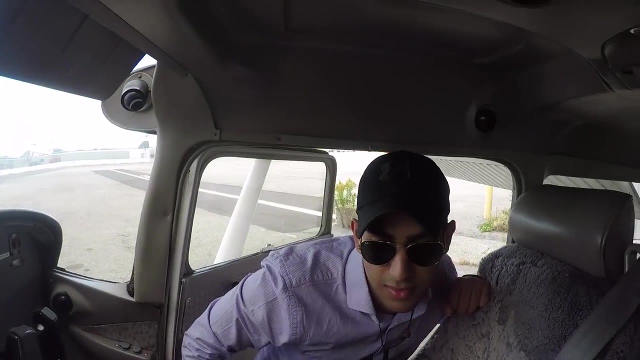 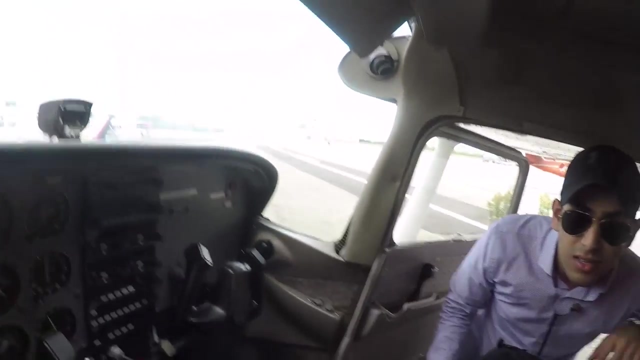 gauges when you're checking your fuel. okay, and the oil is, uh, between 6.5 and 7.. what's the minimum 6.5? how do you know? uh, pr, this is checklist. okay, perfect, so double check the tanks. yep, do you strain the whatever? 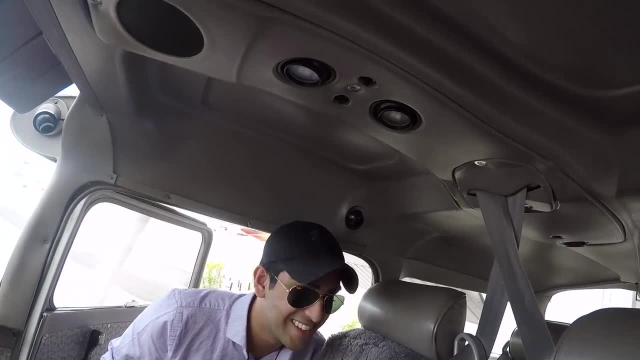 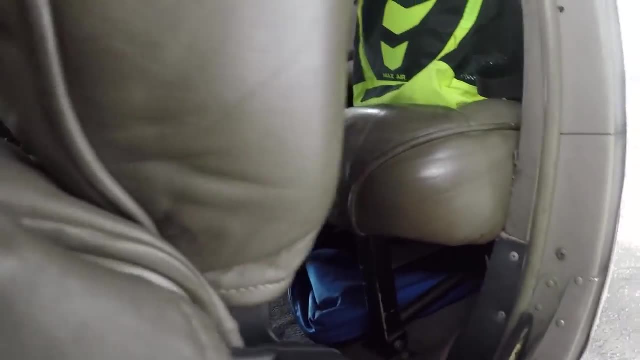 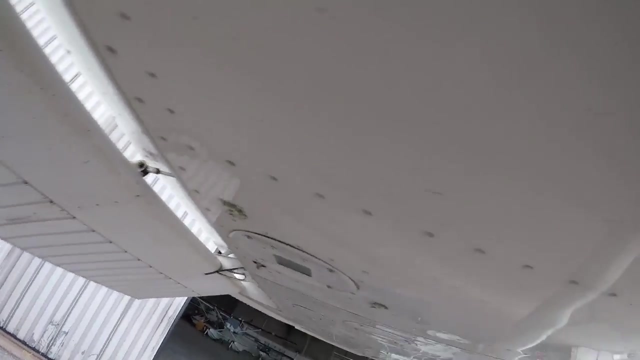 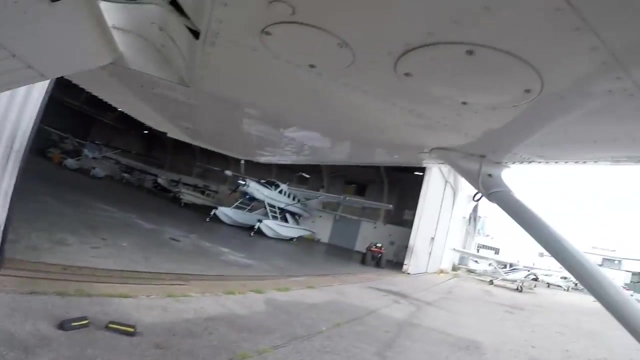 you mean that uh bottle thing? yeah, how to do that? i don't know where's the bottle behind your seat, behind your seat, behind my seat, oh, in here, okay, yeah, so there are 13. i think that's a lot. of this is the one thing that makes me not want to fly these new planes. 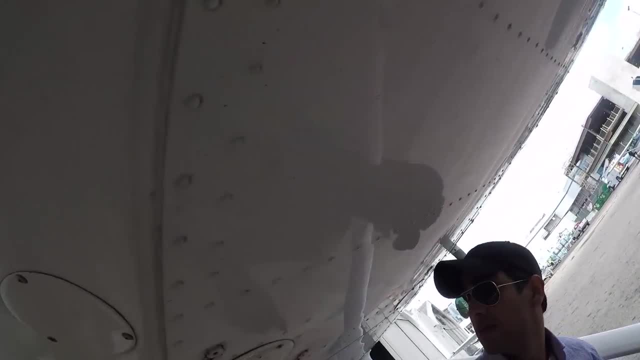 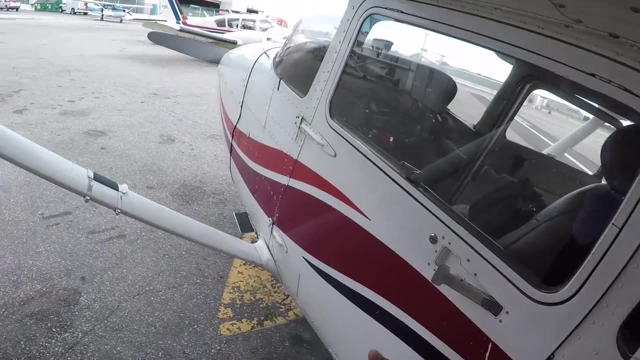 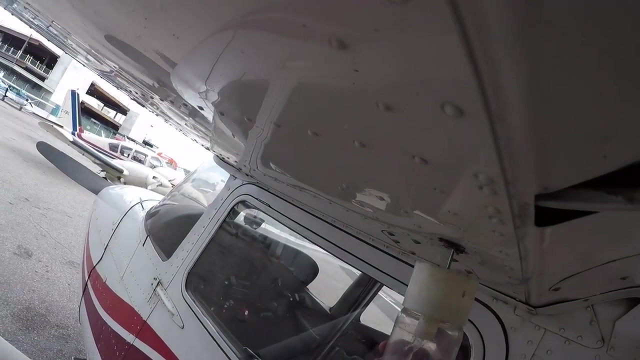 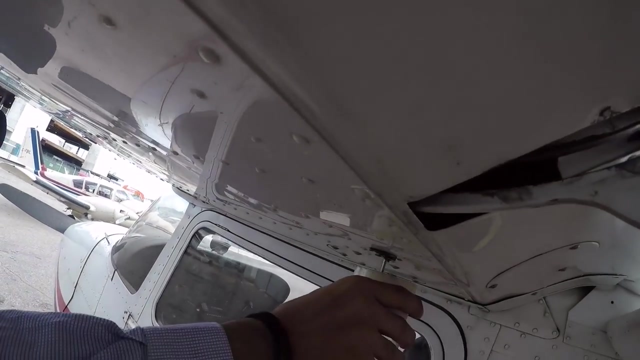 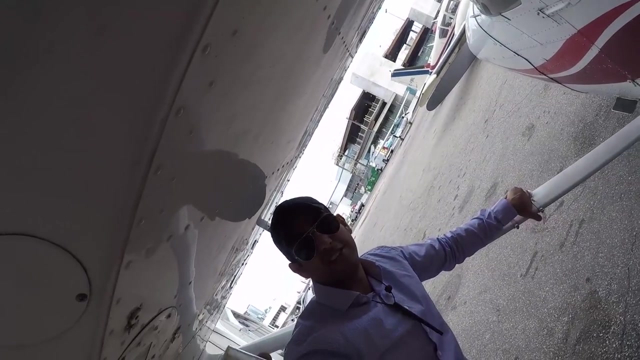 um. one, two, three, four, five. so strain them off. yeah, just stick it all the way in there. how excited. get more um, because we're gonna pour it all back into the tank, right, okay, fair amount. double check. let's add contaminants in there. it's just there. okay, it's from, it's from before. they're all so. 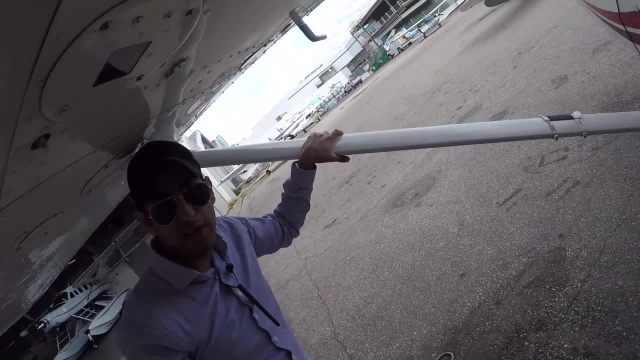 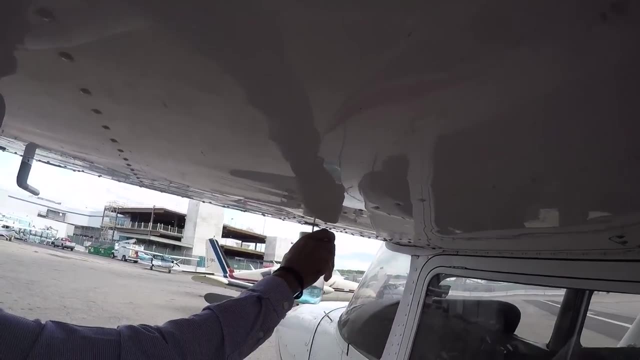 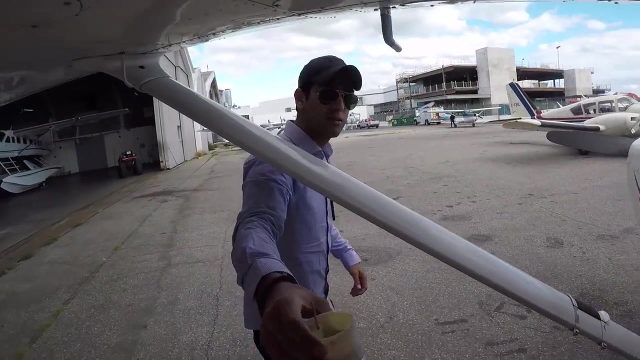 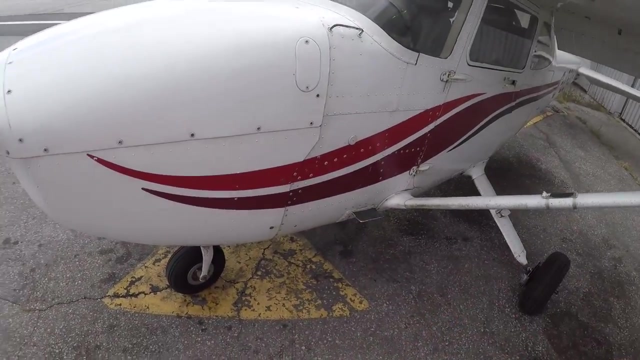 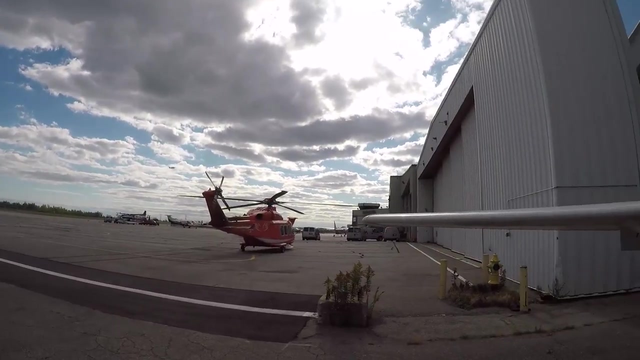 does it matter? no, we've got a filter net, so we'll just: ah, yeah, so i'll do this wing and then you can do the next wing in the under. okay, underside, okay, that's like a fair amount, right? mm-hmm, nice, nice. runway 26 is in control, so we're not getting the scenic approach today. 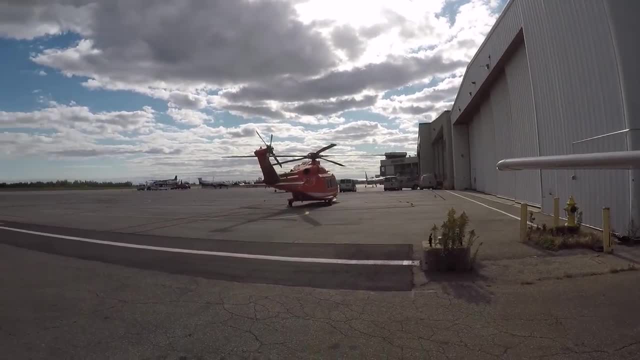 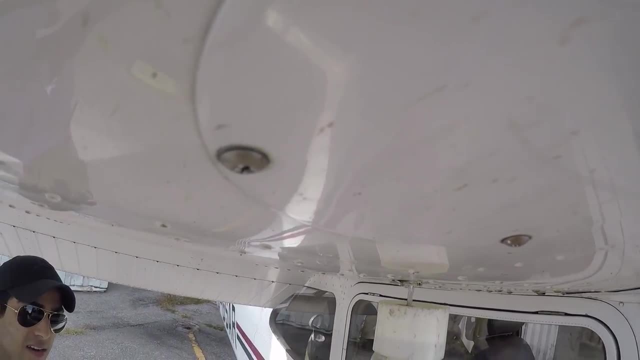 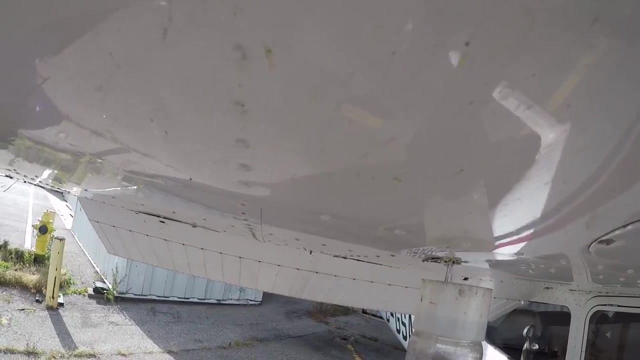 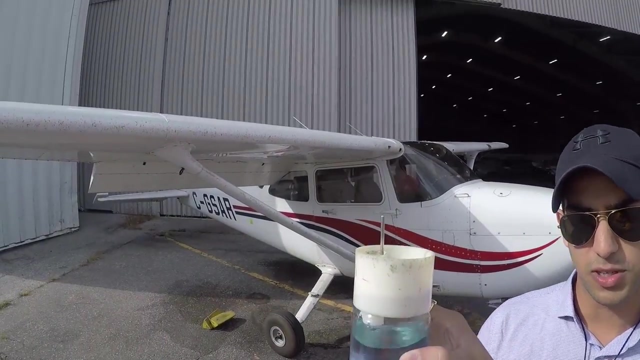 oh man, look at the weather. so there's five here as well. okay, all the way, yeah, Okay, Okay. so looking at the fuel, what color is it supposed to be? Blueish? Yeah, There's nothing floating around. If you saw water over here, where would it be? 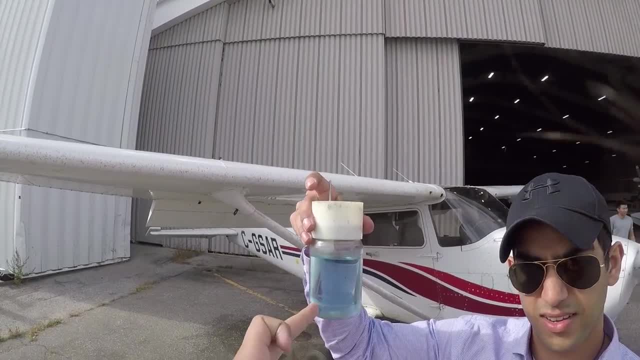 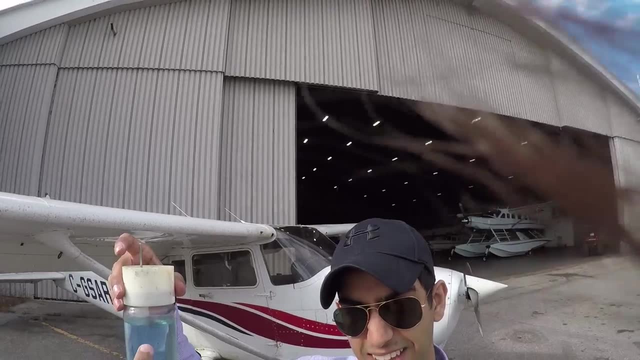 Water. Yeah, Is it more dense or less dense? Water might be down there, I think so, Are you sure? Oh sorry, Water will be floating up there. Yes, You're an engineer. yeah, I don't know what's the density of this too. 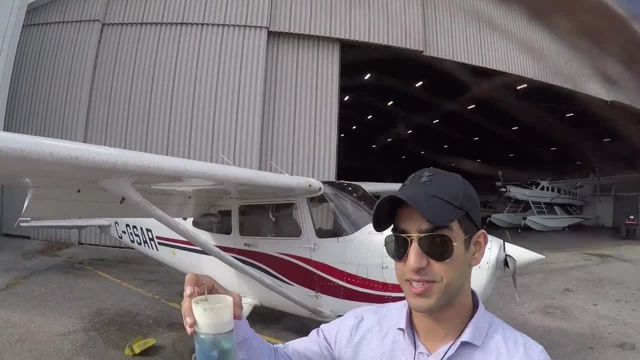 A little bit at the bottom. Okay, So it's more dense. That's what it is, Sir. No, water will be down here, Okay. So if you see water you want to, you know you drain it all out of the tank. but what? 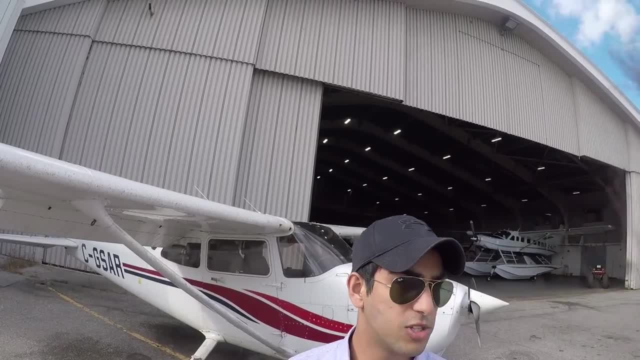 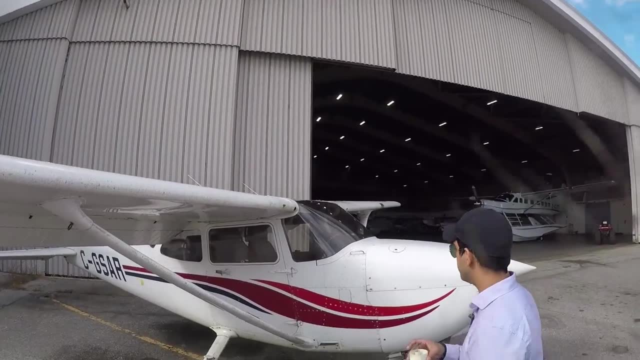 you want to actually do to something that's not just water in the tank is they are probably better. Okay, Yeah, Fixing it up here. There's three more underneath here, So one is right here. Okay, Okay, Okay Okay. 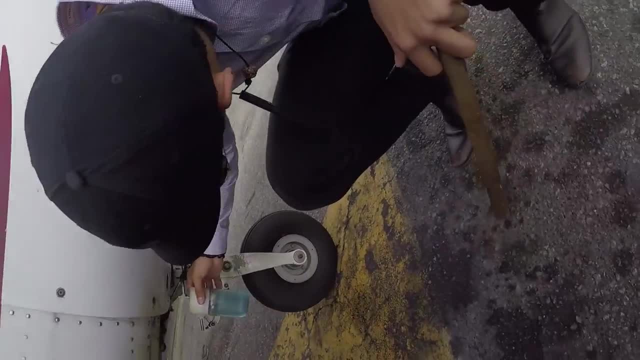 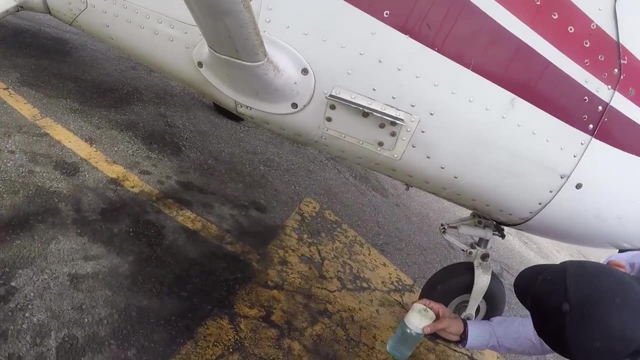 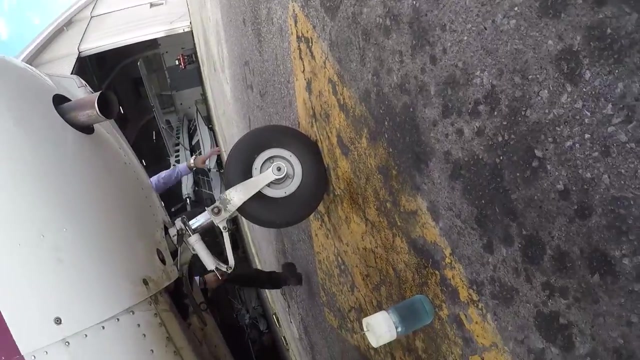 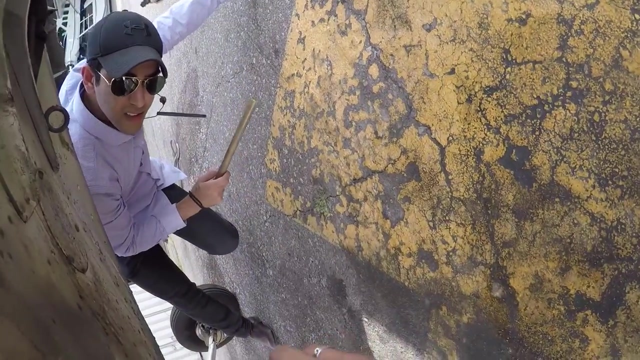 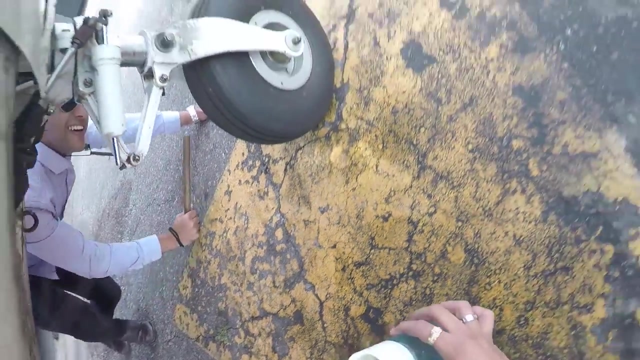 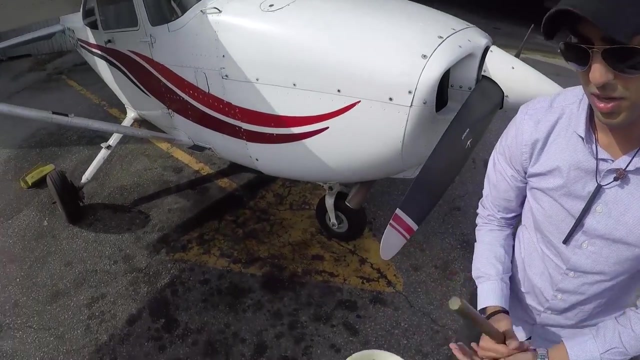 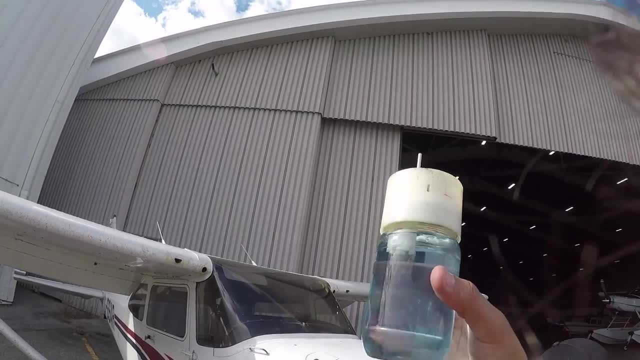 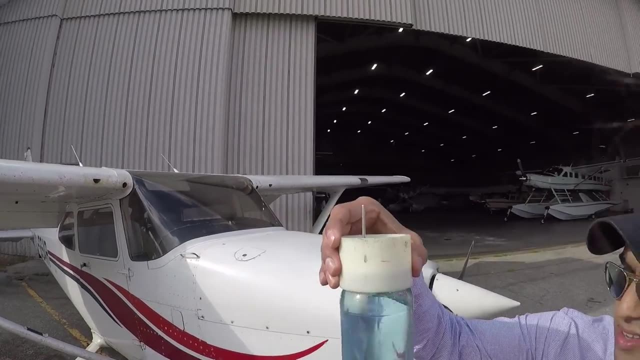 There's no water in there, because we'll sit down if there's any, If there's any floating around, there is something, but Is the cups just dirty? Yeah, okay, Okay, so you pour it back in the tank, Yeah. 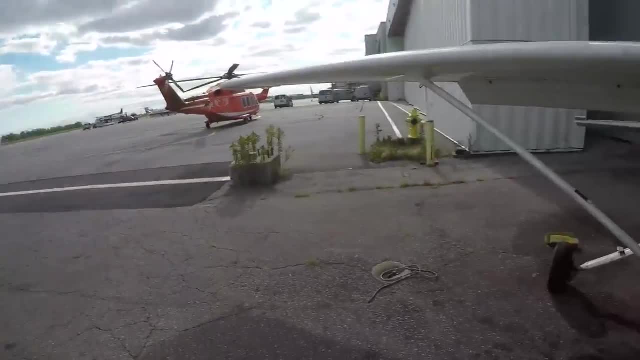 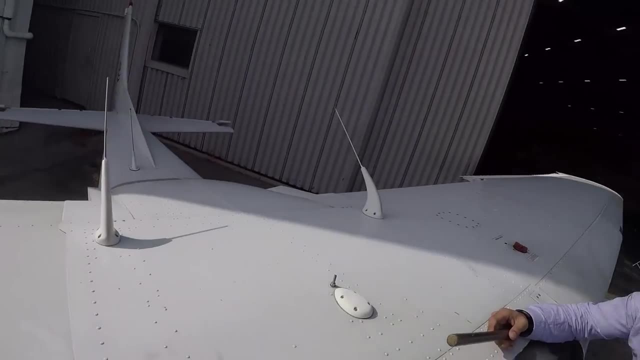 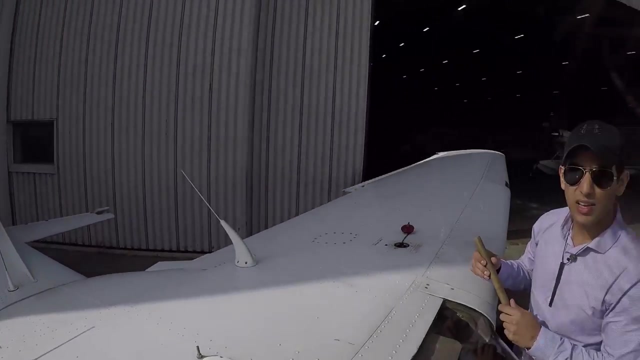 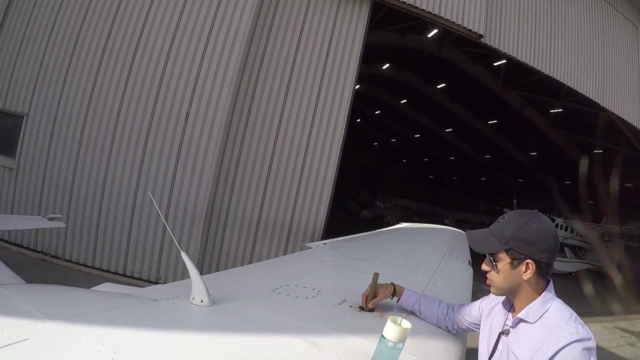 You can't go up on the other side. No, Wow, it's cool. So yours is full, right? Yep, If you didn't know whether or not it's full, you take the dipstick and put it in. There's a line here, but you can stick your finger there to make sure where the top of the tank is. 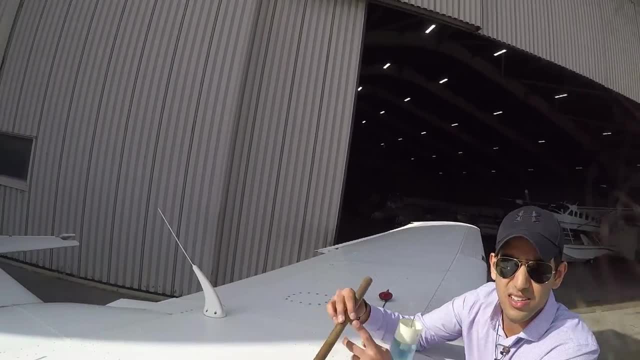 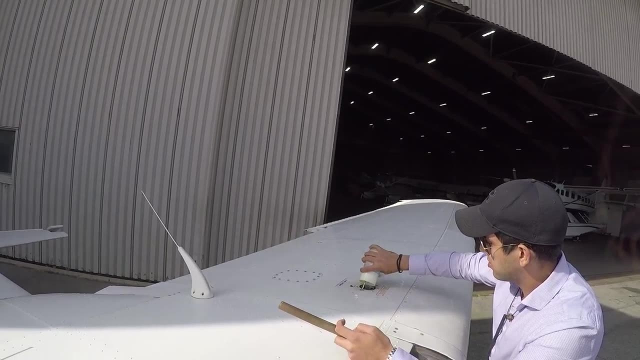 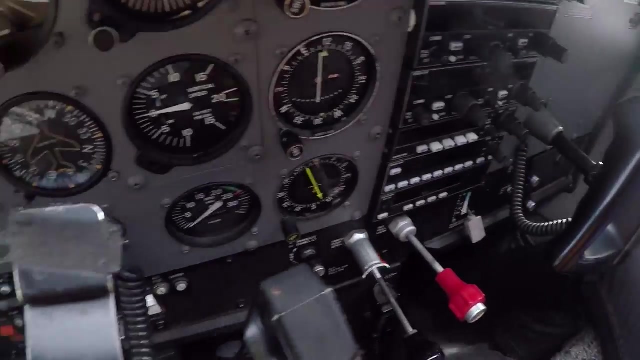 And see where the fuel is. so you've got about 80% of the tank, Okay, And the gates that we observe are open. Okay, 30 seconds. brake caps in check. Fuel shut off. now in check. Fuel left tank. 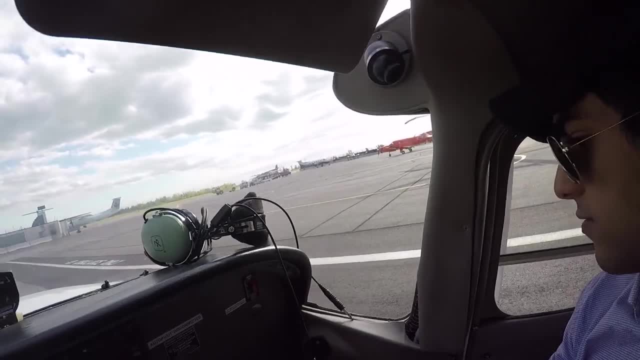 Check Brake car halt. It's 7.2,. was it 37.2?? 37.2, yeah, 37.2,. okay, If there is an explosion, We can switch on. Okay, cool engine start. 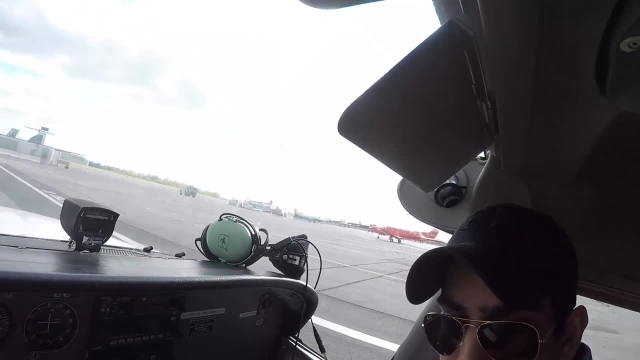 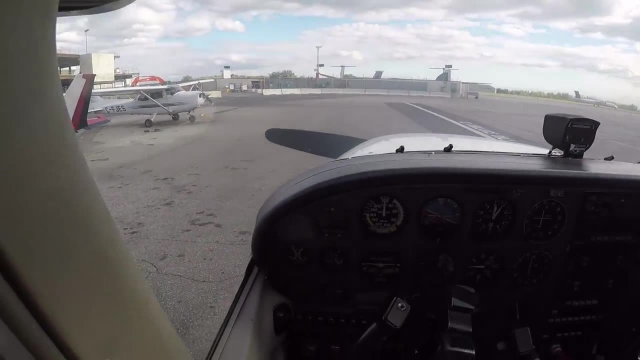 Make sure it's rich. How do you know it's a cold engine. It's cool. I saw that. Did you put your hand inside? No, the warm right here. the best way to do it is turn on your master. okay, see the temperature. 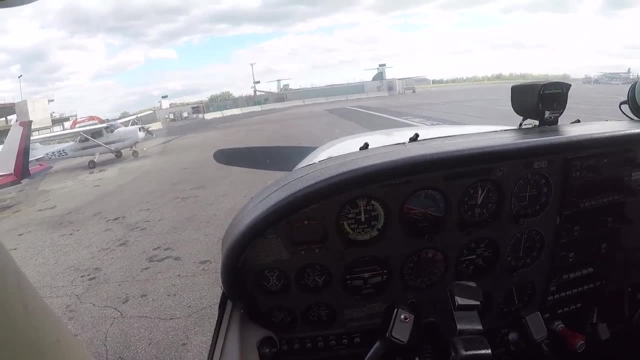 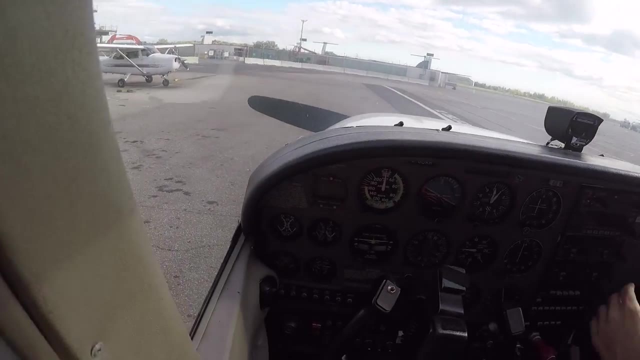 it looks like hasn't flown at all today. okay, so it's a cold engine. so if that's, from what? could it be? what if it has been flying? so, um, if it's gone flying, it'll probably be still in the green. okay, okay, all right, that's you. i mean, there's no exact guideline. 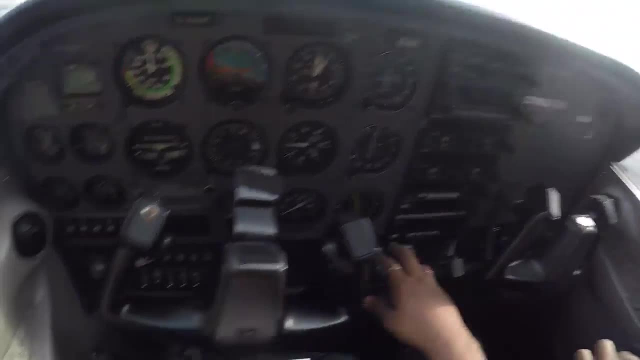 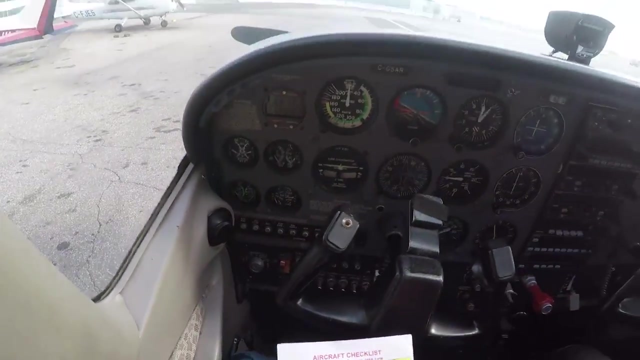 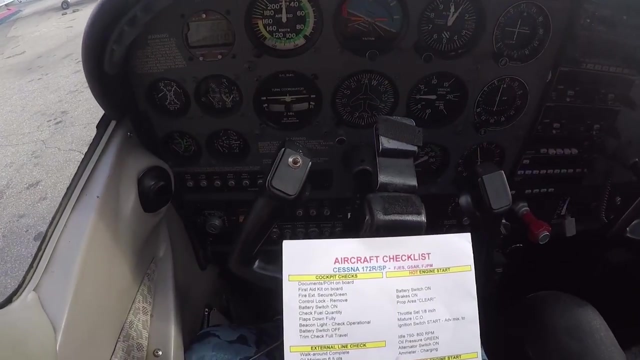 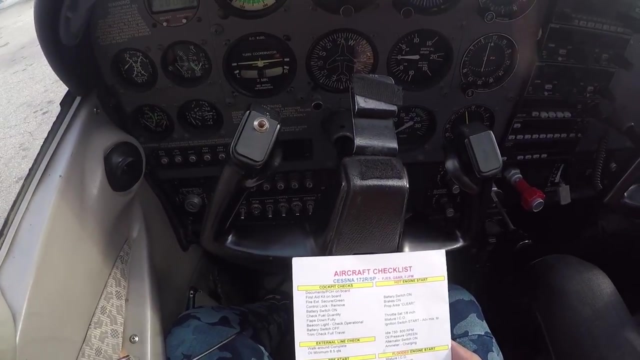 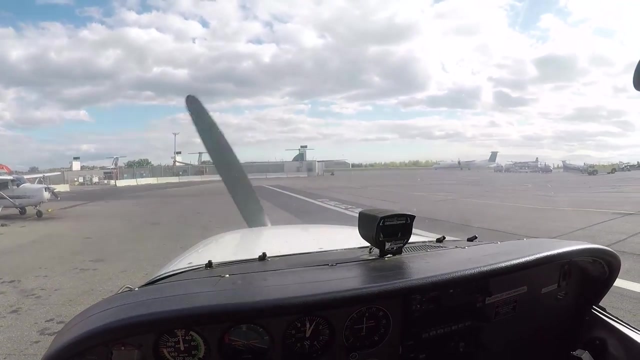 that's just generally what i use. um, okay, you might end up, you know, over priming the engine if you don't start them. that's just fine. proper, clear, clear 15.43 for a second? okay, okay, make sure i will cut off the ignition switch down. 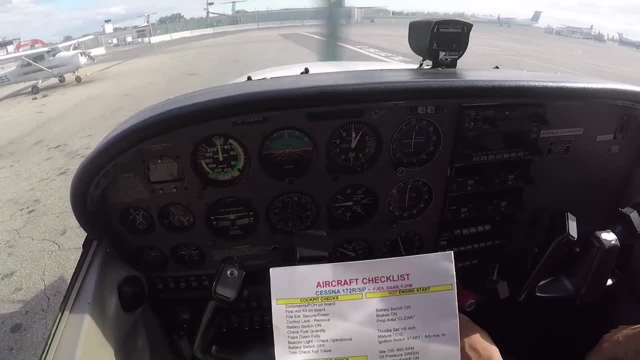 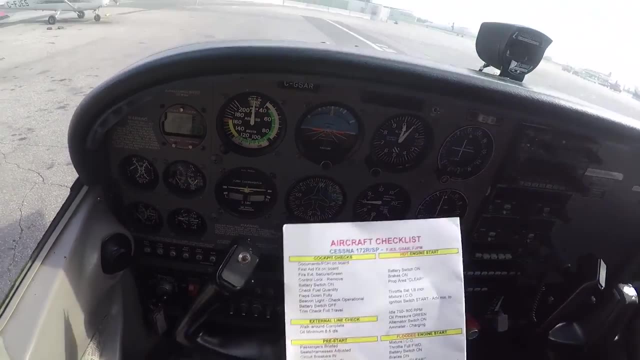 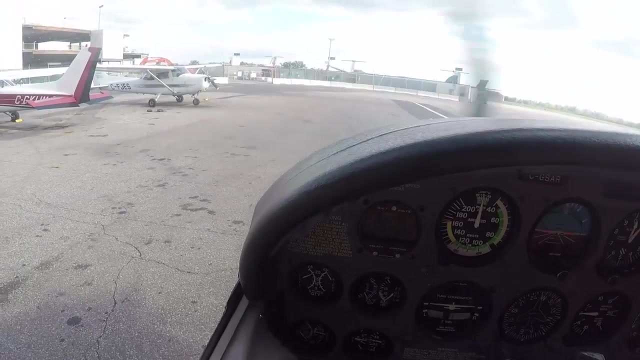 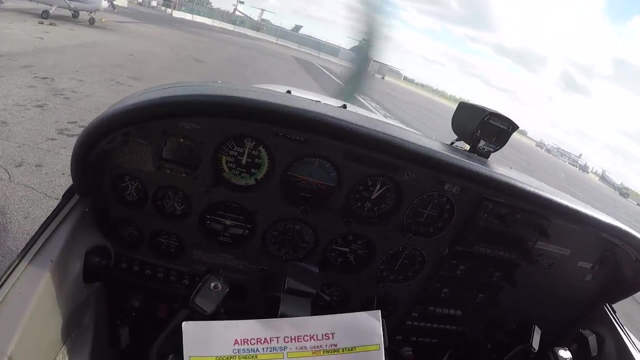 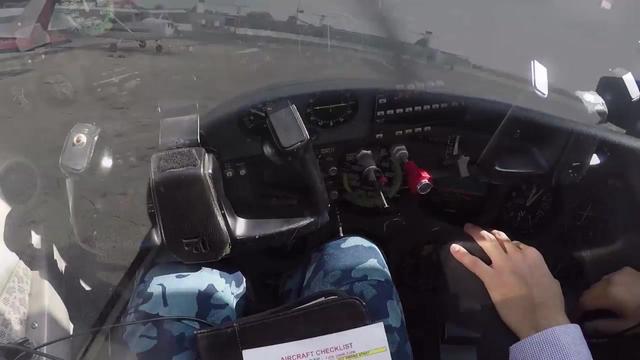 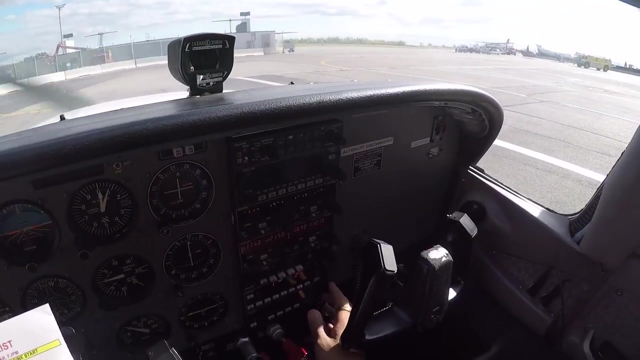 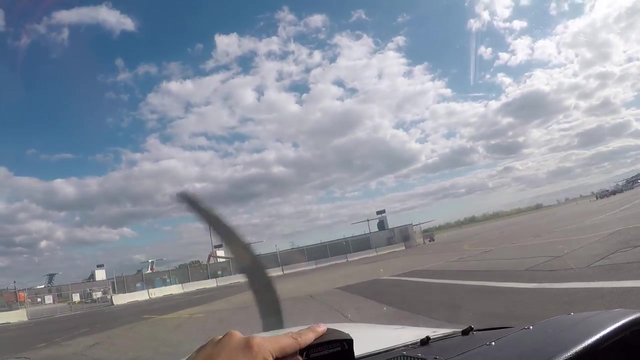 so okay. so other pressure: now we can set it green check. all right, switch on. and we're starting, please, okay, all right, okay, avionics master on check: flight as required. transponder standby check. it's on standby, okay, 1200. okay, heading indicator is at 15: 40.5. 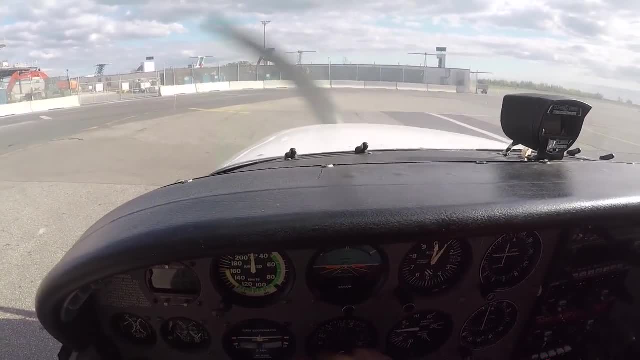 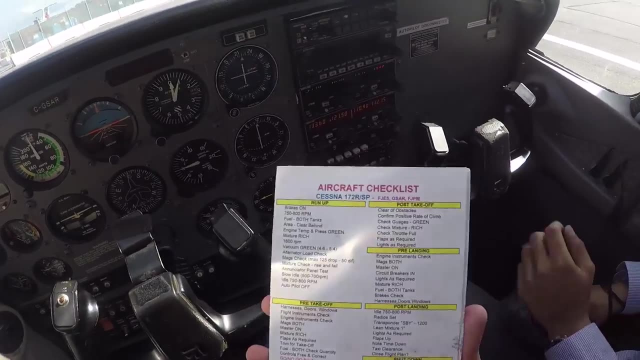 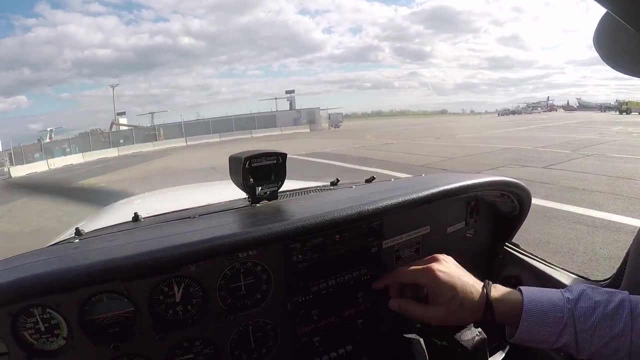 why is it so difficult, i don't know. some of them move a lot, some of them barely move at all. laps is required, so it's there, okay. this is cop two. this is cop one. you can just press cop 2.. you have information, juliet. 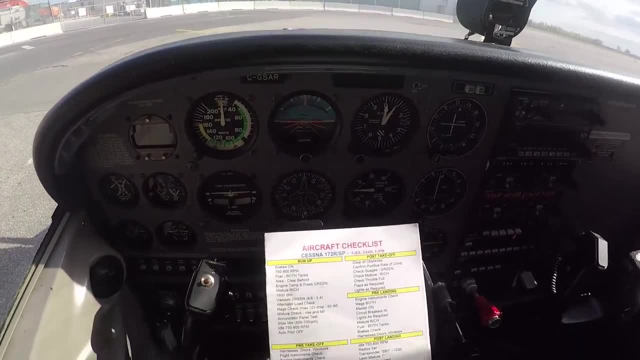 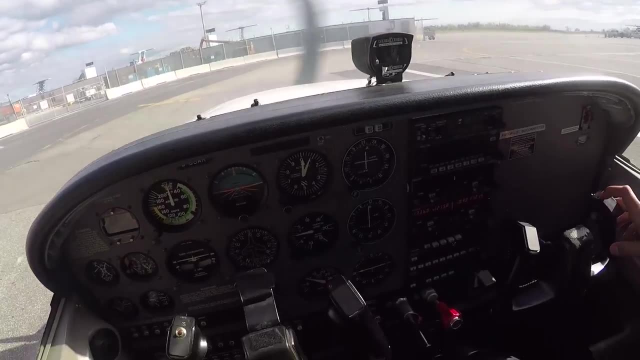 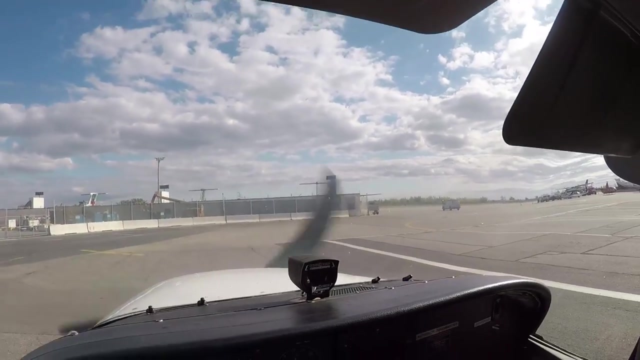 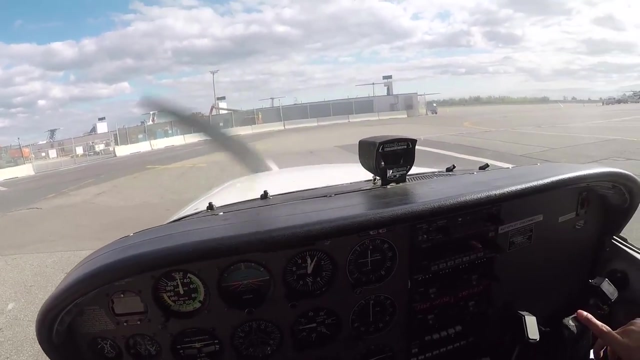 oh, okay. toronto city center airport information. juliet weather at one, niner, zero, zero zulu automated observation wind: three, two, zero. at ten gusting twenty, visibility: niner five thousand broken temperature: one, seven dew point six altimeter three, zero, zero, two the ifr. 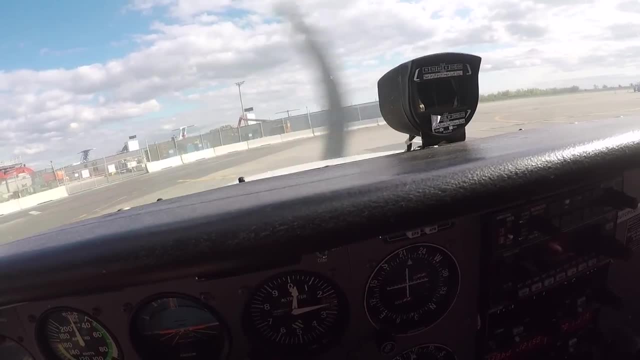 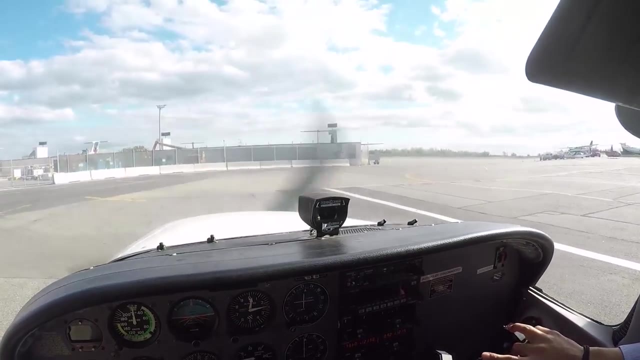 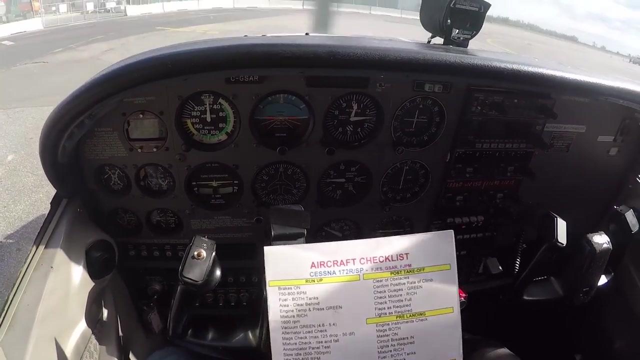 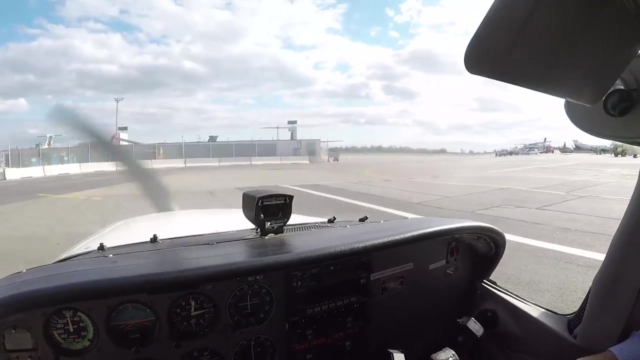 approach is rnav zulu, runway two: six. landing and departing runway two: six. inform agc that you have information. juliet, okay, launch by charlie. and delta contact tower one: one, eight, two. what's the active? runway 26, perfect, so you know what to say. yeah, i know um city ground. 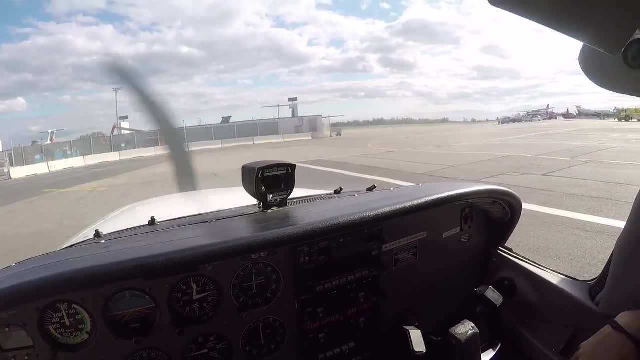 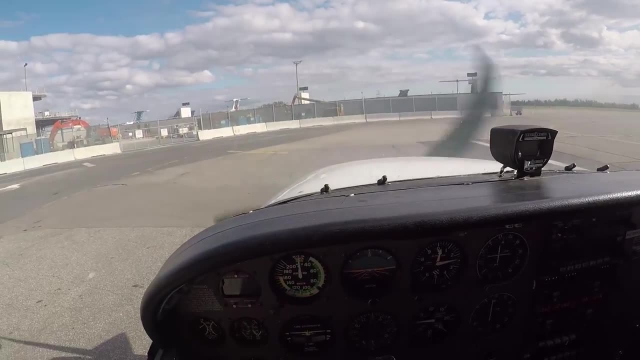 go for it. are we dead? okay, city ground다고 이쪽으로. for romeo hang up on locally. is information juliet, yeah, for romeo: squawk: 1, 2, 4, 1 runway two, six. the winds: three, three zero. ten altimeter three, zero. 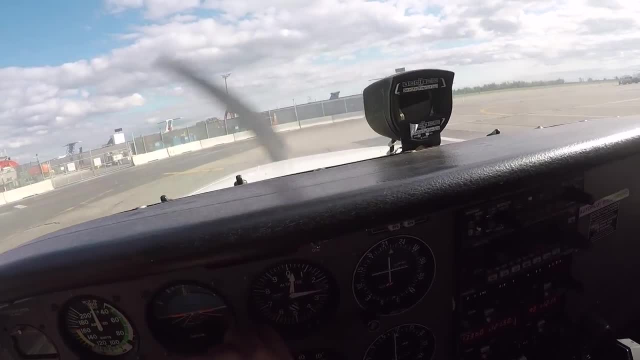 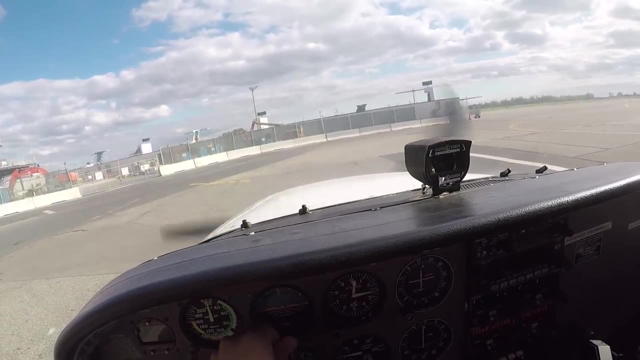 zero three taxirely delta terror woman a2 holding shoulderhana. Hold short 26,. I've got CR for Romeo. Perfect Damn. why do I get a hold short? Dude, you should really just come in and do your radio exam, you'd pass it instantly. 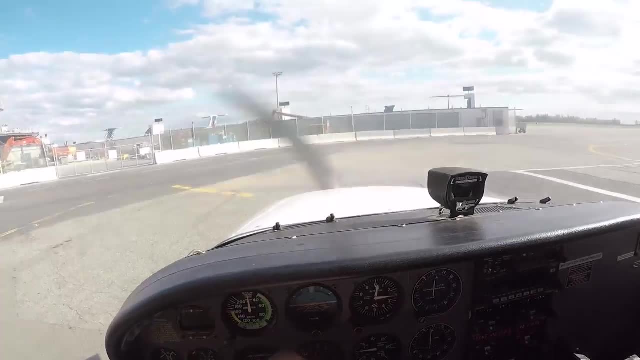 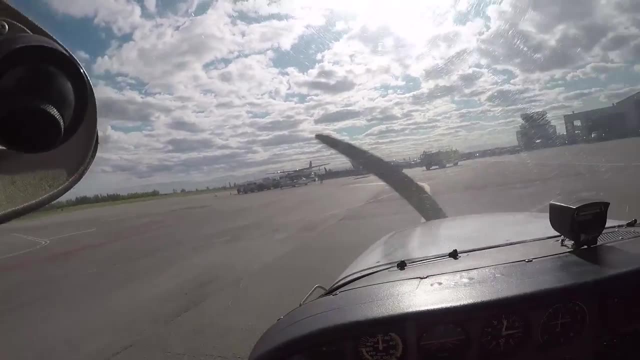 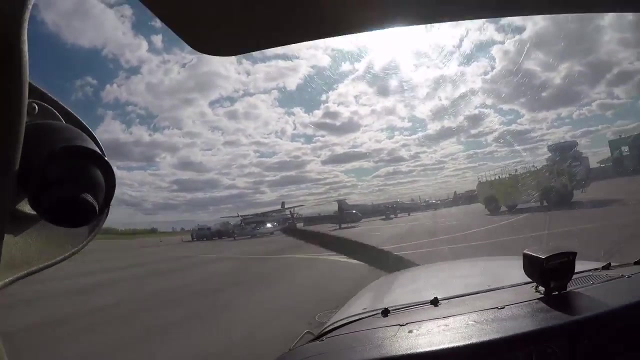 and you'd never have to do it again. This is my simulation practice. Charlie Delta, hold short 26. Charlie Delta, hold short 26. Roger Man, look at the sky, it's beautiful. Yeah, nice day to fly. See if we can go VFR over the top. 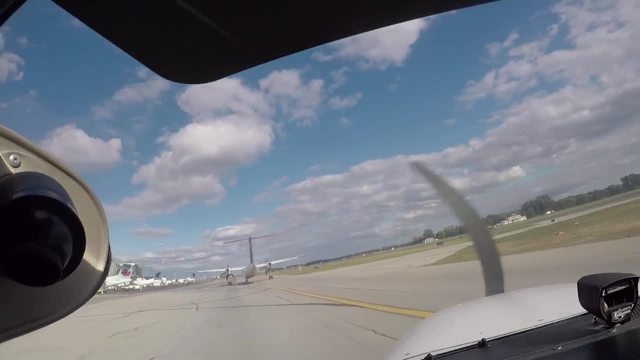 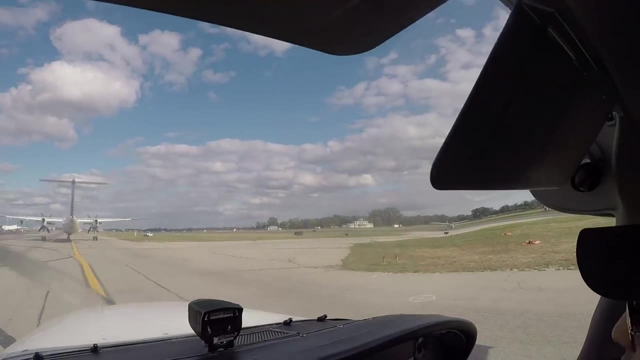 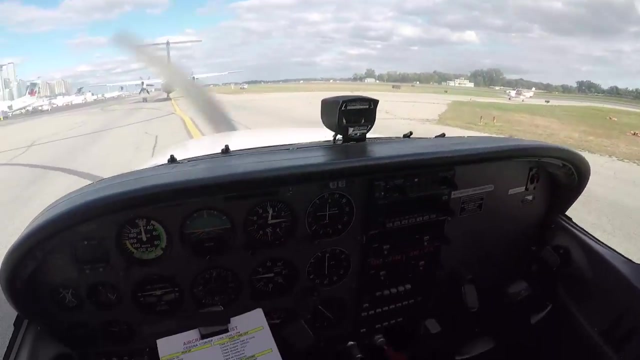 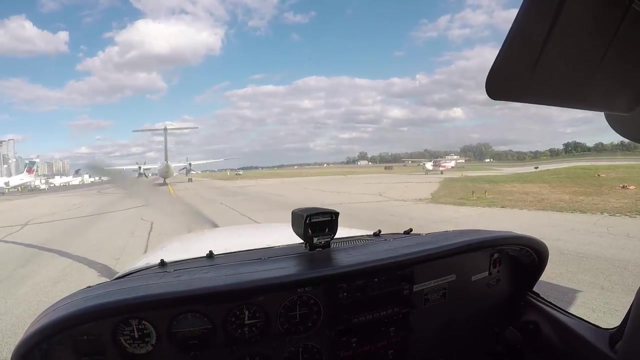 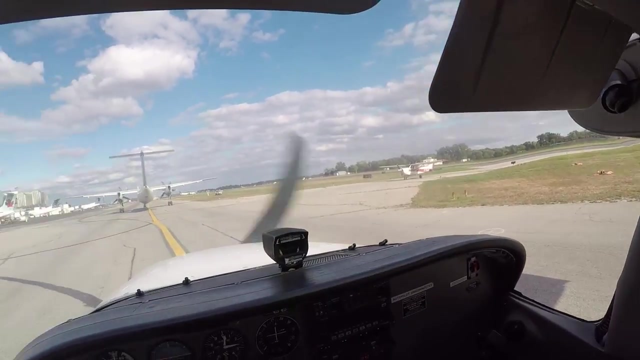 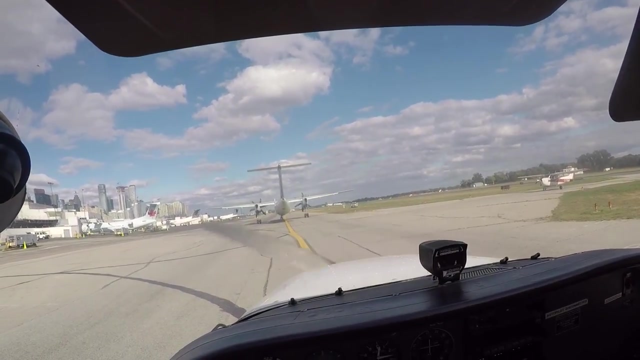 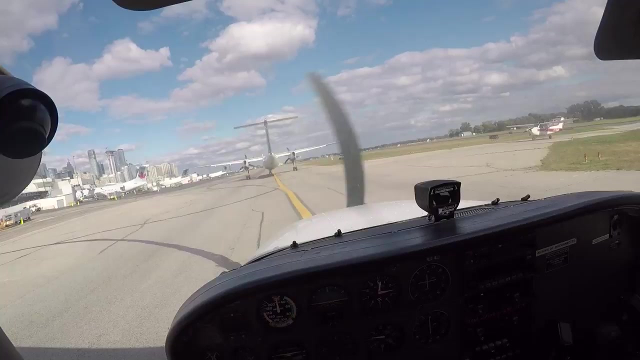 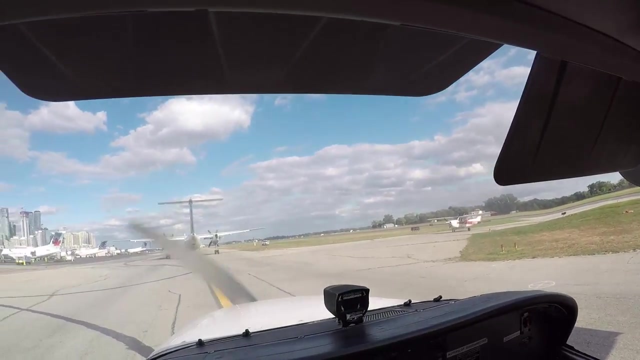 Um, oh, he's going to exit right here. He's like starting up, I'm going to stop right here. Holy, The plane is coming. Would you rather work for Jav? I am, I am jazz reporter. would you rather work for jazz reporter? I mean, I've sat before as. 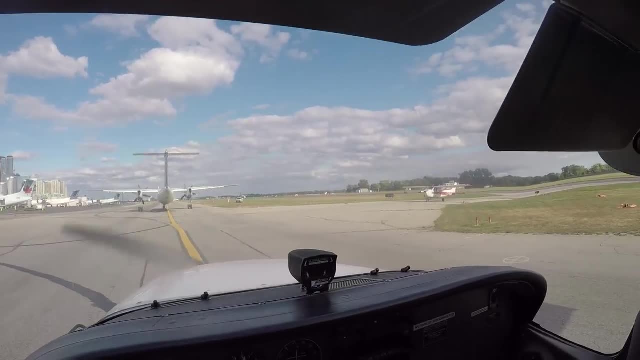 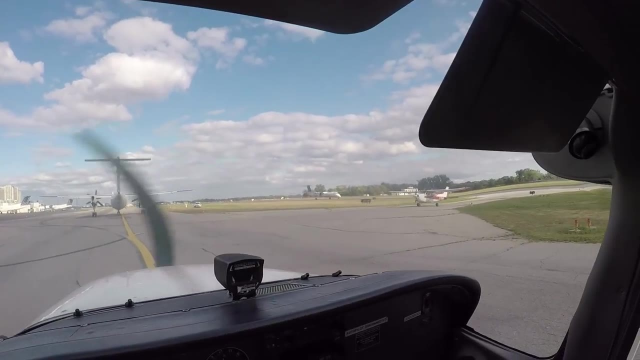 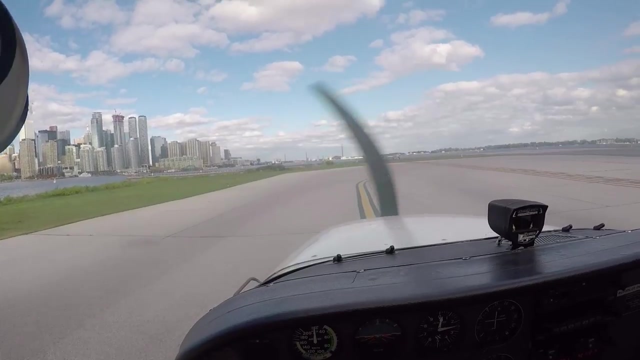 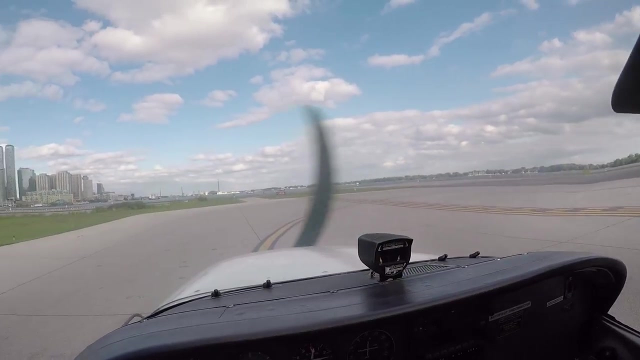 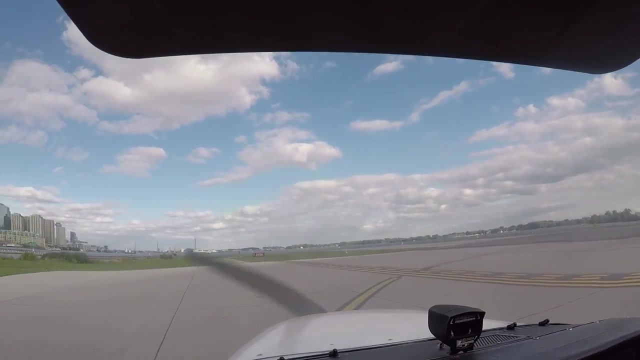 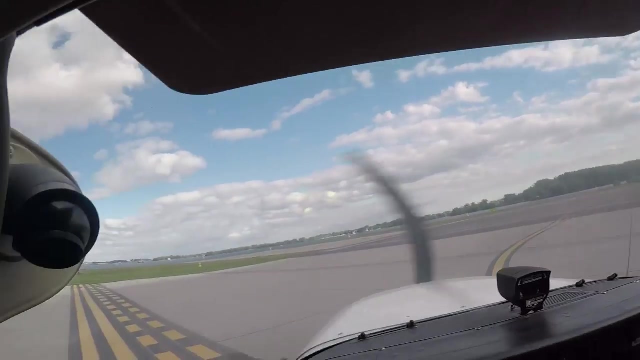 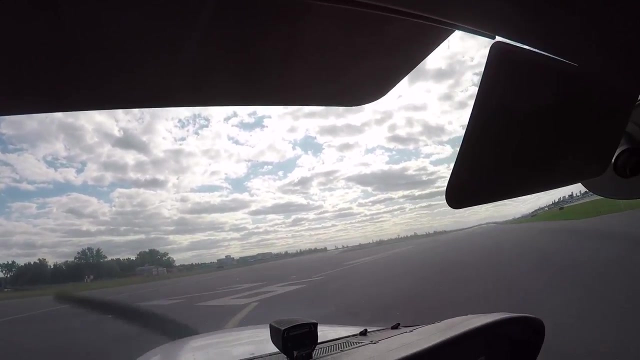 a passenger. I've never did he tell us you are for Romeo, ready at Delta, promises our lineup on the way to six. by never been to six, I've turned out about two point five zero from him seven jet eight, four, one gas noon twenty six when three five zero fifteen altimeter three zero, zero, two. 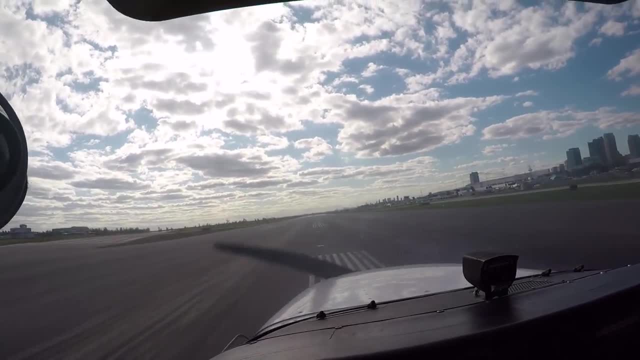 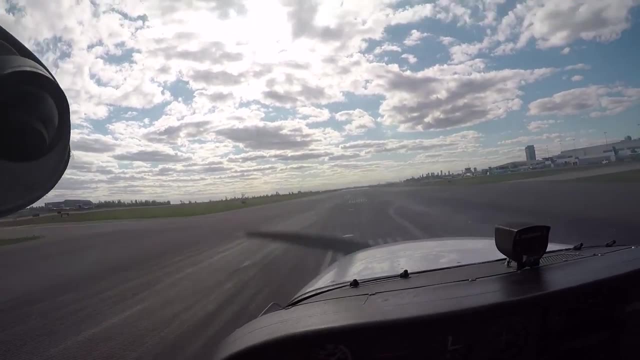 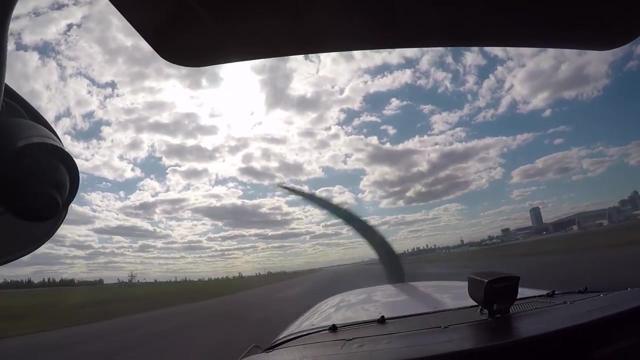 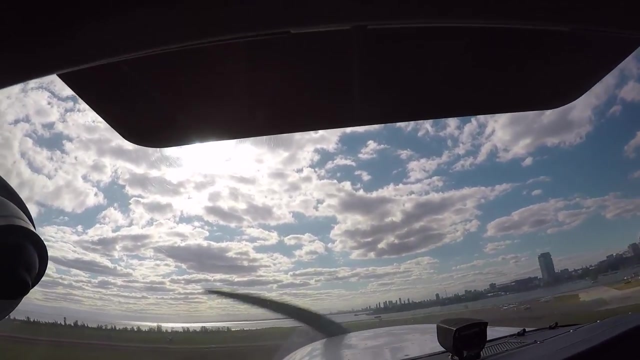 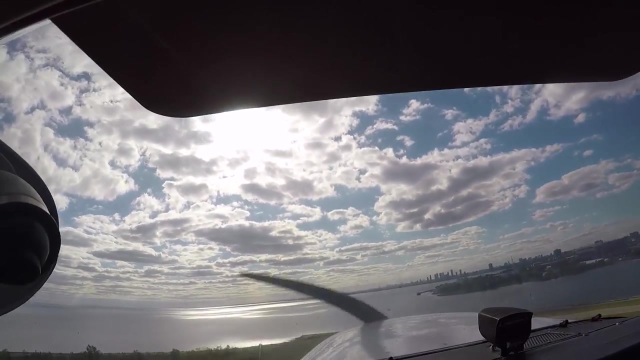 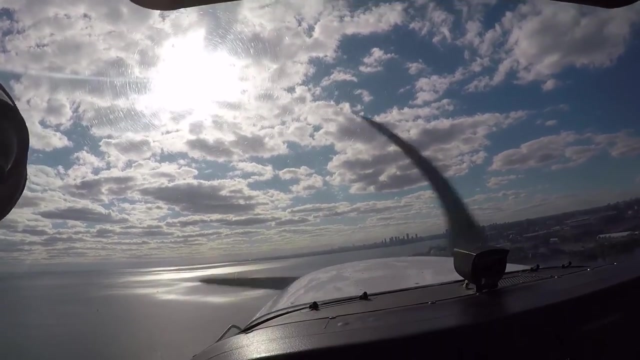 holy. okay, all yours. you run way to six. Oh, that's a bit bumpy today. yeah, it is, so it's a climb, so remember to cancel out that, yeah. yeah, it's even more important on the day when disgusting like it is today. I'm not gonna tell you why, cuz I don't scare you. 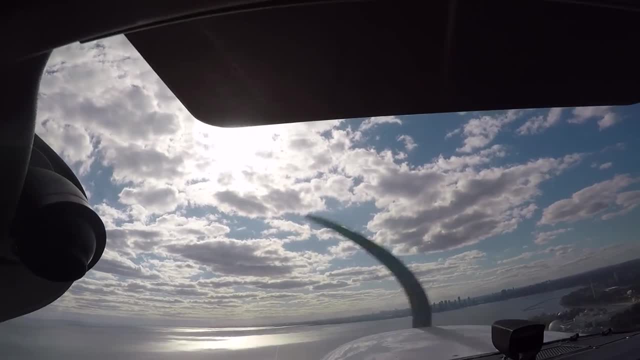 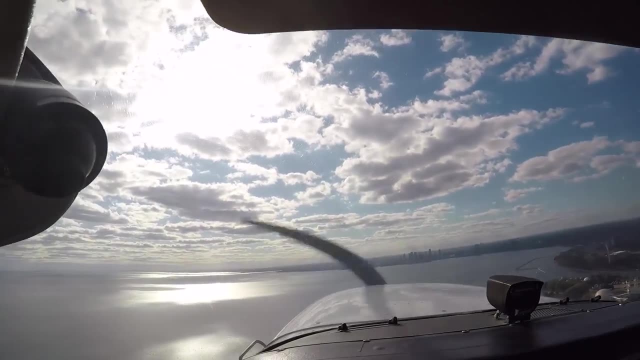 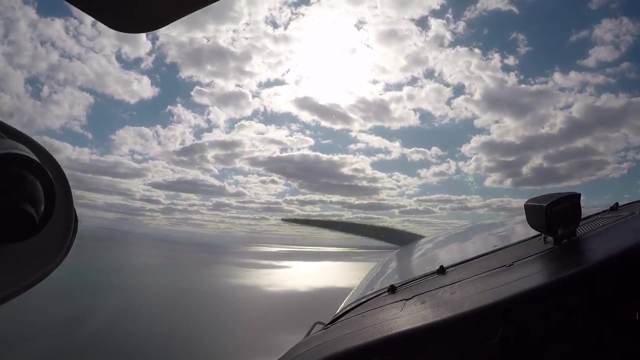 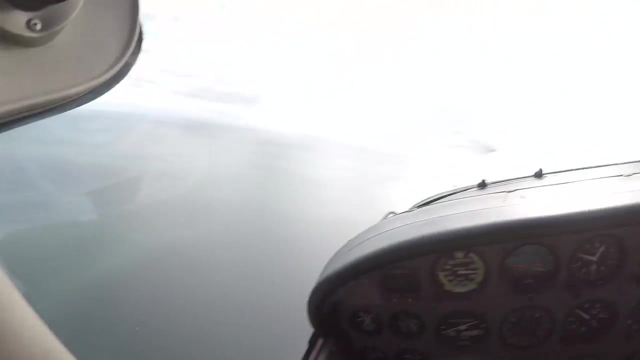 now, it's just a case, you know, the gust is strong enough to make you stall. if you're coordinated, easy recovery. but if you're not sure, everything that's it. yeah, for two, from six eight seven already on the Sun, you, there's a. for six eight seven, Roger, standby for a court. 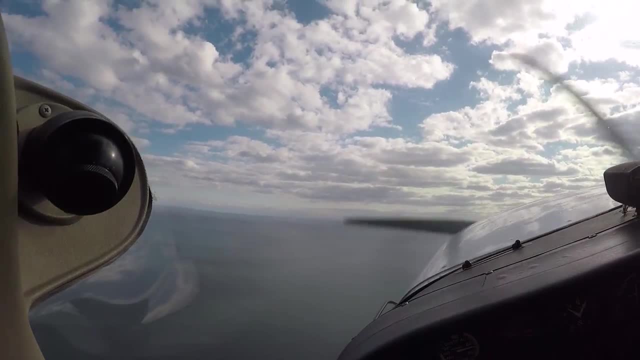 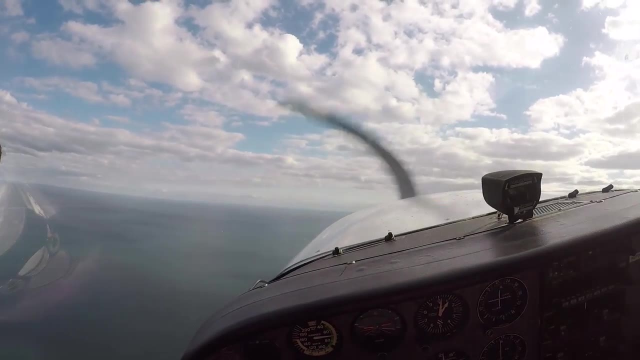 but hit me too. so try flying with one hand on the yoke and one hand on the throttle. only reason being is, or only reason being if you, if you hold on to this with you know, very light, at four to seven you can line up front six. 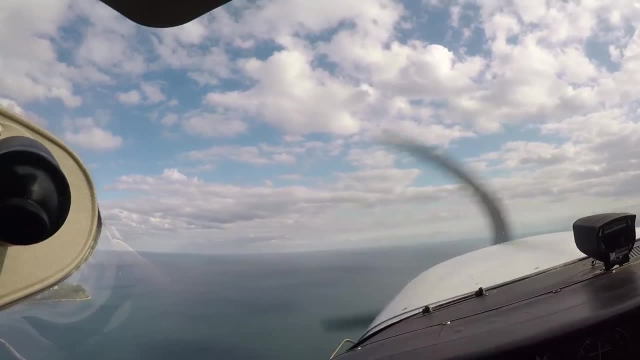 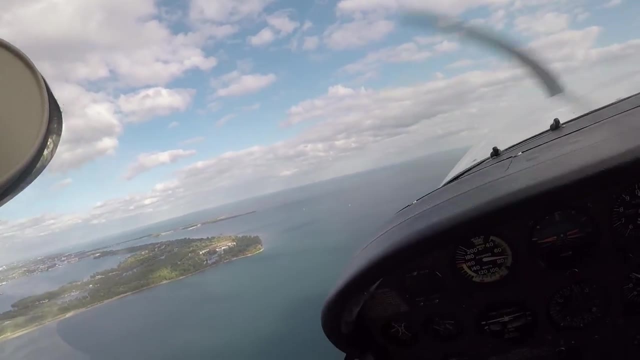 non-departure altitude now 3,000 feet, I guess. touch, then you can really feel what the airplane is doing or wants to do and control eyes. if you have like a, That's great. if you don't really sense that, Yeah, Major 841, you can turn in for the airport any time. 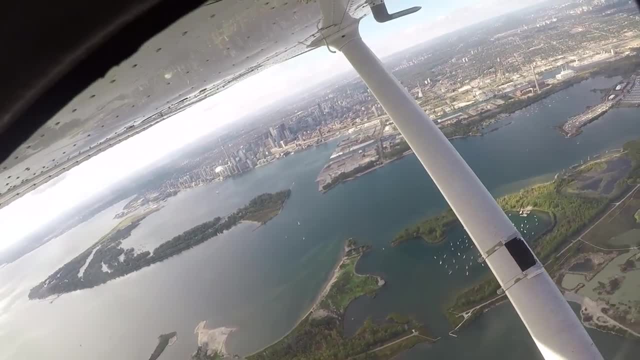 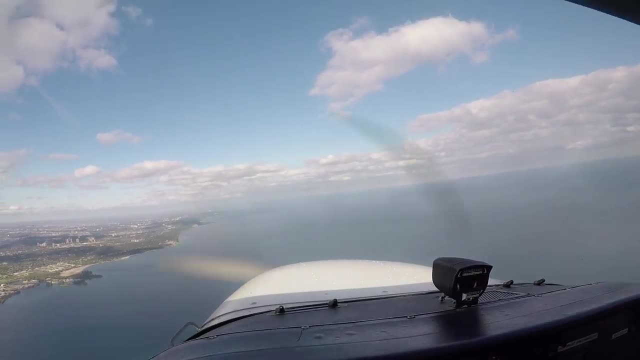 841, we're doing that City Tower. it's Bonanza, Shirley Fox, Gulf of Patango, with you, Gulf of Patango City. descend to 2,000 feet, altimeters 3003, through city control zone. 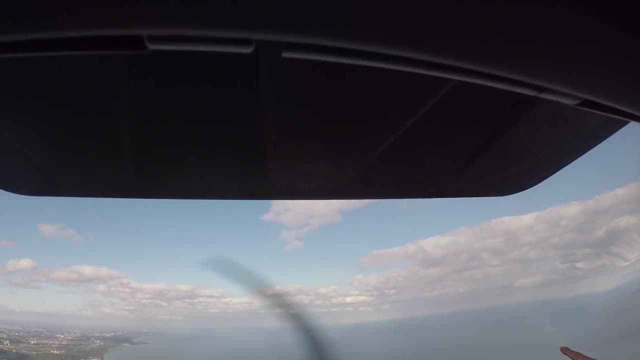 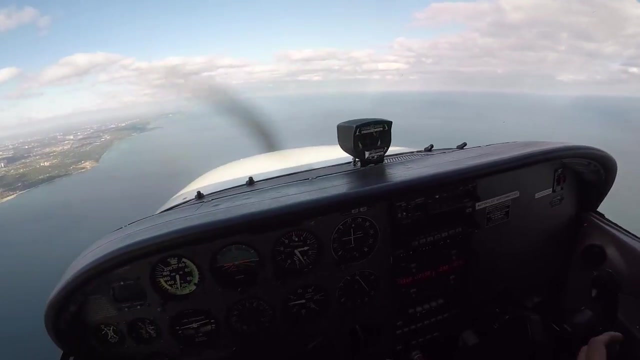 past north of the CN Tower. Look, you can see the sun rays coming down from the clouds. Do you have a notebook or something? No, Here you can use this. do you have a pen? City Tower- I'll give you that too. 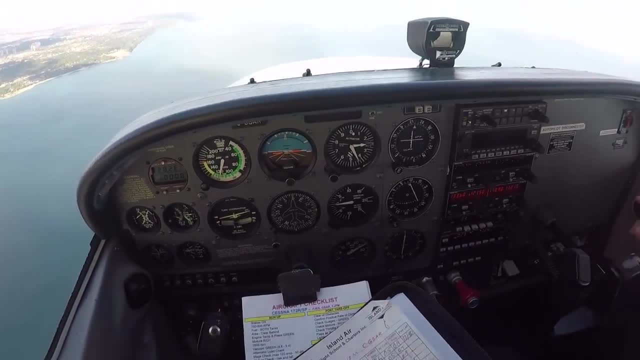 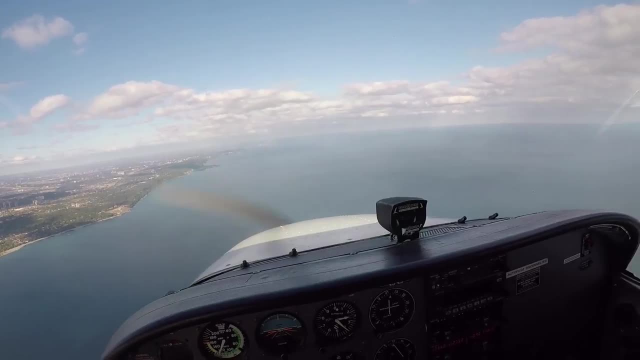 So stick the HOB sheet inside the little pocket there and use this scrap paper on the back. Here you can use this pen, And what I want you to do is basically 7J841, Exit Echo, if you've got it all the way down. 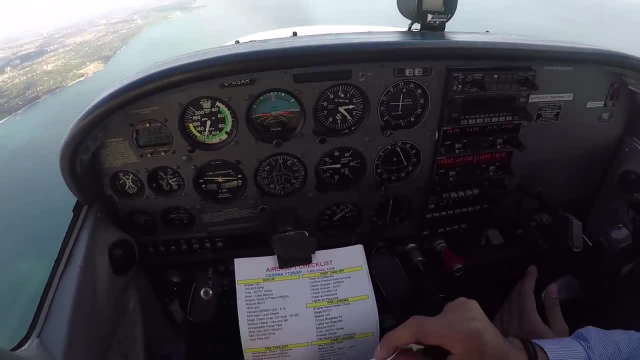 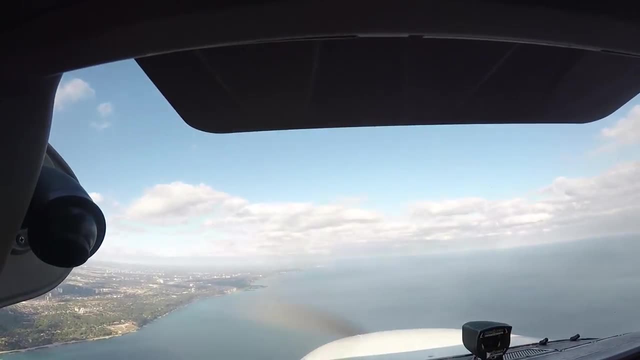 to the end of knots and over the ground. 121.71, off-run. OK, so put this in here, just so you have space for right. We don't want to lose that sheet 7J841. And make three columns like we did in the grad school class. 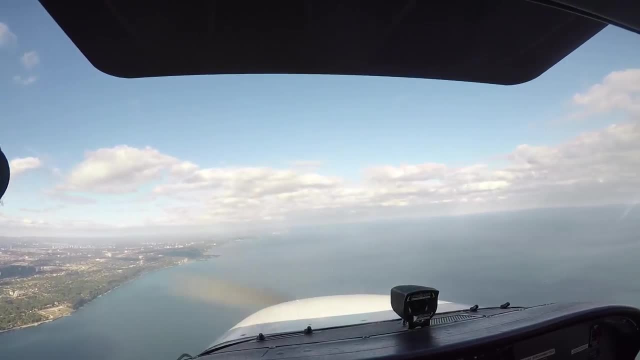 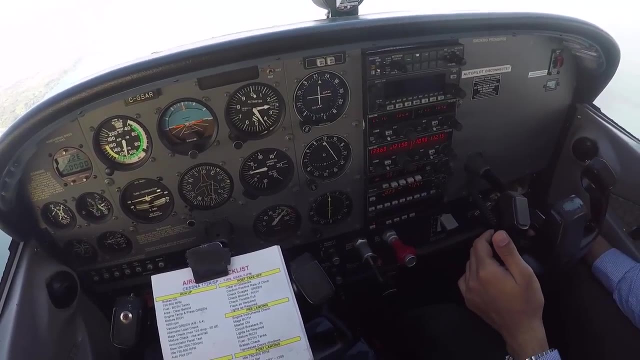 Ideally, when you do this, you're not going to be right. You're going to be riding in your lap just because it's, let alone efficient. It's just not good to be stirring inside when you're VFR pilot, But it's good for your first lesson. 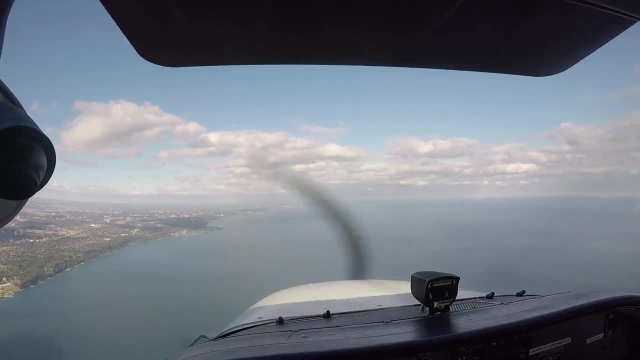 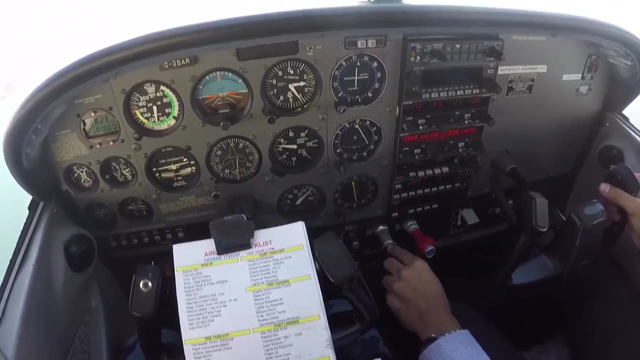 so you know how to do range and endurance. So, right down to a bunch of RPMs, We'll start with 2,000.. Very nice, And what we'll do is actually: why don't you tell me what we'll do? 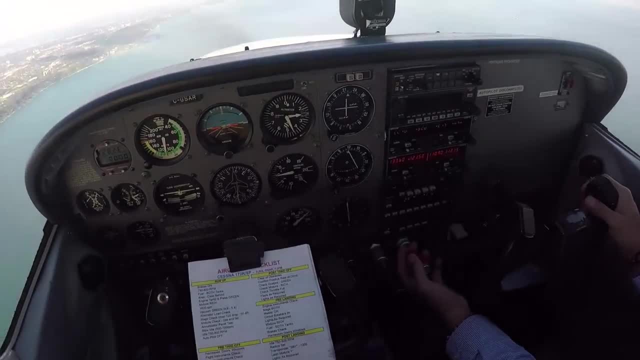 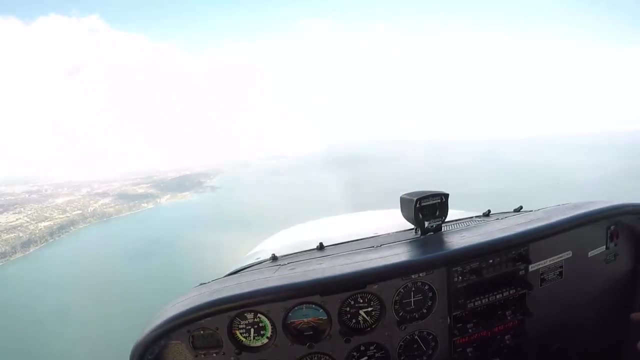 How are we going to find best range? Well, I'm sure Best range. We're going to go up into the engine over town about 3,500 feet sending 4 Cs down towards. So how would you find it? 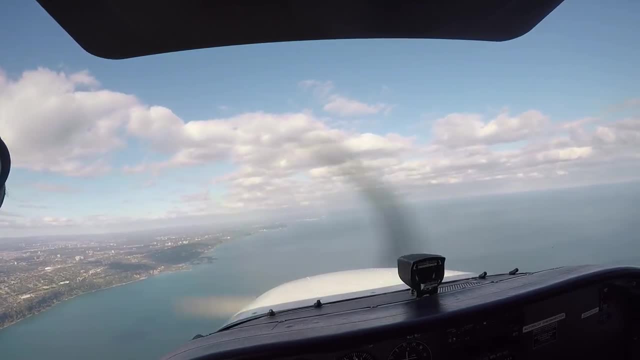 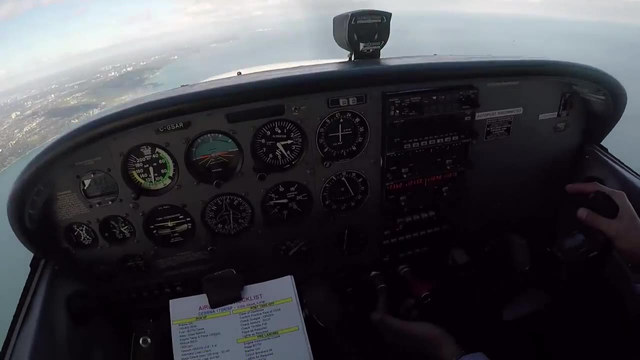 We'll drop our RPM and check on the airspeed. So when there's a major drop, so we'll go back to the previous RPM. Perfect. And what about endurance? What about endurance? OK, so we'll check if our altitude is dropping or not. 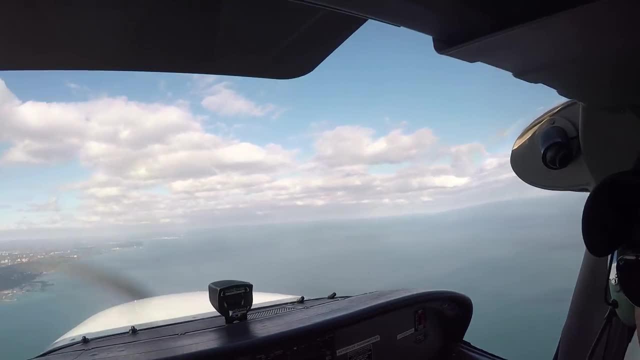 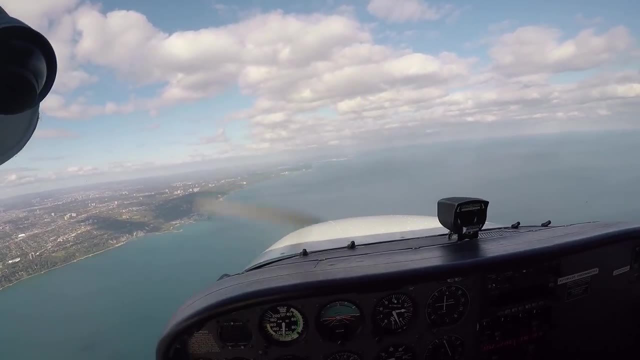 by decreasing the RPM. So when it drops, so we'll go one notch up. Perfect. So what I'll do is, once we get to altitude, I'll demonstrate it for you, And then I'll have you do it by writing it down on paper. 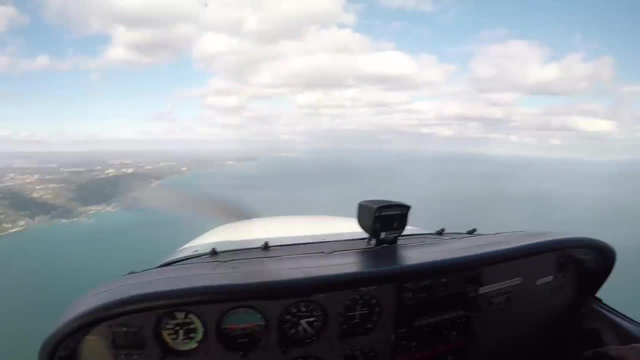 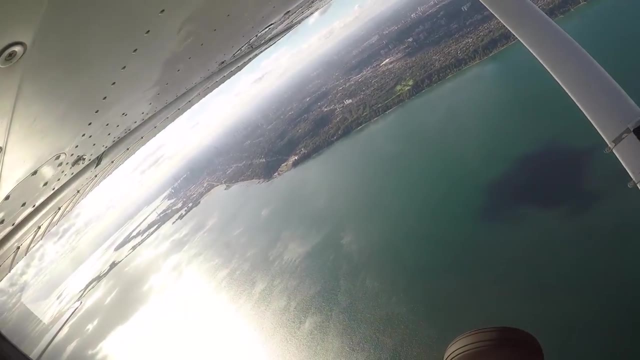 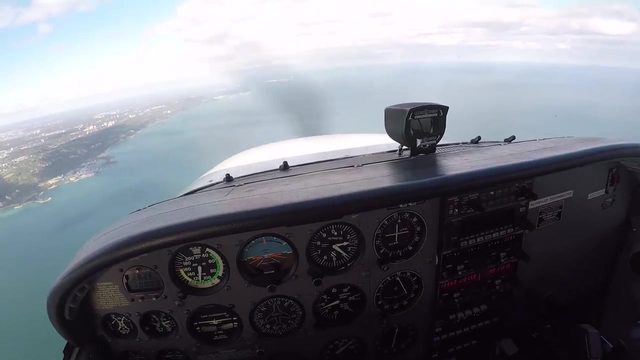 And I'll have you do it by not writing it down on paper, just so you get proficient at not having to use my notepad In the meantime. why don't you lean out the mixture for me, just while we're getting there? 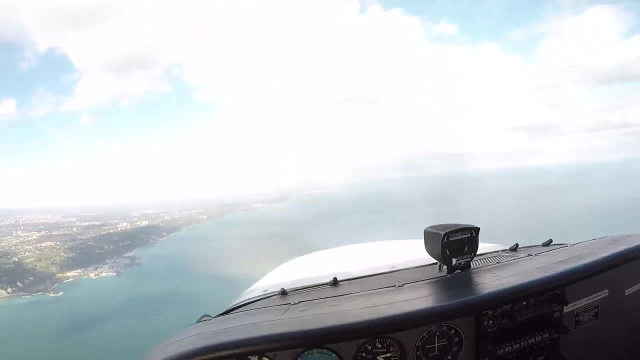 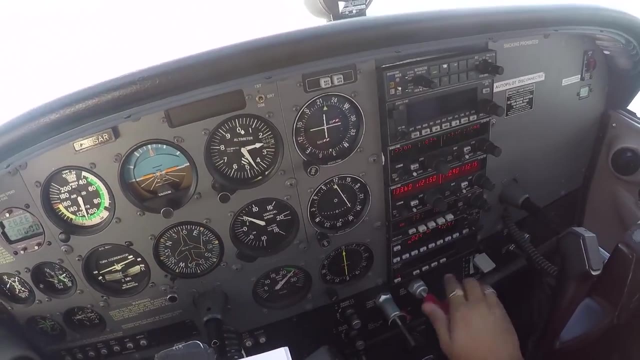 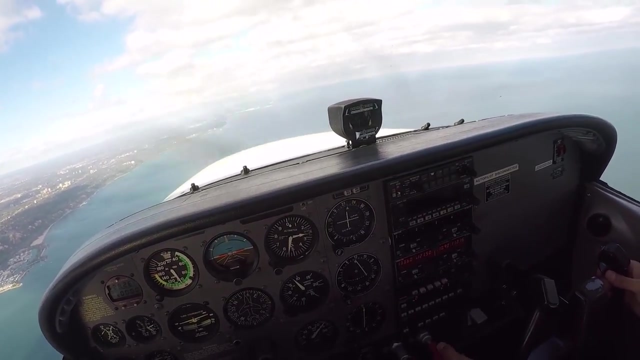 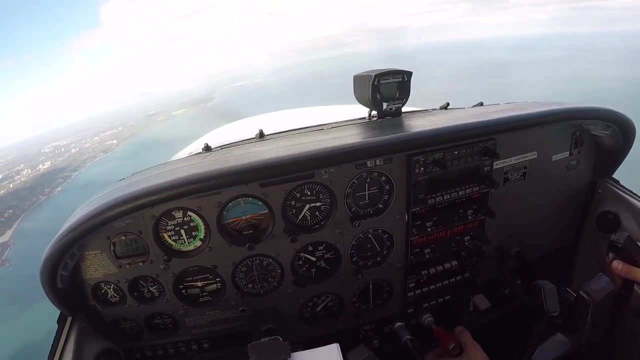 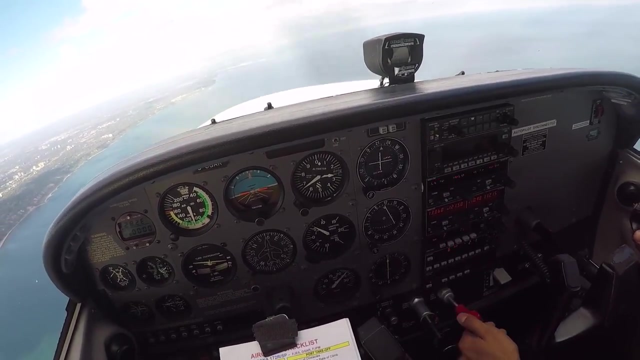 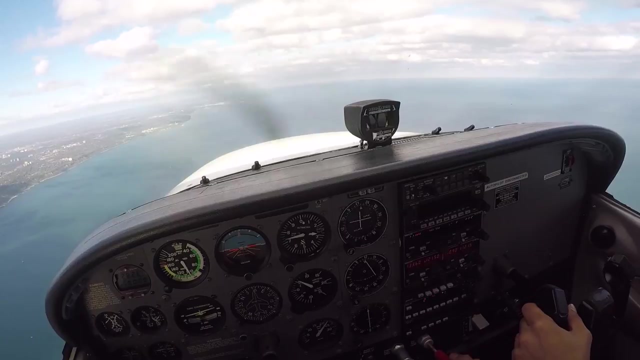 Like perfectly leaned- Damn this I am. I have to lean forward, Is that correct? Let's see, It is windigting. I see the deflection too. Man, it just doesn't want to lean. There we go. Oh, so a major drop, Okay. 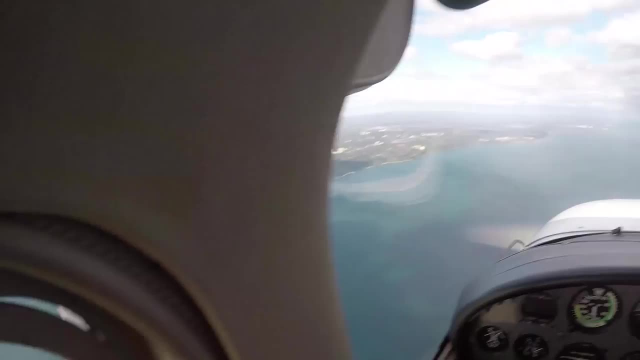 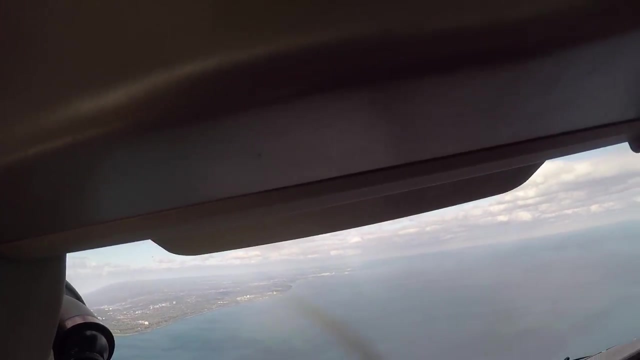 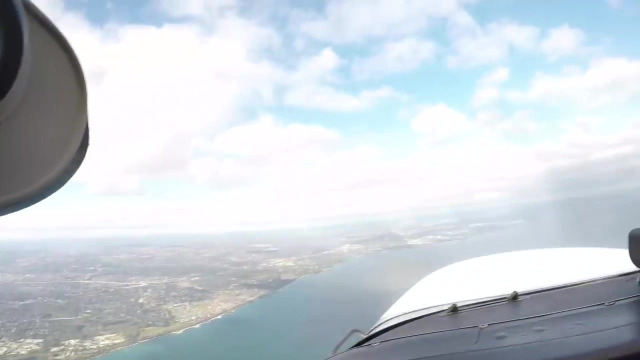 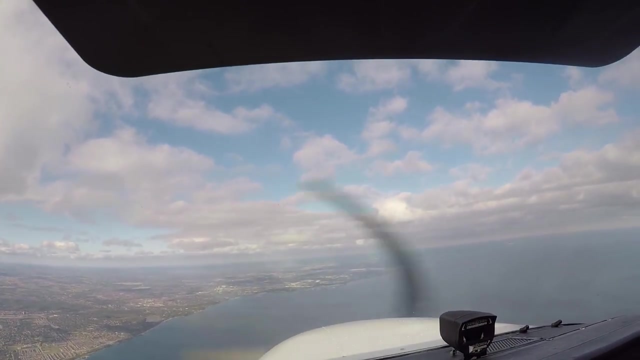 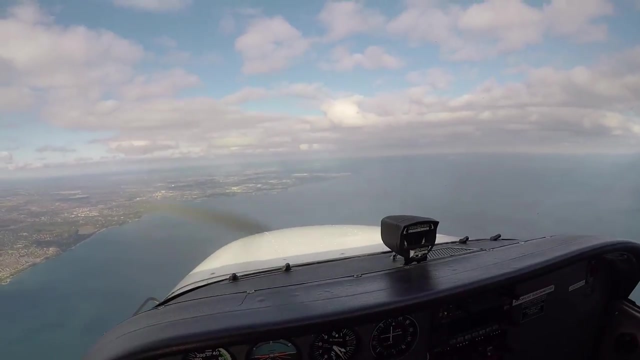 Okay, very nice. What the hell was that? What do you call it Tickling? Okay, level out at 35. Run complete Check. So it's attitude first, then power, then trim. Okay, so I'll take control. I'm going to show you best range. 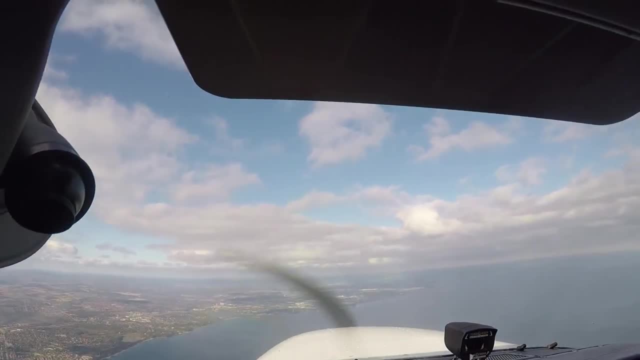 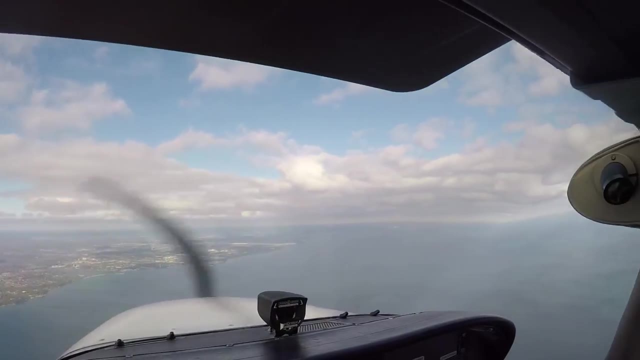 Let me close this Kind of cold in here. We'll start off with best range, So I'll have you write everything down and then we'll do it again. You want me to write the airspeed? Yeah, So we'll start off with best range. 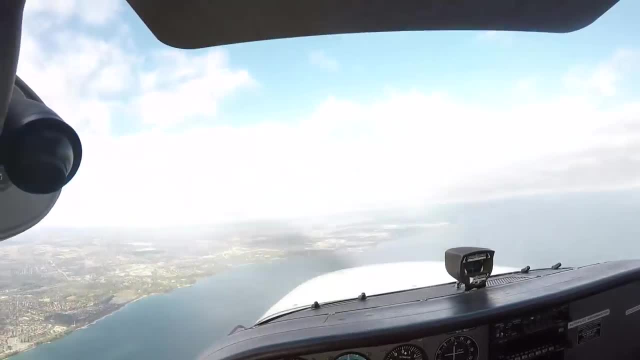 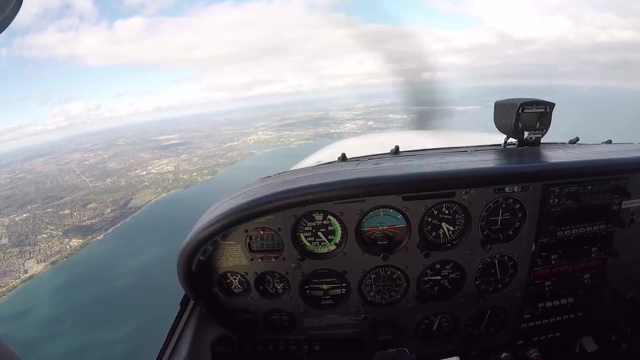 So we'll start off with best range, We'll start off at 2,000, like you said, and we'll let everything stabilize, right? Okay, Waiting for everything to stabilize, You want to make sure that, while you start at 2,000,. 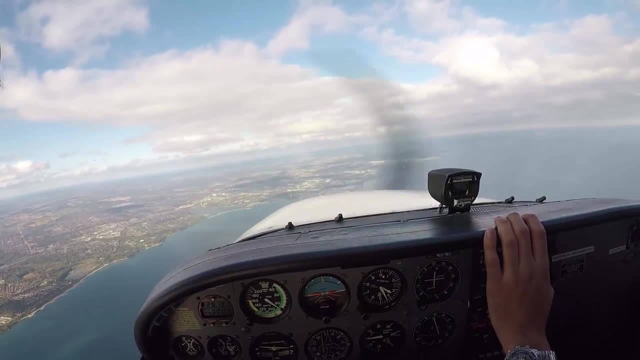 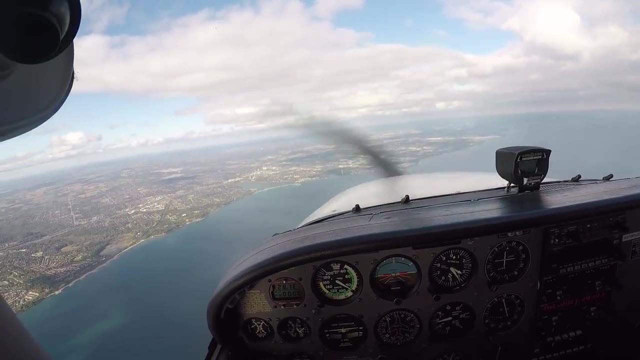 altitude is not changing and airspeed is steady enough for you to actually use that as a reliable reference. So what are we at right now? 85 knots, 86? Yep, 86 knots, Okay. So why don't you write down 85 knots? 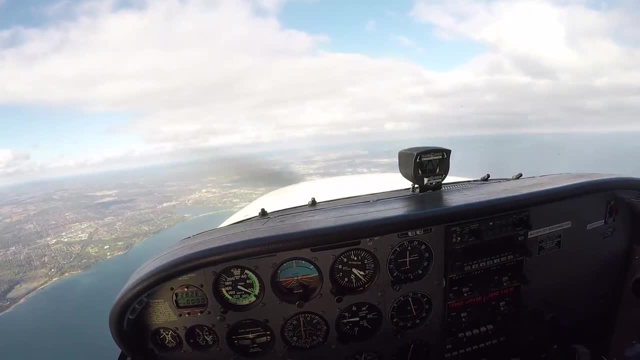 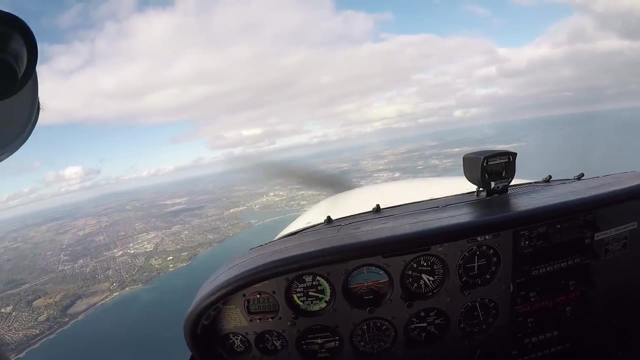 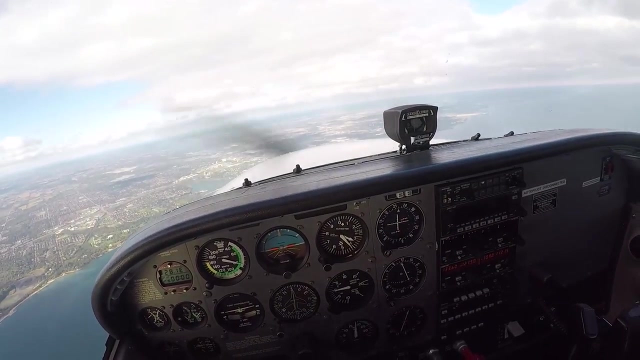 And then we pull it down to 1,900.. Now we know we're going to have to slow down to maintain altitude. We're at about what? 80 knots Yep, We'll pull back another 100 RPM. Yeah, left turn. 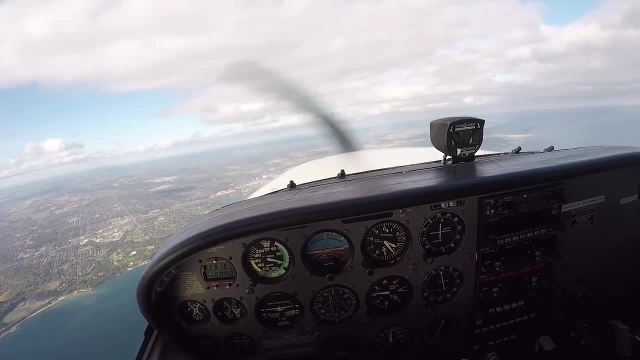 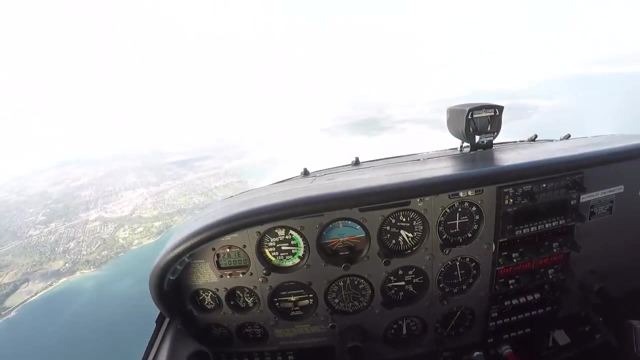 Left turn outside of you, Roger. Roger, Looks like we're about what? 75?? Yep, So pull back or right down. pull back another 100, 1,700 RPM East of the town of Mount Albert, at 3,500 feet. 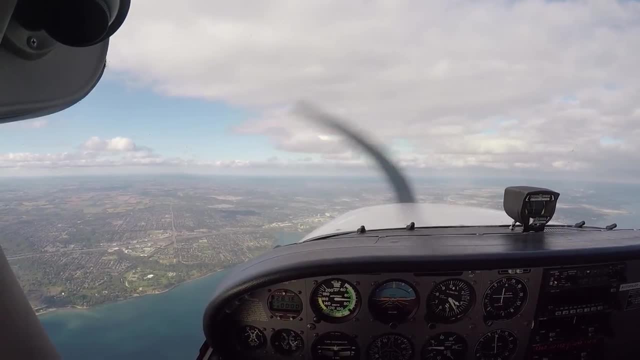 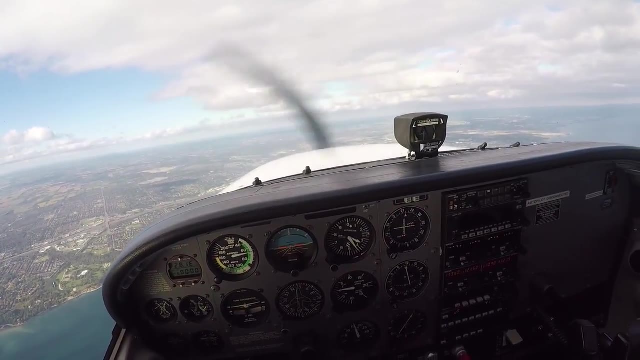 We're going to stay on the east side of the town of Mount Albert called Papa's Avenger. Okay, what are we? 70 knots? Okay, pull back another 100 RPM. Whoa, that's a bit too much. Yeah, we were happy to come out of there. 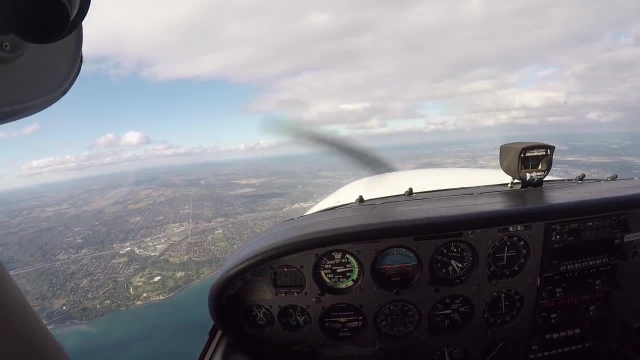 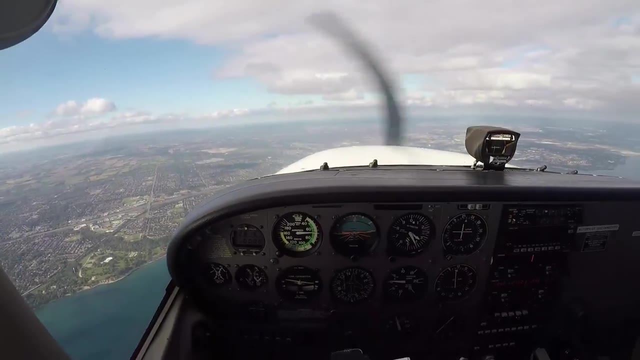 That felt heavy too. I was like whoa, 0-1.. 0-1.. 65 and 1,600, so we'll put out another 100 RPM Now 1,500.. This is why it'd be a bad idea for slow flight today if it's this gusty, just because you know. 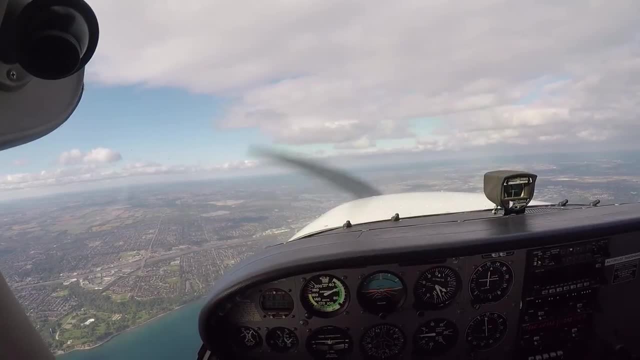 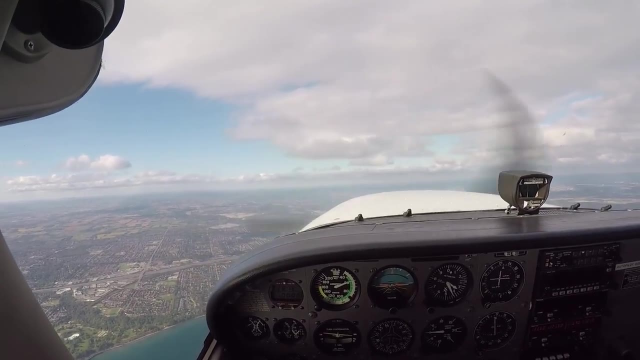 Yeah, it's 60.. Oh, it's 50.. So 1,500 RPM If we try not to lose any altitude. Look, we're at 55.. You can hear the stall warning horn. We're still losing altitude. 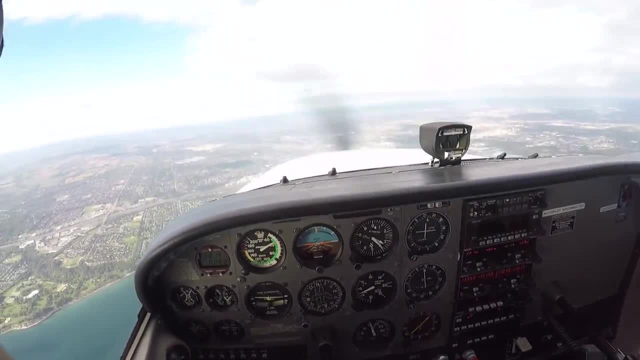 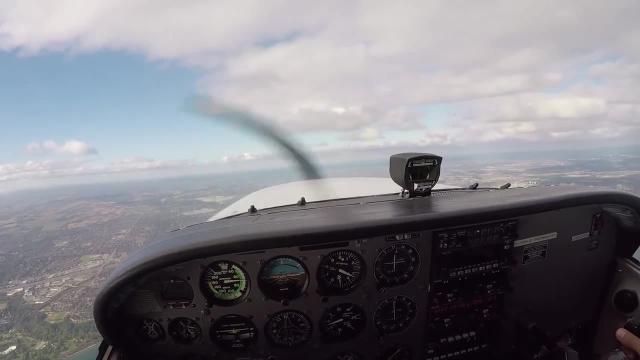 So we know best range is probably 1,600.. 1,600 RPM- Okay, okay, Right, Yep. So what you want to do is some people will go straight back to it. That's not wrong. but what I found is at that point, if you transition to slow flight, it's 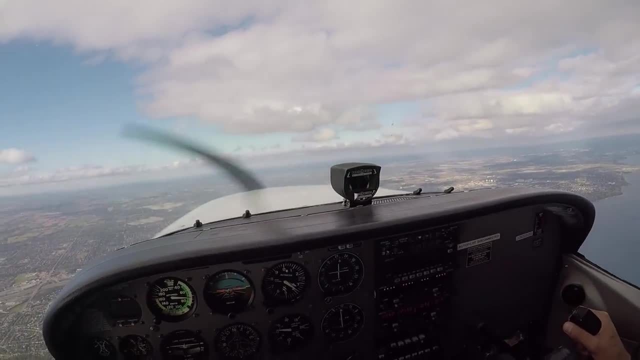 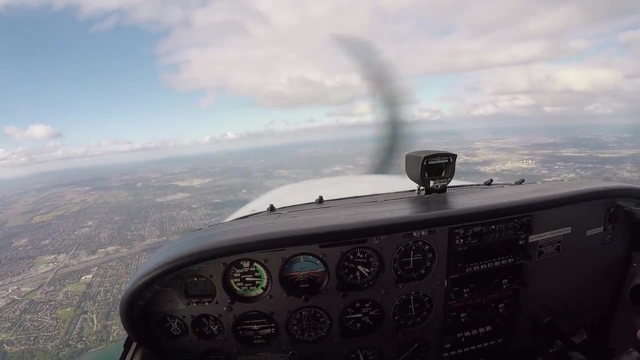 harder to actually find that area. So accelerate back, get back to your altitude, if you lost any, and then just pull up straight to 1,600.. Okay, For best range, trim it out and then you should be expecting wood speed 65, right. 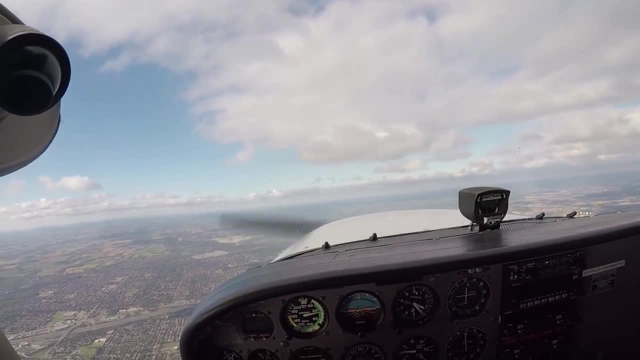 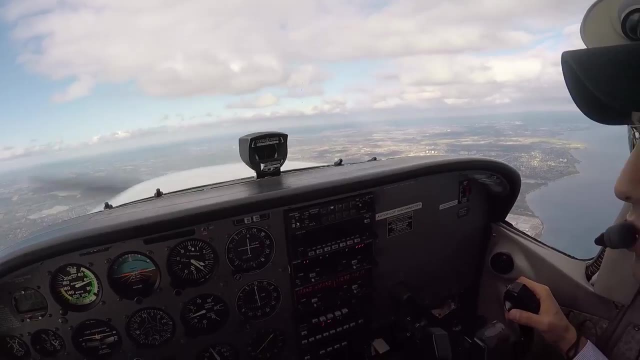 So let me ask you right now: Are we in best range? Yeah, Are we going to maximize our fuel consumption or maximize our distance traveled based on the fuel consumption right now? Oh, it's not 1,600.. Okay, Are we in best range? 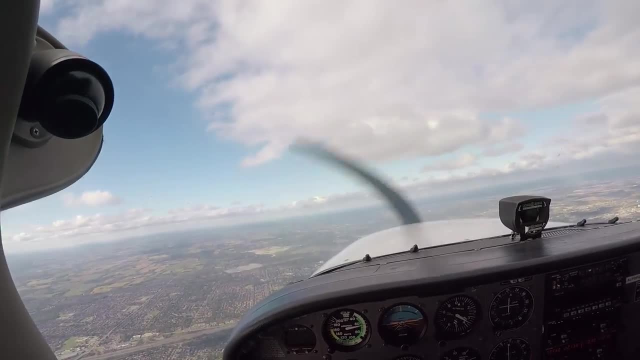 Yeah, I think so. Are you sure? We are not losing any altitude, and almost 55. Is this the best fuel consumption we can get, though I think we have to lean out Right There you go, So you're going to lean out the mixture. 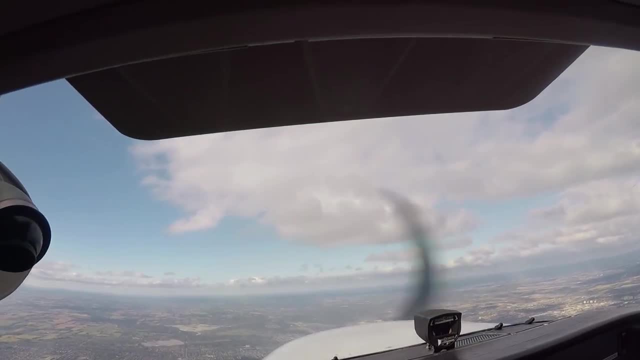 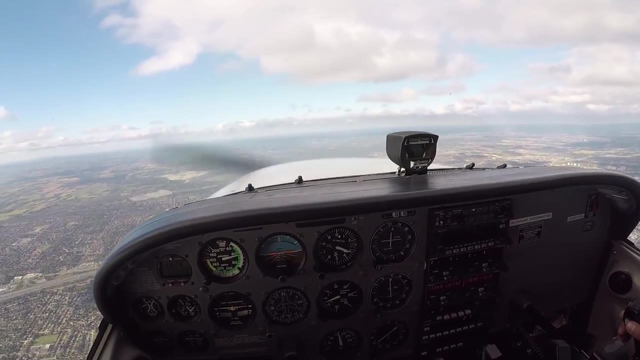 Best range, Yeah, Best range, Yeah, I think we have to lean out. Right There you go, So you're going to lean out the mixture: Best range, Yeah, Best would be to, you know, do exactly what we did on our way here. 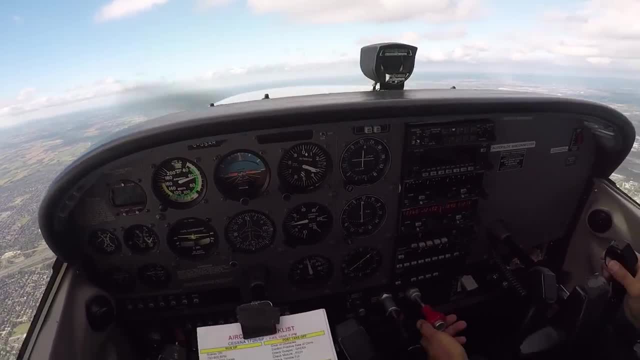 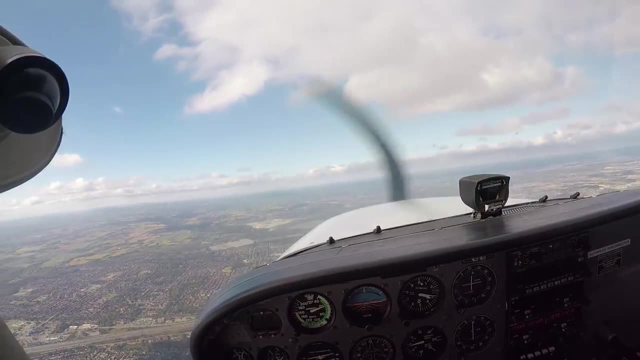 Okay, We're looking for the drop, See. So we got a little bit of a drop: One, two, three. Now we're in best range. It's a bit bumpy, so we're getting thrown around, but this would be best range. 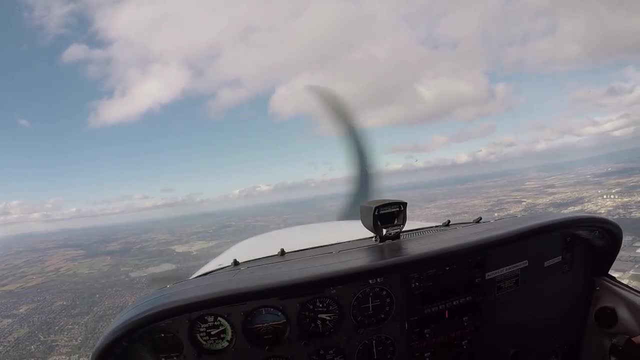 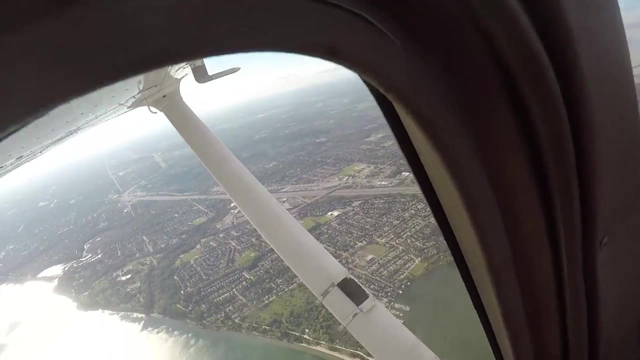 Oh yeah, I see. Oh, we're below 16.. Sound good, We are losing altitude. Okay Yeah, Sounds good. Same thing with endurance, except this time with endurance. Yeah, Yeah, Yeah, Yeah, Yeah. 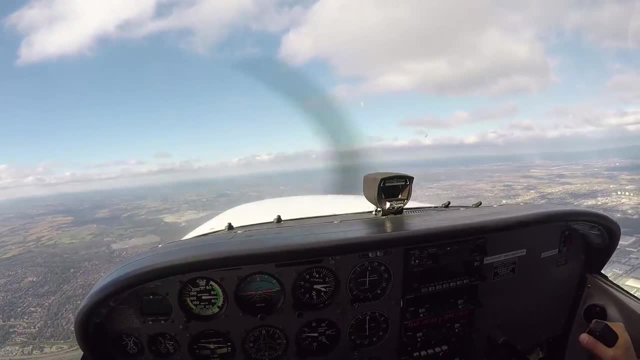 Yeah, We lost some altitude there With endurance. instead of checking the airspeed, we're going to be checking your altitude- whether or not you can maintain any altitude or maintain your altitude. Okay, So I'll just start at 1800 now. 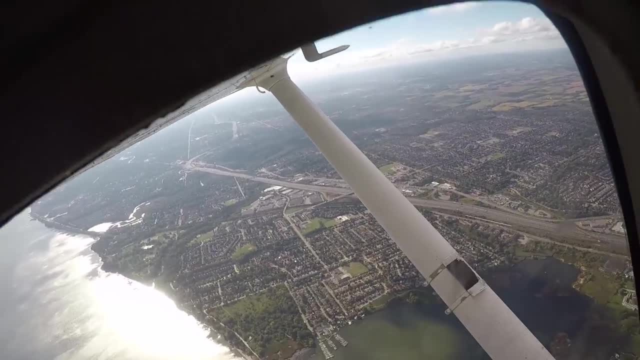 Just speed it up so I'm not wasting your time. 1700, can we maintain altitude? All right, I got it. We got 200.. 600. I got it. Wow, Oh my God, This is a great jump. 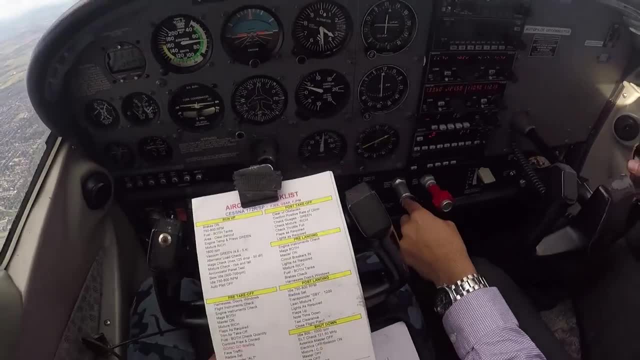 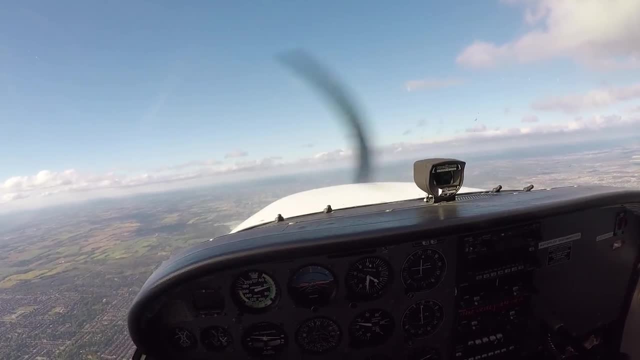 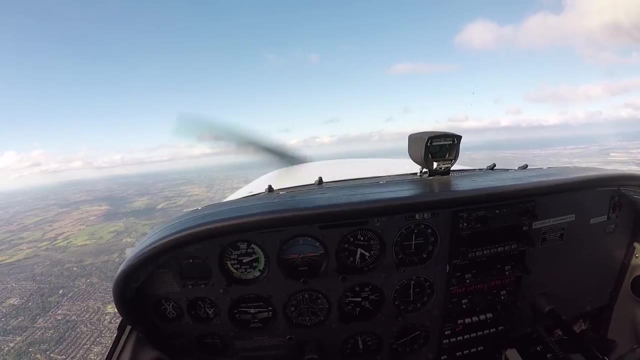 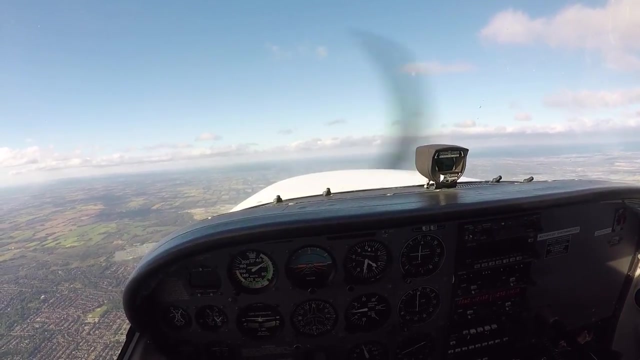 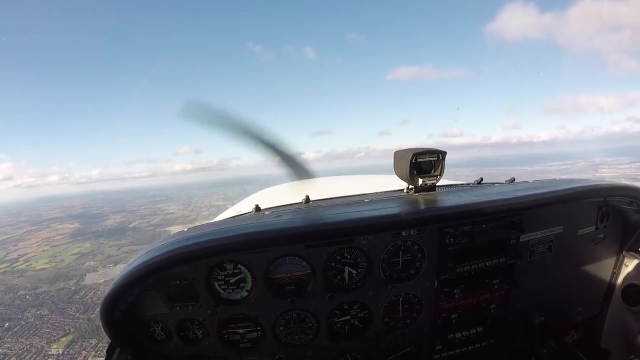 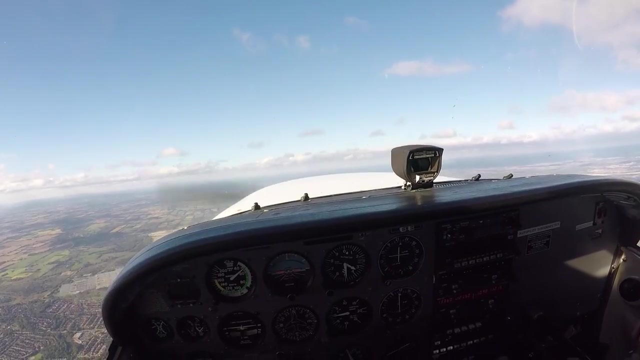 All right, Second stable, just waiting for everything to stabilize 1600.. We have the stall warning horn going off, but we're at 1500 RPM right now and we're not losing any altitude. The horn is kind of annoying, but this is essentially almost best endurance. 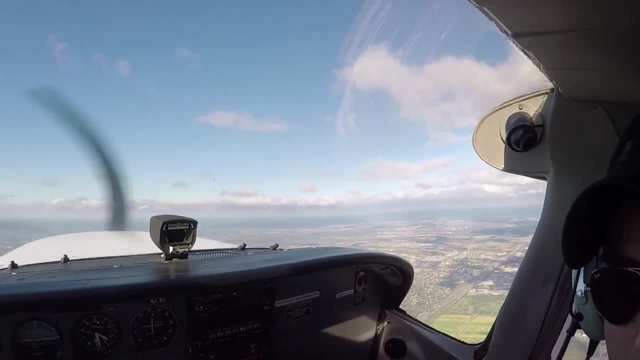 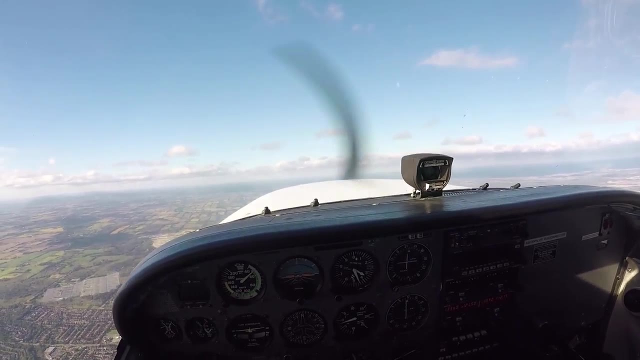 What's going to make it best? endurance: You want me to stall warning on Huh. You want me to stall warning on? Yeah, because we're at the lowest power setting possible and we're able to maintain altitude. Oh, okay. 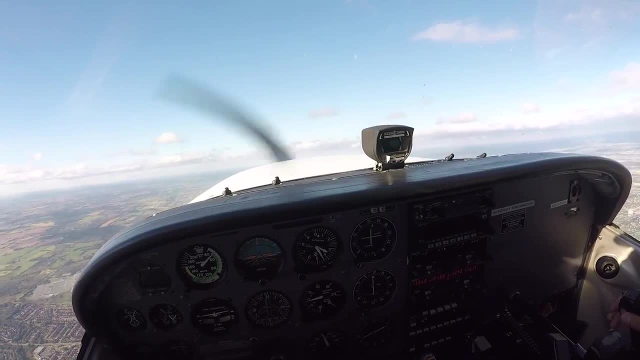 Oh, I see, I see Right, It's kind of sketched that you have the stall warning horn. Oh, we dropped a little bit there. It's kind of sketched that you have the stall warning horn on, but this is essentially what. 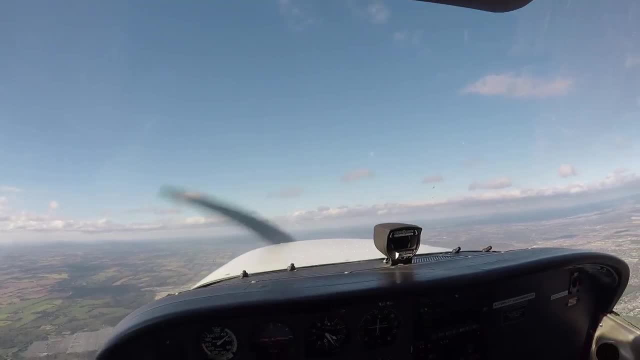 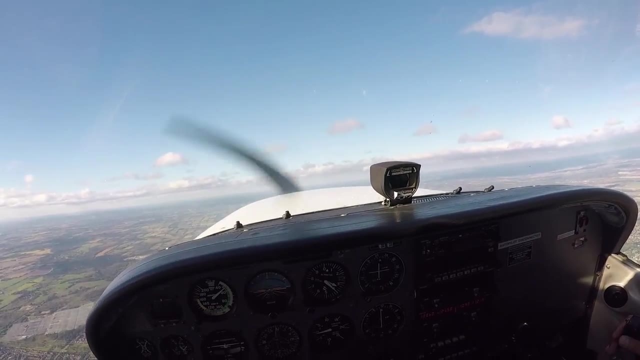 best endurance might look like. Okay, I mean your airspeed's a bit low, but this is basically how you find it. Are you in best endurance Right now? Yeah, almost. How are you going to get into best endurance? 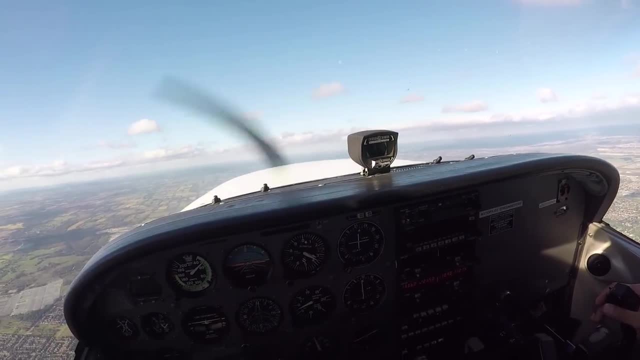 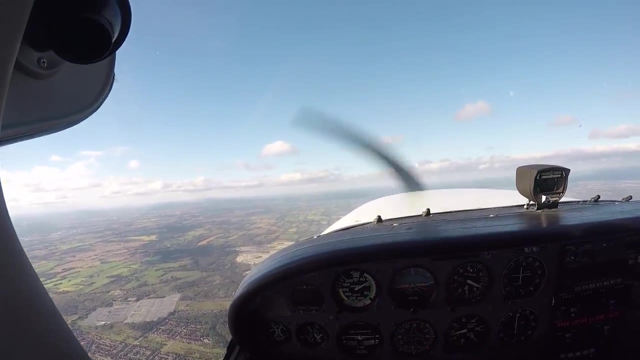 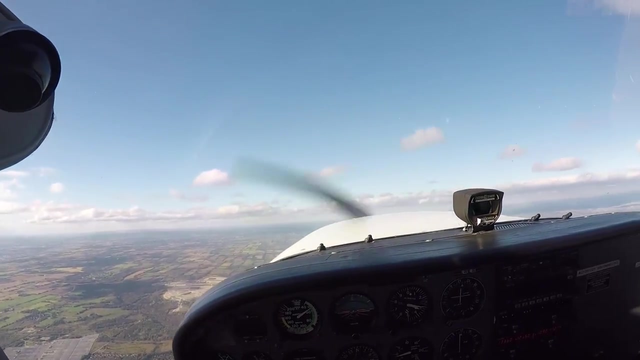 Lane mixture Right. So we got a lot right there. That's how you find best endurance. So notice the speed: 55 knots is better or lower than best range, right? Okay, That's basically it. You're not going to get tested on this for your flight test, but it might come in handy. 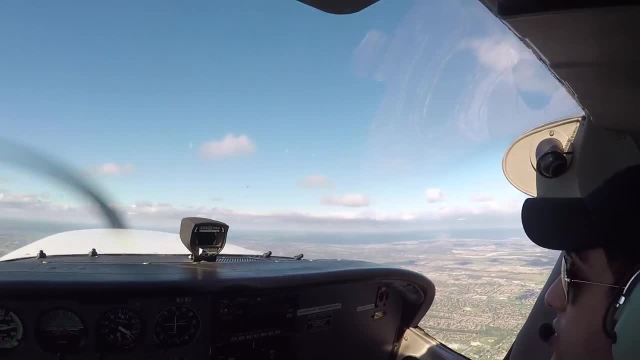 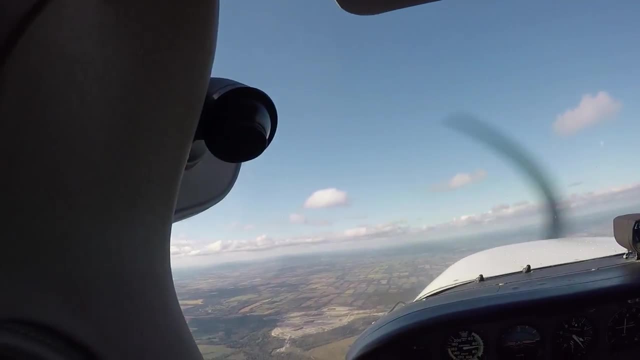 when you're, Yeah, flying as a PPL yourself. I actually had to use this when I went to London for my cross country and I did a 150 with my roommate and she was outside looking taking pictures and I looked at the gauges. 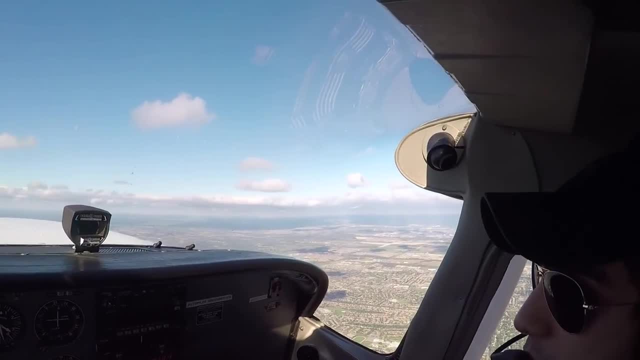 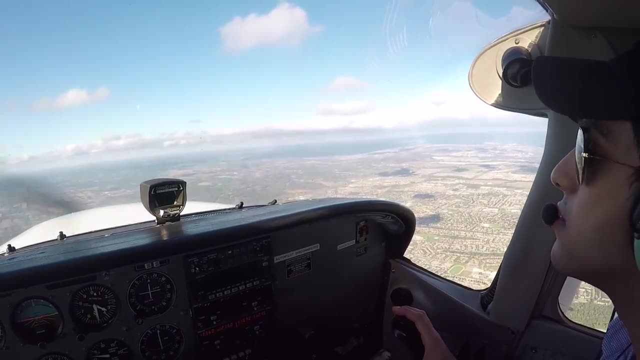 and they all said empty And I was like, oh my God, we're going to drop from the sky. So I got into best range. Luckily I had double checked the fuel before we took off, so we had enough fuel left. 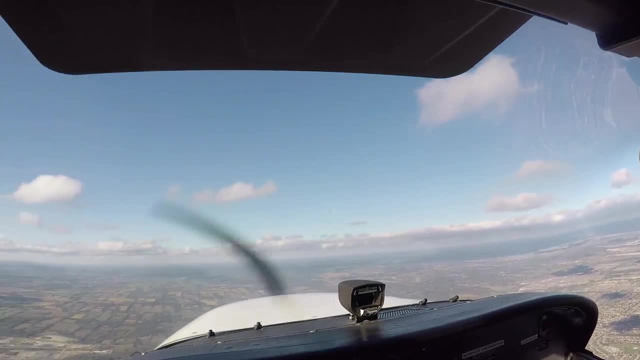 We had quarter tanks in each one, which is about an hour. Oh Lesson that the gauges aren't reliable, Anyways. So yeah, you might actually use it. So here I'll give you control. Hopefully I've trimmed this out. 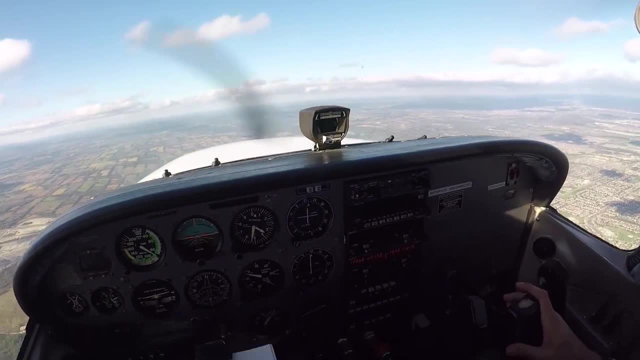 Why don't you do the exact same thing with the writing this time? Do you want me to do writing also? Yeah, So just for the first Here, I'll write it down for you, so it's easier. What RPM do you want to start at? 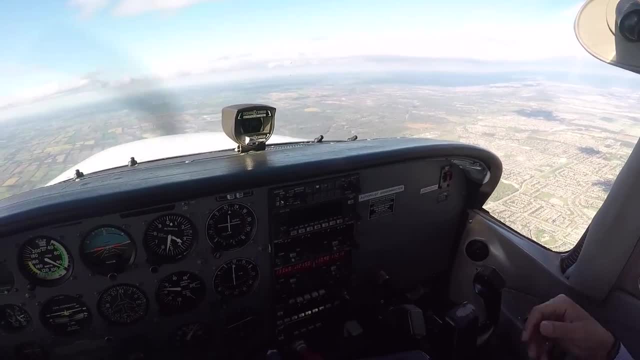 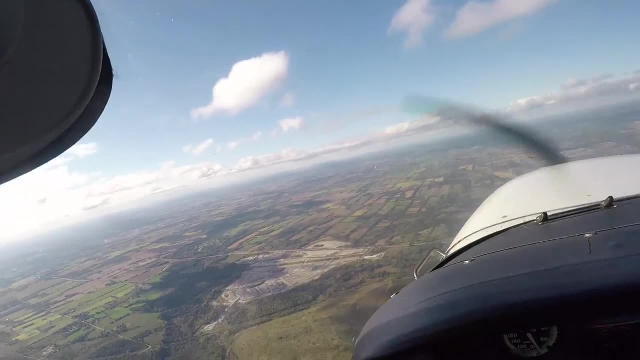 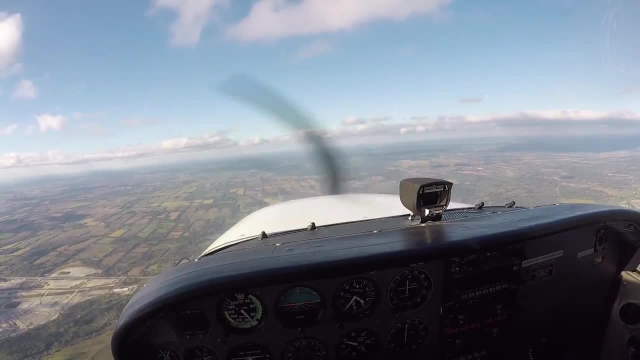 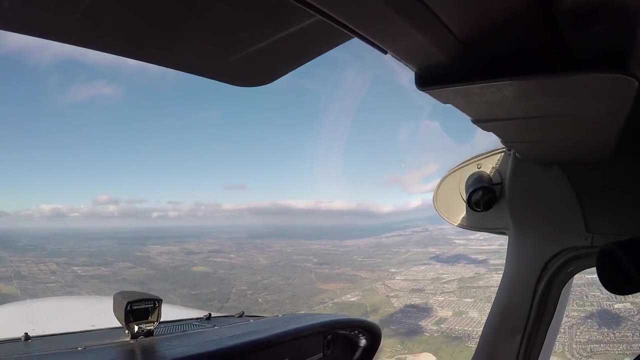 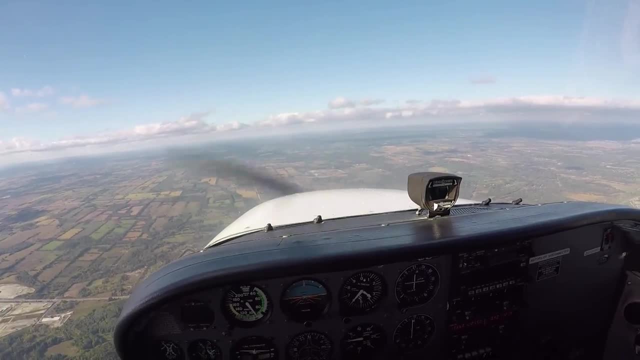 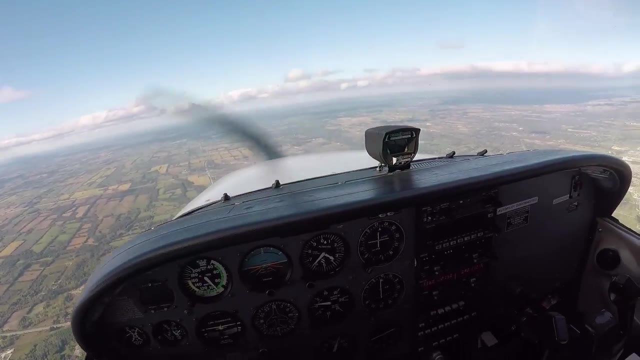 perfecting the actual procedure to find out best range and endurance. Okay, Tell me when you're ready. Oh man, Okay, 2,000.. 2,000.. Let's stabilize altitude and airspeed. All right, All right. 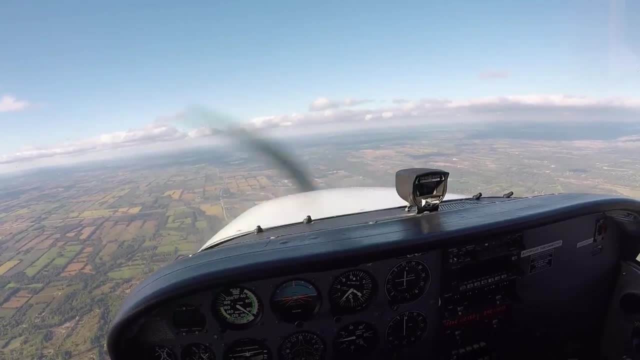 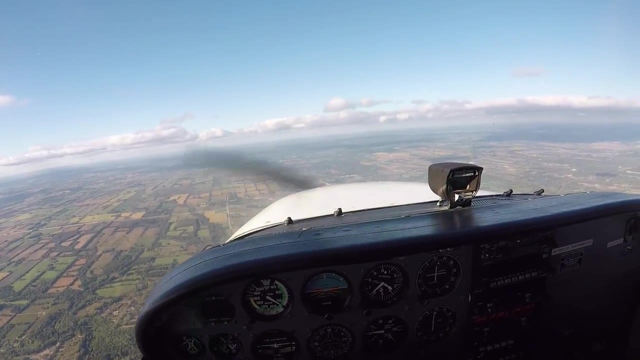 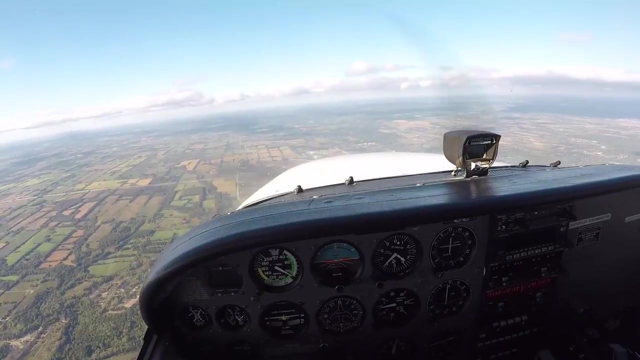 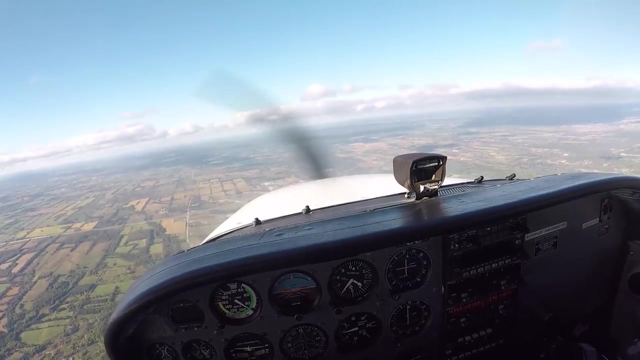 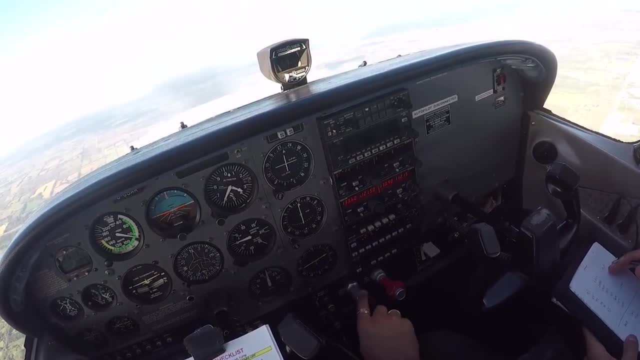 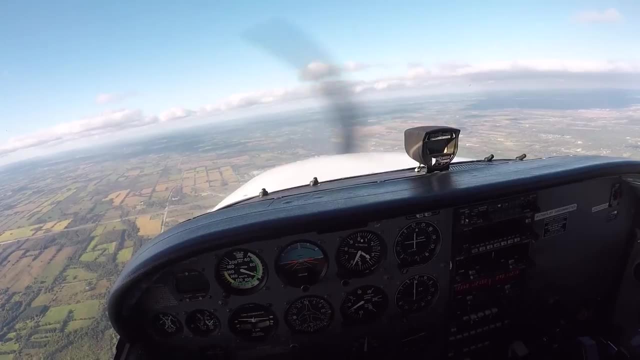 1,900 or 1,800? 1,900.. Okay, That's 1,900.. Nineteen hundred and ninety-two. I'm losing it. Okay, so stop that loss, Though that's now eighteen hundred, right. 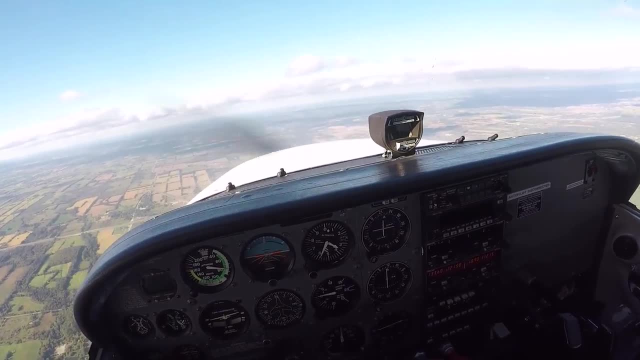 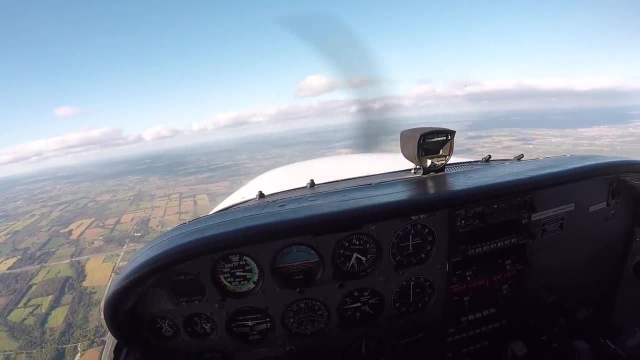 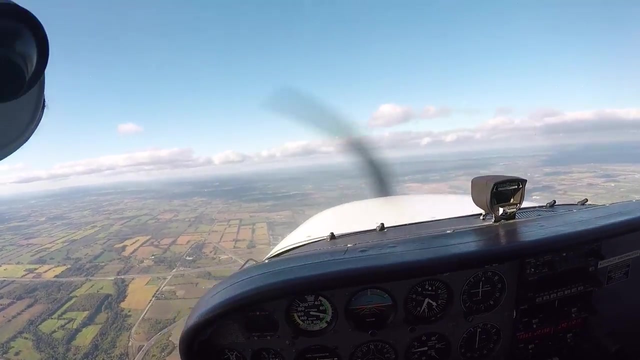 So get back to nineteen, Oh, other way, Okay. eighteen hundred eighty-five, It's okay, we can start from there. Or seventy-five rather, because that's the drop we're expecting. Um, why don't you go down to seventeen-hundred? 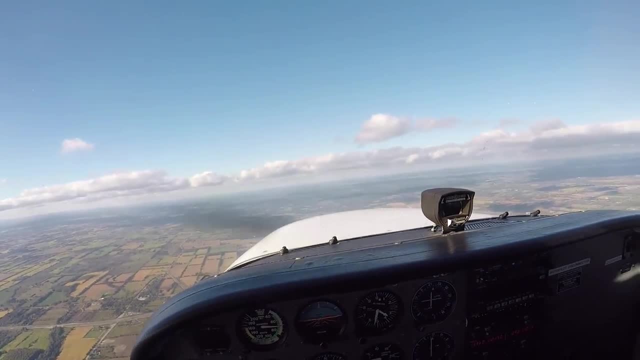 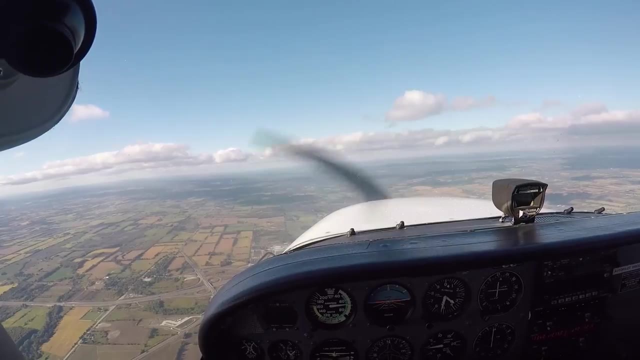 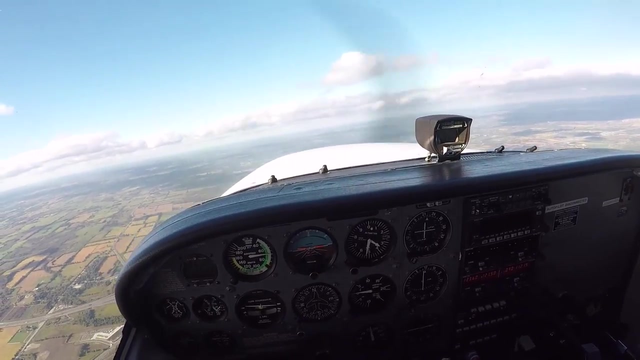 Okay, What's your altitude? I mean, what's your airspeed? Airspeed is seventy. Yeah, looks like it's around seventy to me. Okay, Alright, so back to hundred. That's between How much? 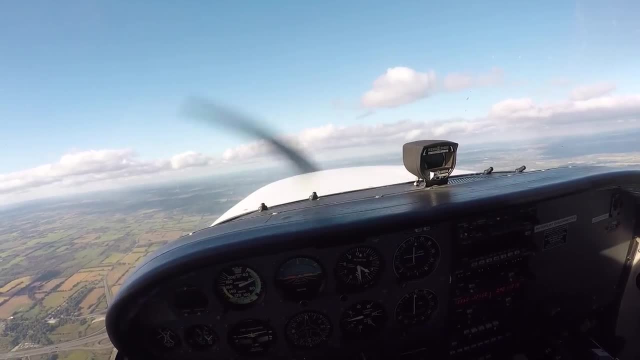 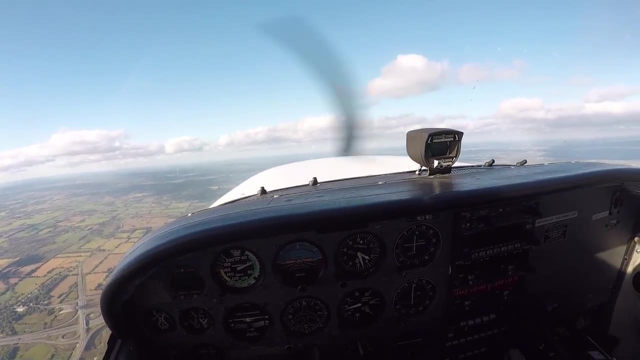 Okay, sixteen-hundred, That's your below sixteen-hundred. Get it back a little bit. There you go. So we are at sixty, so that's ten knots drop. Okay, so sixty. So best range then should be seventeen-hundred. 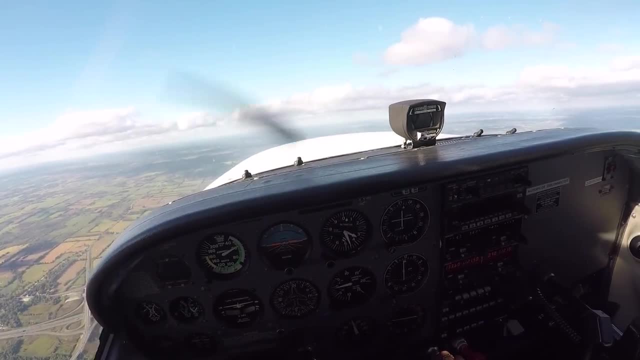 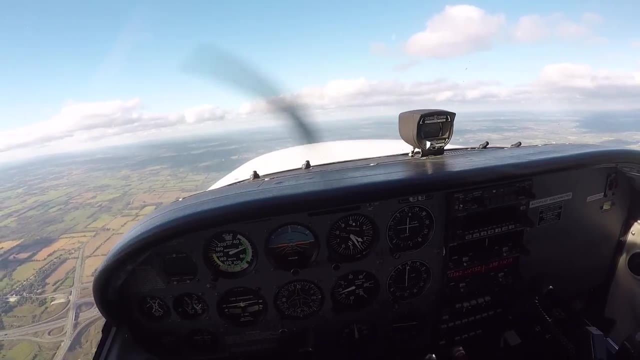 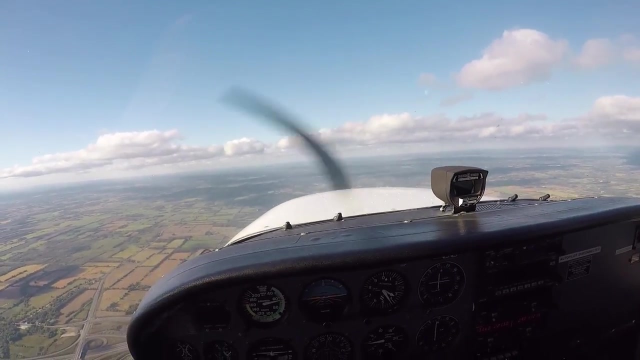 So let's get back to seventeen-hundred, Perfect, and that should give you approximately an airspeed of sixty-five to seventy, and we should not be losing any altitude And we'll just hold it there. So let me know when you're at best range. 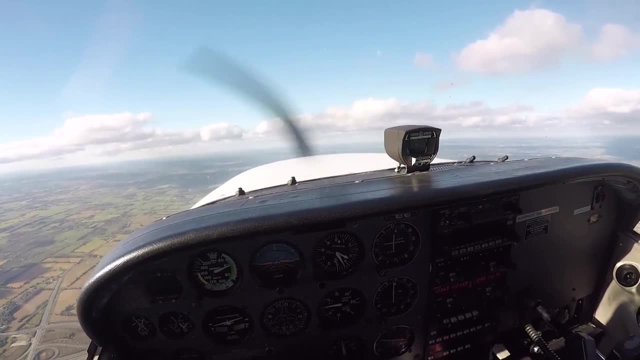 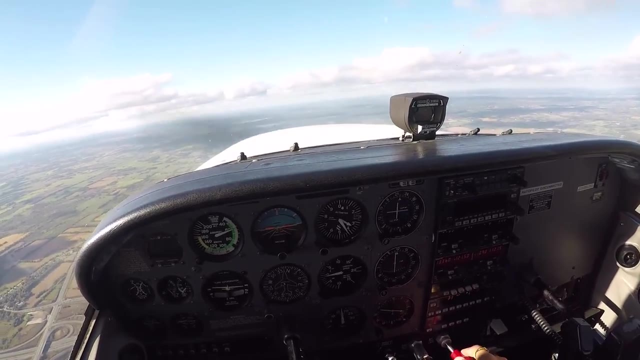 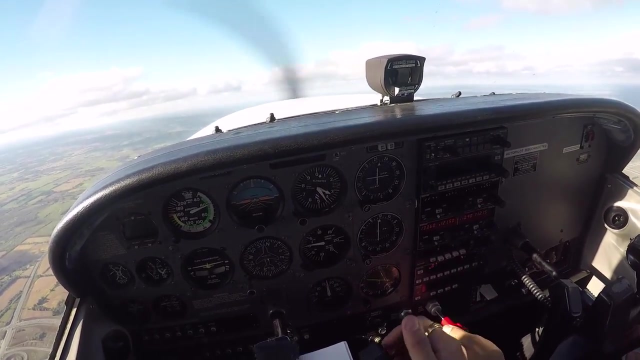 There you go. I can't see the drop at all. Keep going until you see the drop. Did you see a drop? I didn't see a drop, A minor one, but notum, but not a major one. There's your drop, right. 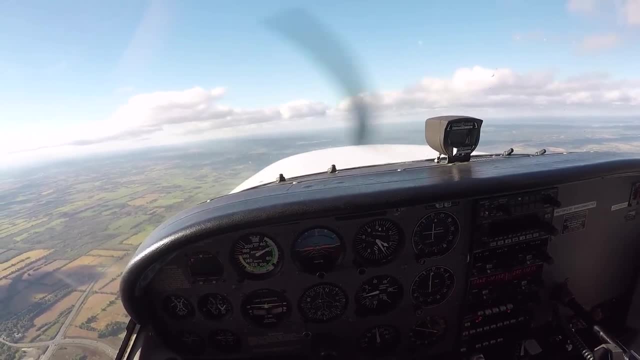 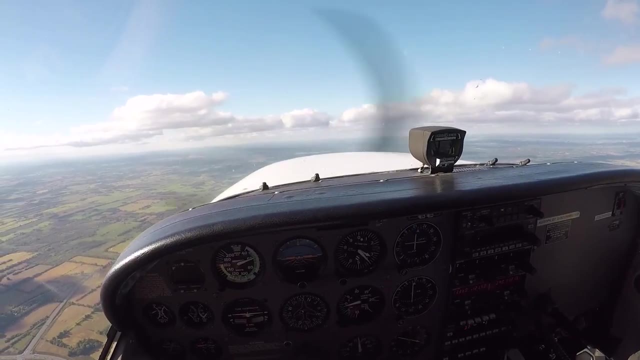 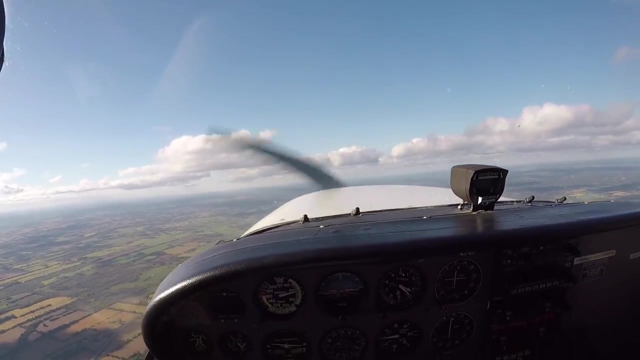 Yeah, One, two, three. The storm warnings trips me off. Sorry, it's not a big deal. Sometimes, when we are at zero VSI, we are losing altitude. That's because this is a very laggy instrument. Ah, okay. 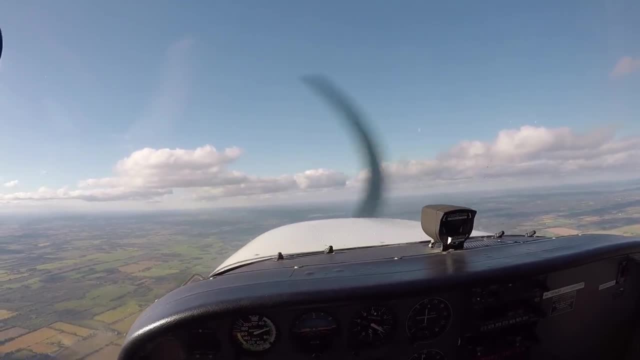 I see, Yeah, you'll learn more about that in ground. We can talk about it on the ground once we're there, but it's a very laggy instrument. But perfect. Well, that's best range. Why don't you recover for me? 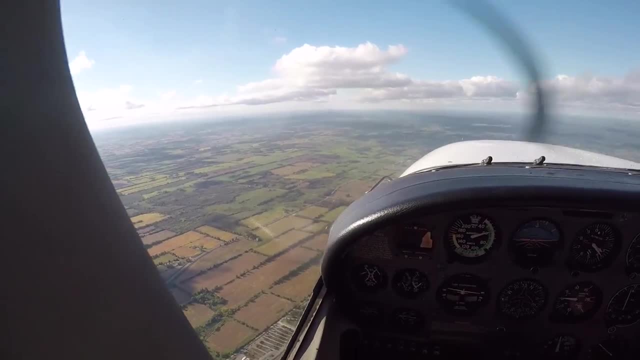 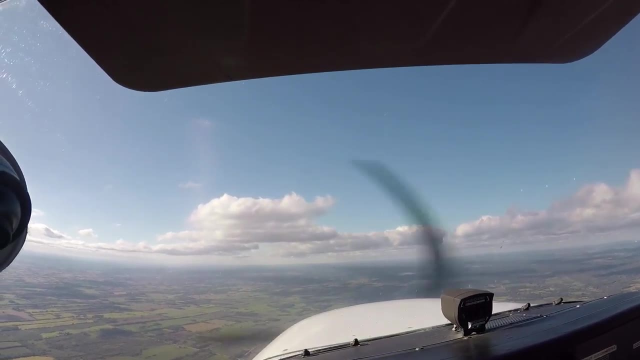 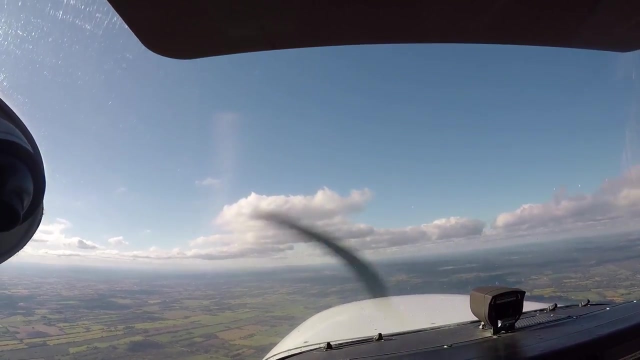 Okay, Look around. Complete Check Gauge is green. Check Two: All right, Make sure it's on. So notice the attitude and the airspeed and the performance of the airplane. What the hell is that? Are those birds? 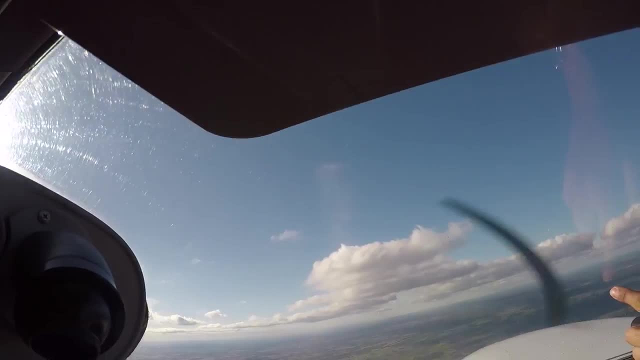 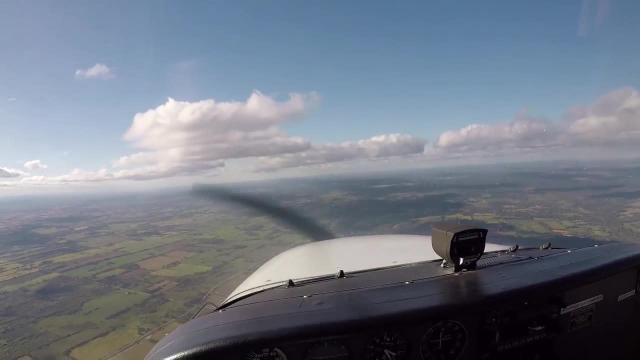 Where? Oh yeah, I thought that was like a dirty cloud. Anyways, notice the attitude and the airspeed and the overall performance of the airplane. when you're in best range It's very slow, very nose up right, It's counterintuitive. 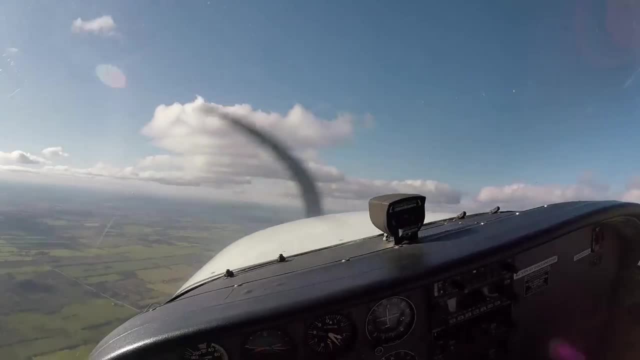 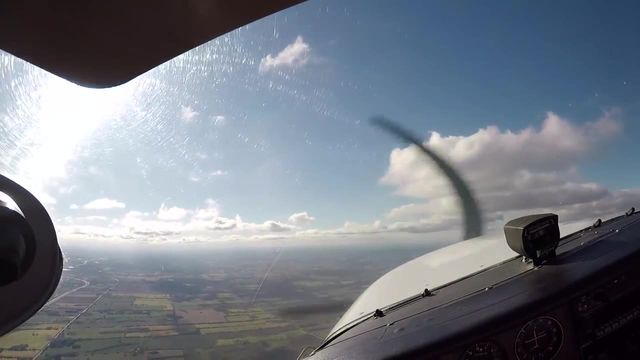 to think that if you want to get somewhere or to maximize your distance, you go slower than you usually do in cruise. So why is that, do you think? while we're recovering, Why do you think we have to go slower to maximize our distance? 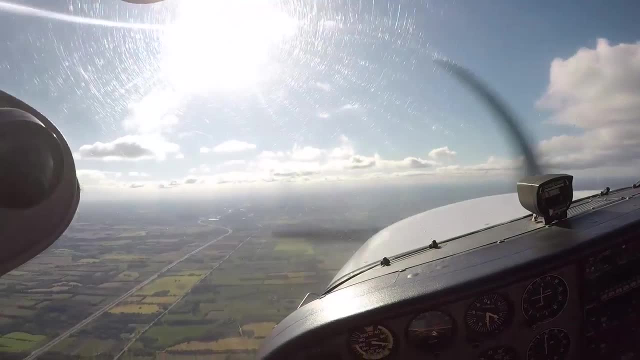 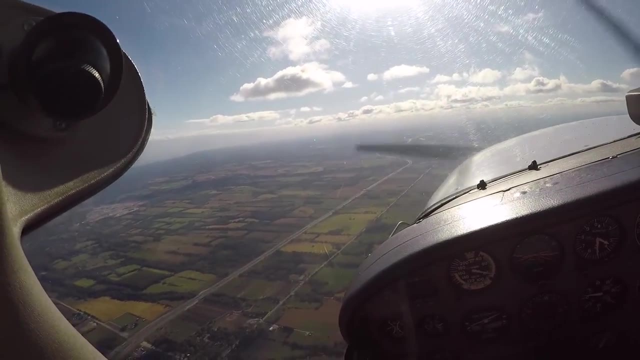 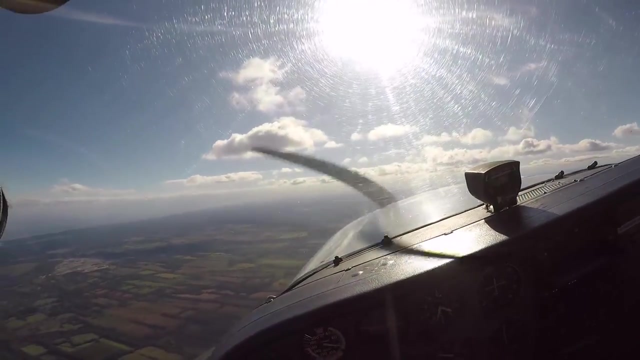 Because we're using less fuel? Yes. but if say, say we went full power, Okay, What stops us from, you know, going the same distance at 1600 RPM? What about full power? Full power And the airspeed? 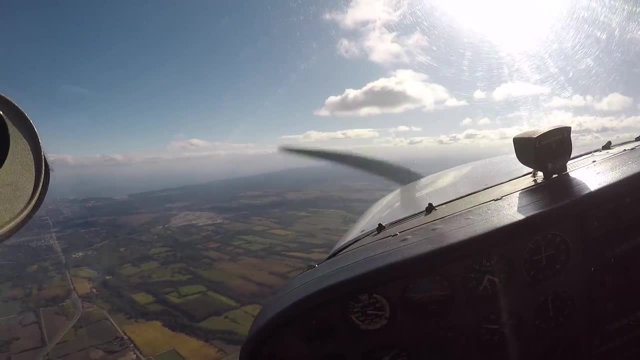 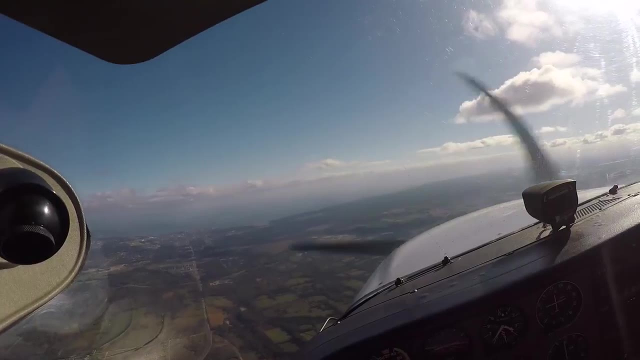 that should be your hint. the airspeed we're at when we're at full power, Okay, stops us from maximizing our range For the consumption of more fuel. More fuel for what? Yeah, Like more fuel Per amount of drag felt by the airplane, right. 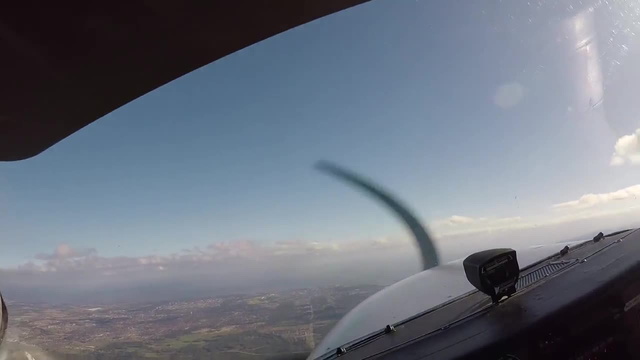 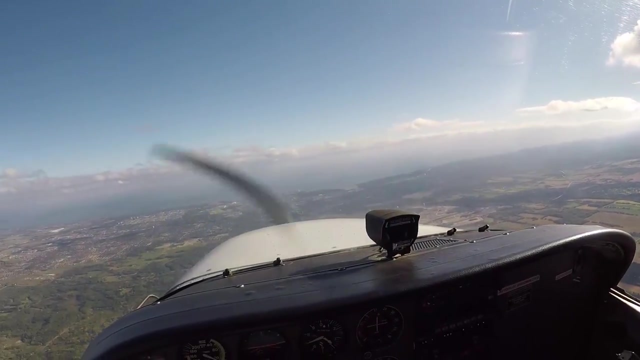 Remember that chart we had of the airspeed versus the drag? Okay, And then the faster you go, total drag, right, Yep, The faster you go, the more drag you experience, And you don't need to waste time talking about that right now. 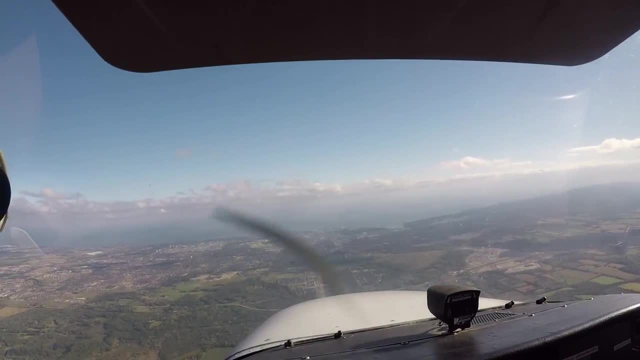 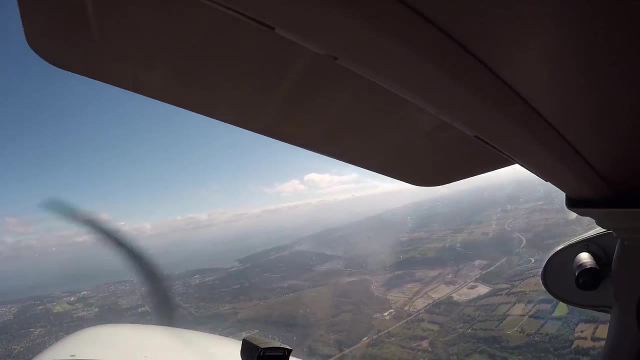 because that's all theory. but basically, all I want to say is notice that, to maximize your range, we have a lower airspeed and a nose up attitude Here. let's turn north. Holy, You're going to save some time, Okay. 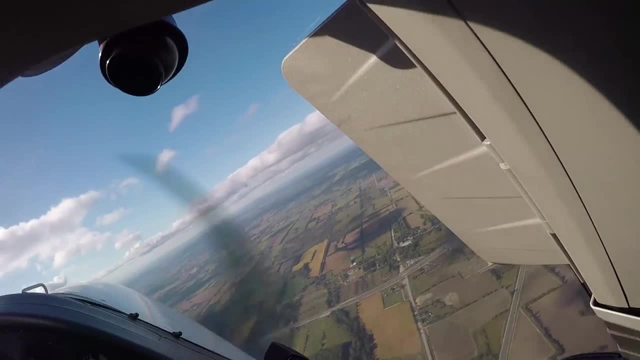 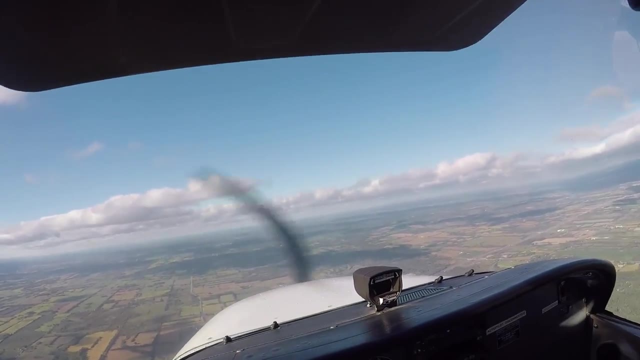 Did you just sink all the cheese for full day? No, not really, Man. I had to sleep like an hour after going. After that, It's definitely tiring. I drink a lot of coffee. Oh, Holding that there, holding that there. 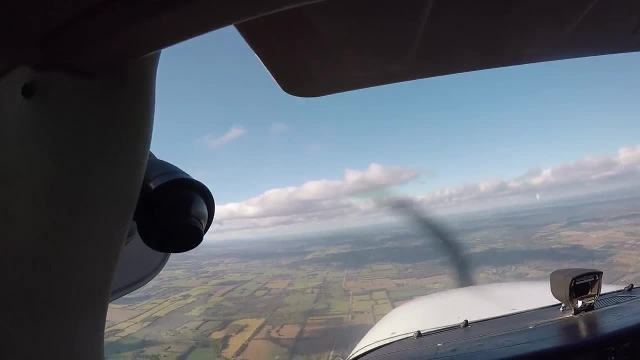 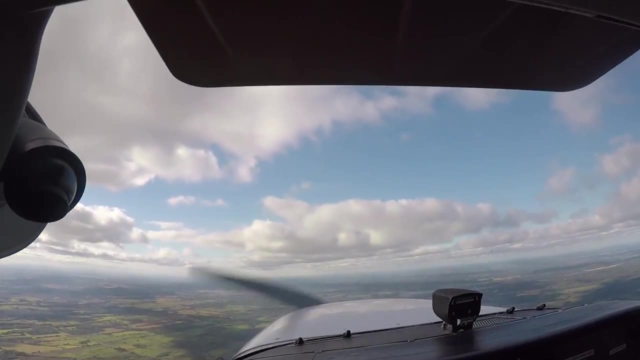 Look, You're blowing up. You're blowing up, I'm blowing up. Yeah, I'm blowing up. All right, see you in a couple of days. Uh-huh, See you in a couple of days. We're going to. 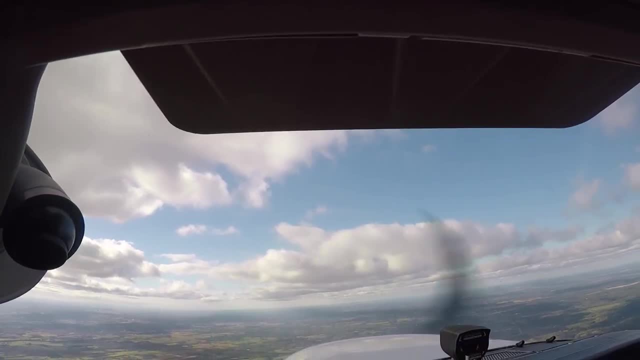 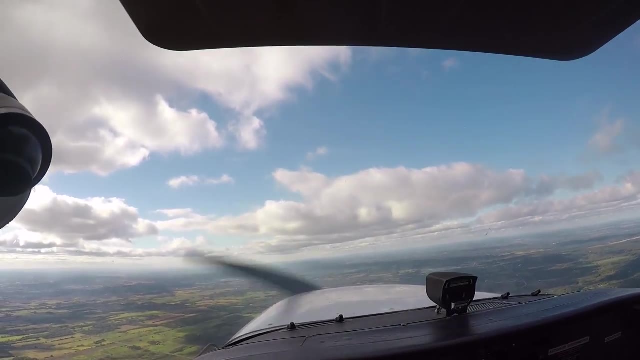 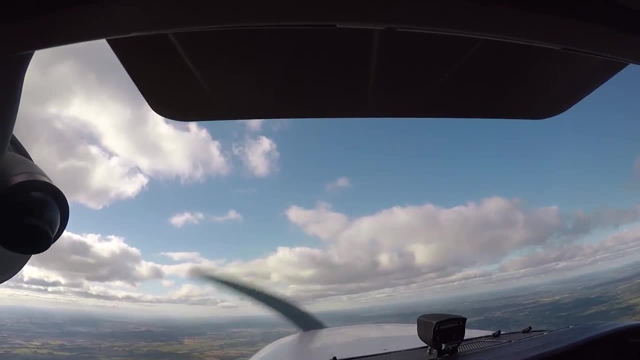 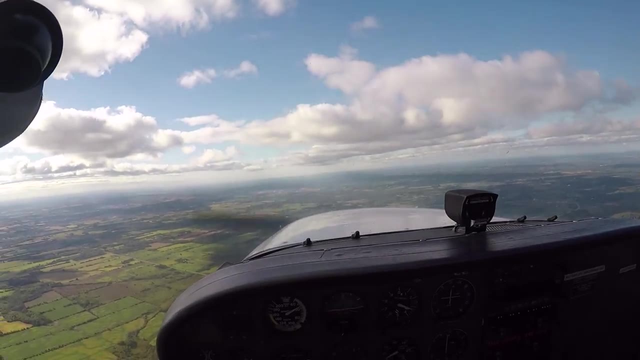 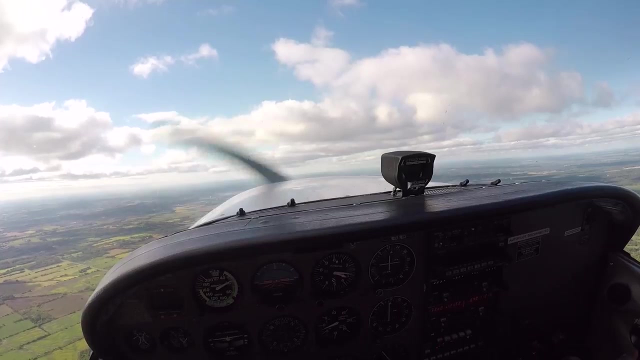 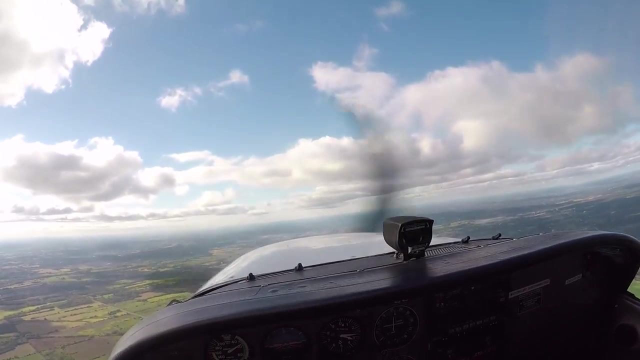 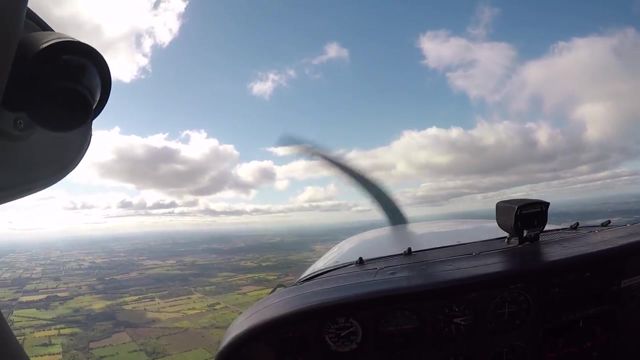 power, let it stabilize. hey, so after it stabilized, notice now we can't maintain any altitude at all. yeah, so we know if your best range was six, seventeen hundred. you said getting back to the last power setting where you could maintain altitude and holding that. whoops, there you go. look, your altitude stabilized 55 knots, not losing altitude. 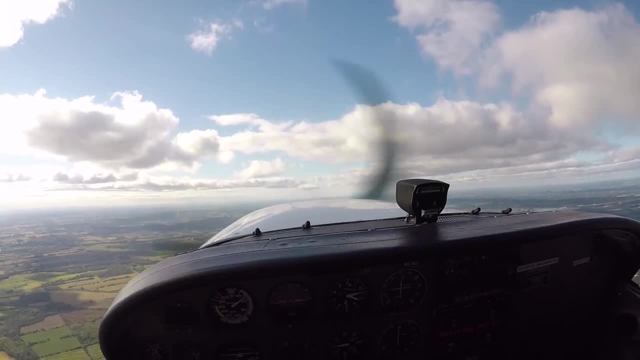 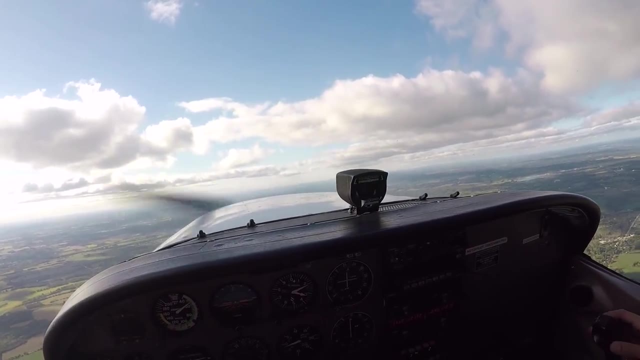 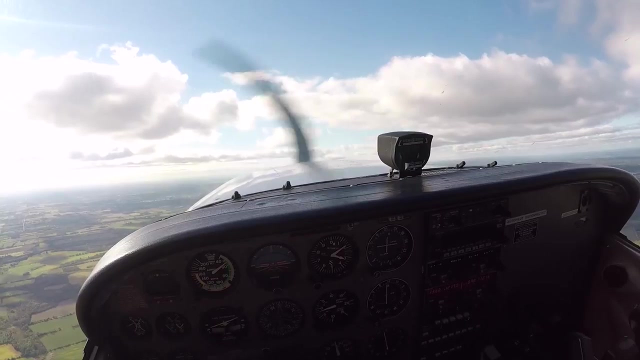 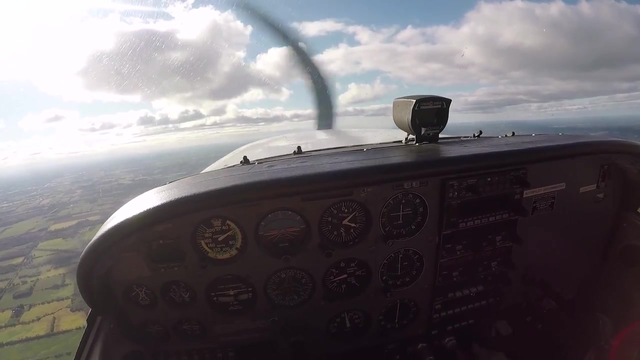 lower power setting than range, lower airspeed than range. this is your best endurance, or is it? or is it now? we are losing altitude? now hold it. this is your best endurance and the right. why is the heater on? remember you want to maintain that attitude that gave you the best. 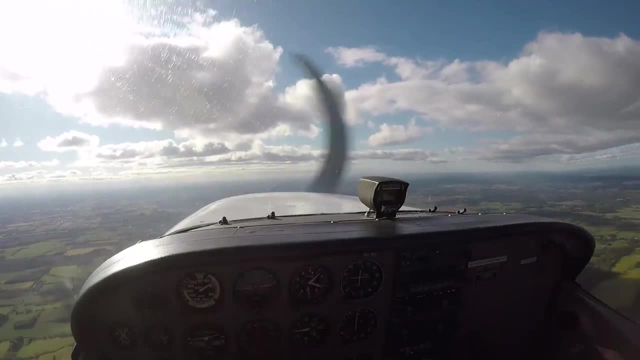 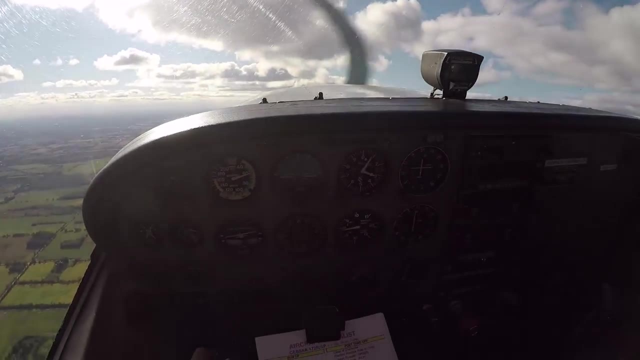 endurance right, because the minute you pull up and slow down the airspeed you scrub the whole calculation. yep, it's annoying too, because we don't have a constant, constant speed prob. so the minute you pull up here, rpm also drops. I don't how much that contributes to it, but I could be pulling a lot of stuff out. 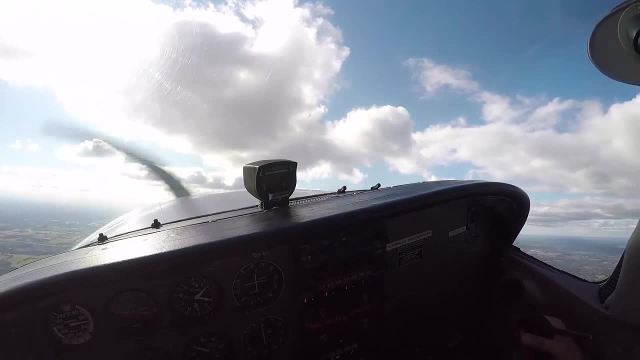 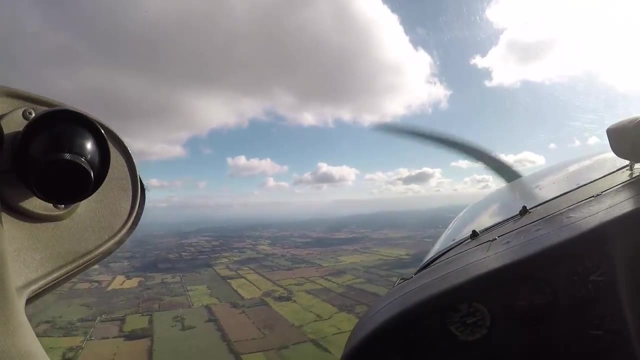 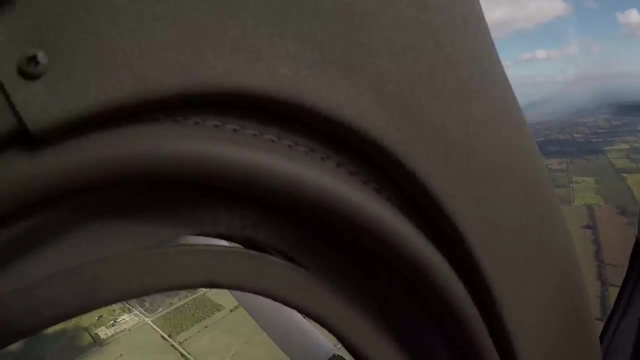 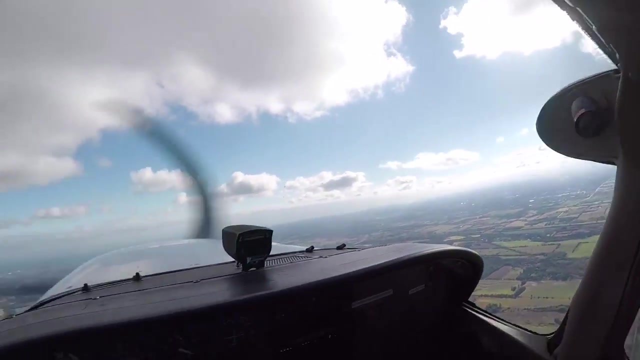 of my, but anyway, does it make sense? yeah, so what i'll have you do now is will climb back up to altitude. I got a peak at you. yeah, here we go And I'll have you do it again. Okay, find me best range, Find me best endurance. You have control, I do. 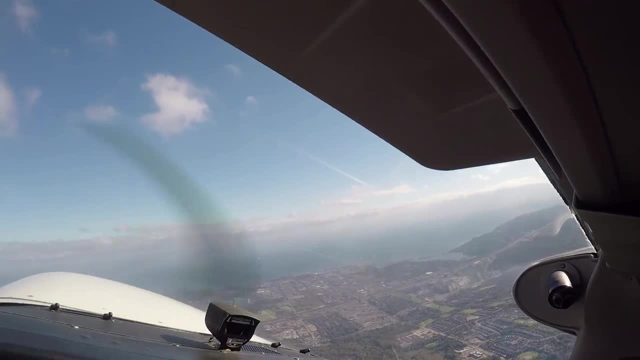 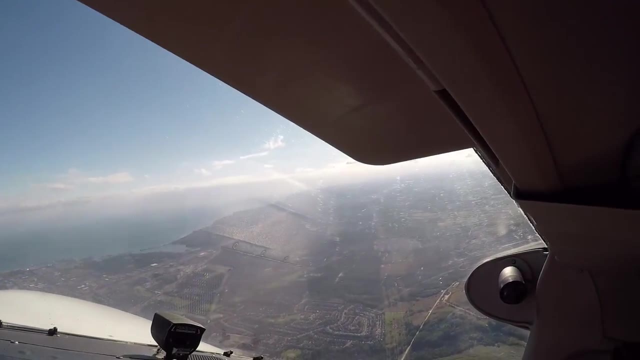 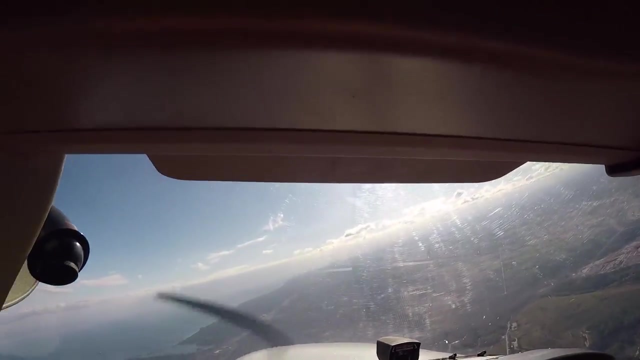 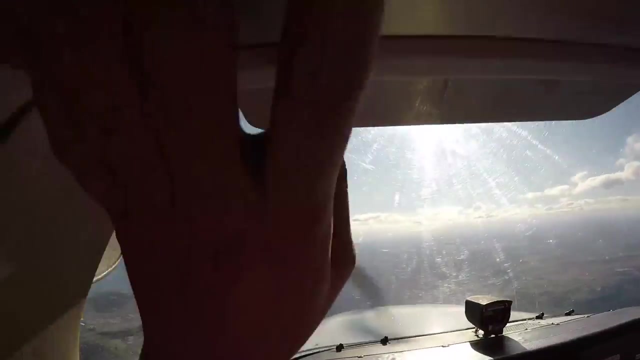 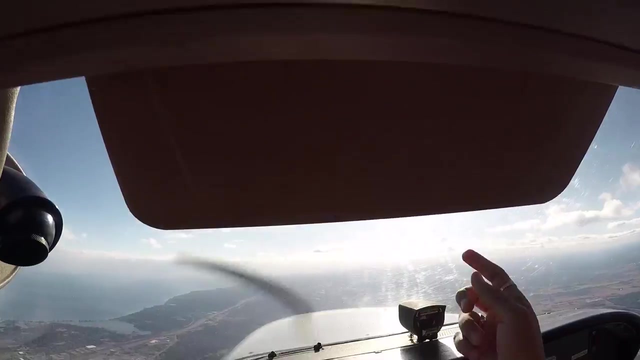 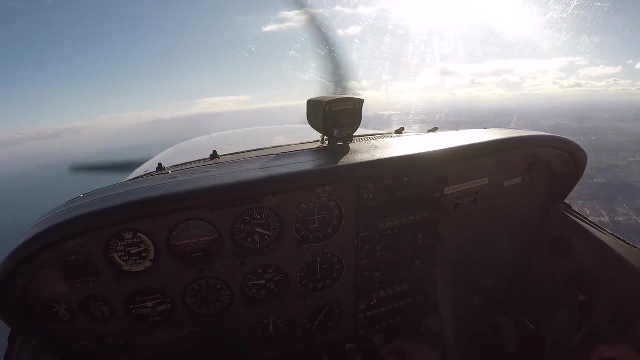 Let's just turn away from that side, because we might be getting into Oshawa's airspace. Hey, attitude, power trim, Ow. I wish I had the GoPro. Oh, the sound effects. This thing's probably blocking your image. Perfect. So are we in best range? Not yet. 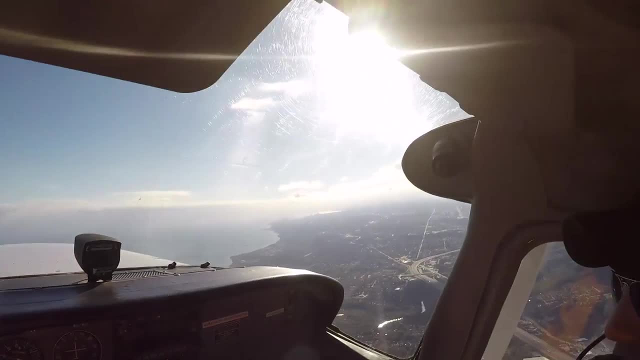 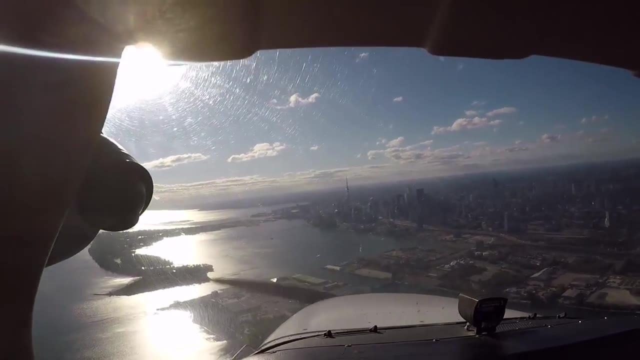 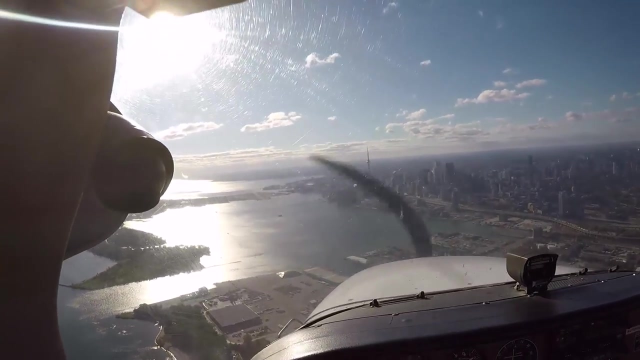 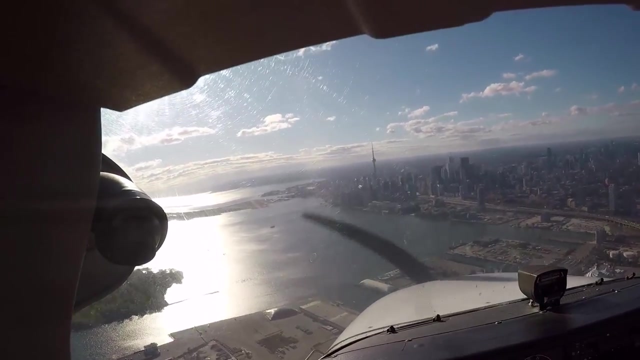 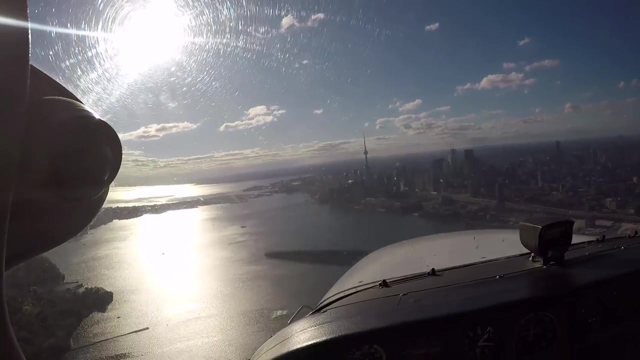 Hey, it looks like beautiful, beautiful, no complaints. let's recover. So elevations, What does it? 300, or elevations 300? Let's start slowing down, Power back to 1500 And pull back to slow us down. I don't, That is straight. 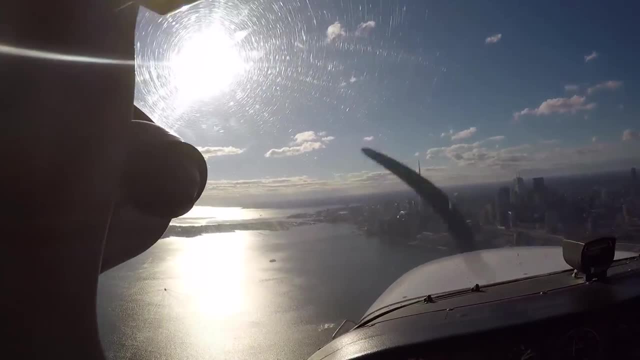 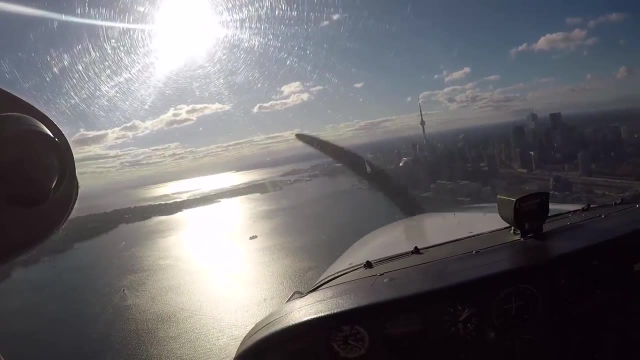 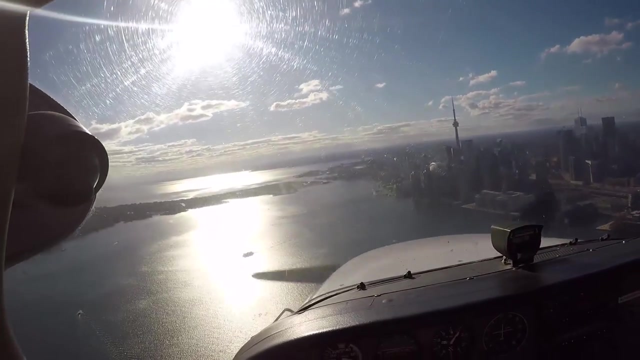 It's a little 10 and 10 left, right, Yep, And It's a bit bumpy today. Usually the rule of thumb is: add half the gust factor to your approach, So we usually approach it 7-8. It's gusting 10 knots over the wind speed, So we'll fly at 75. 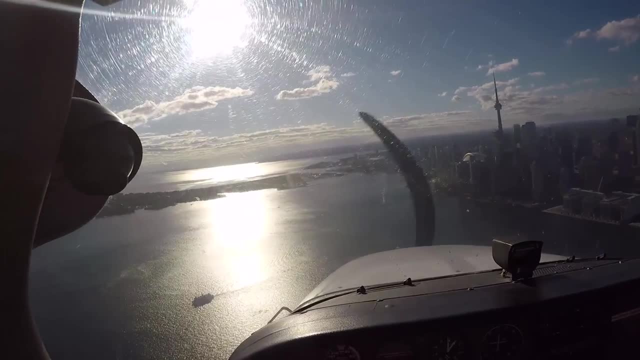 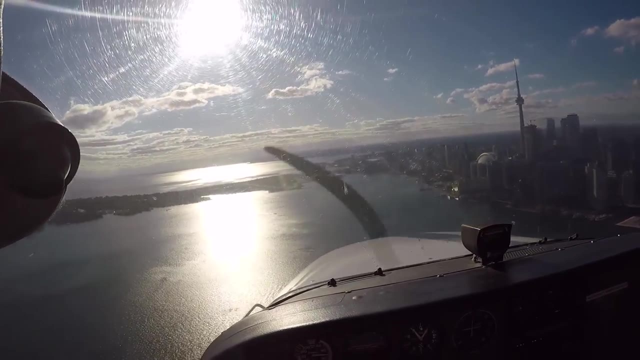 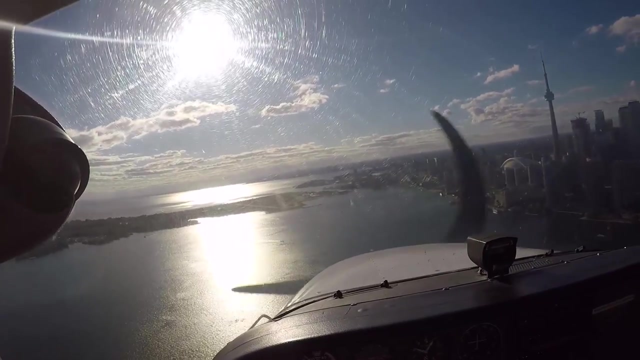 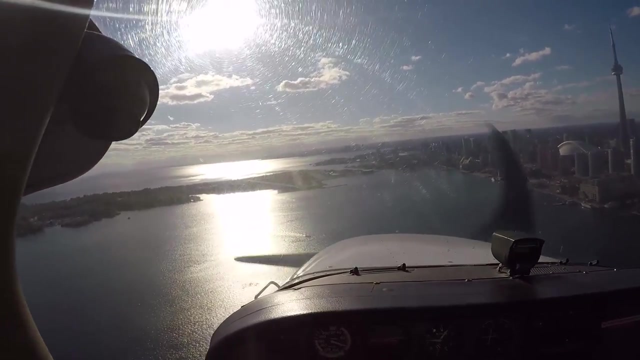 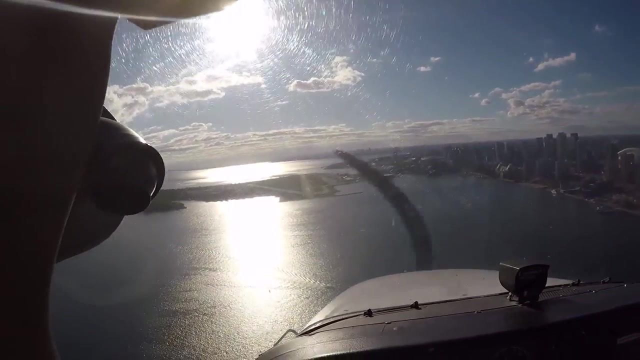 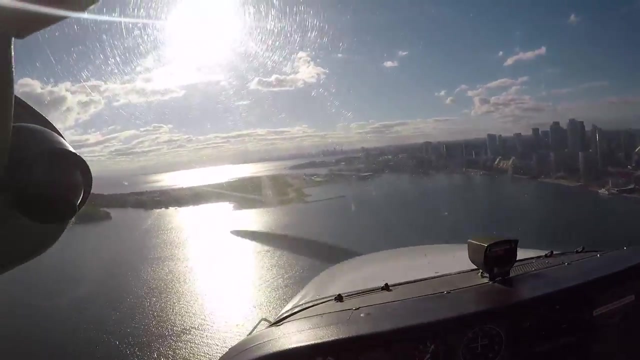 I'm gonna drop down a little bit more. No, Sanchez, little bit more. Yeah, it's what is it? 330? high are we low, We are high. So pull back the power a little bit. Power idle, power idle. We're quite high. Can we do the flaps full? Probably not in this wind, Oh, okay.